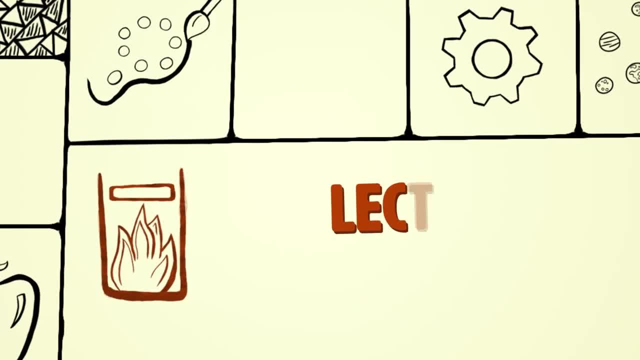 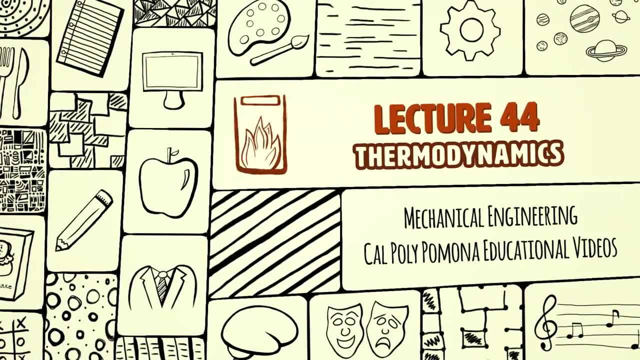 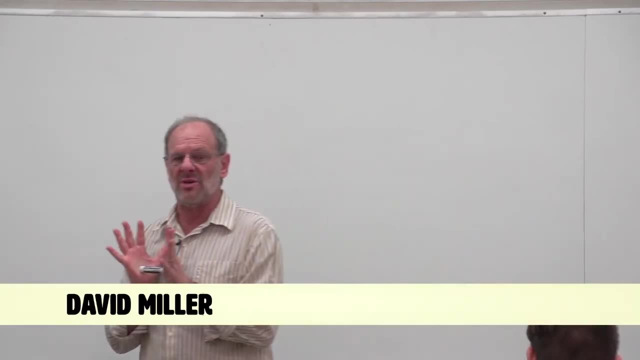 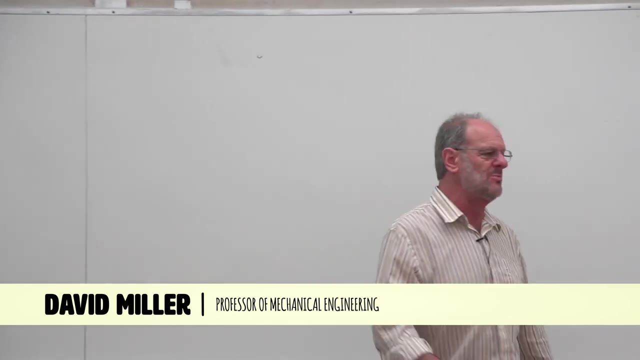 Okay, Well, good morning everybody. So please don't forget to pick up your homework. that's up here at the front. These are all problems that dealt with well if they were dealing with property relations. you know there are a few bounding analysis problems in there. 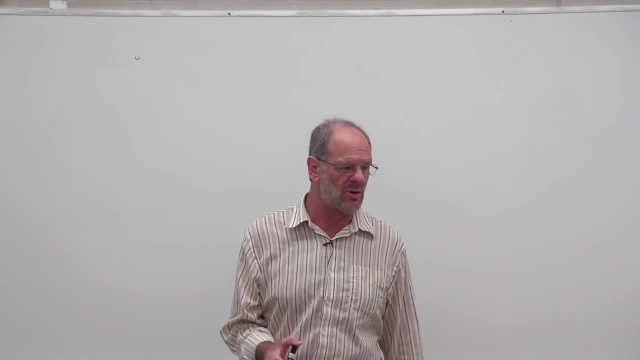 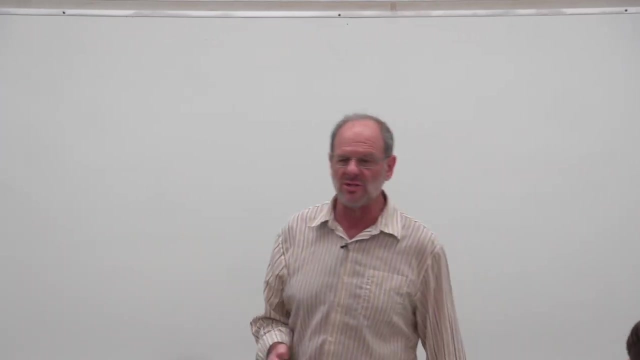 and you know just one where you were actually a couple. One was very short, which asked you to just go through a little bit of a derivation, But pretty much everybody did fine. I mean, the problems are pretty straightforward. Most everybody got the right answers There were. 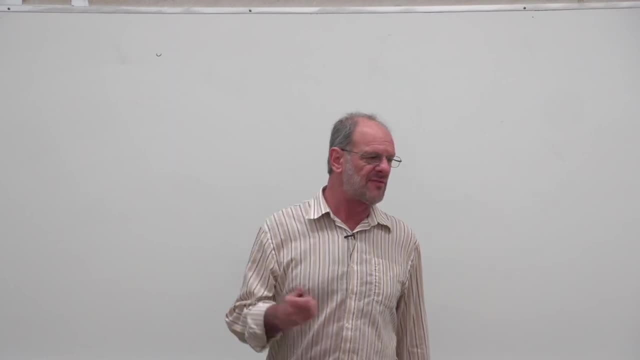 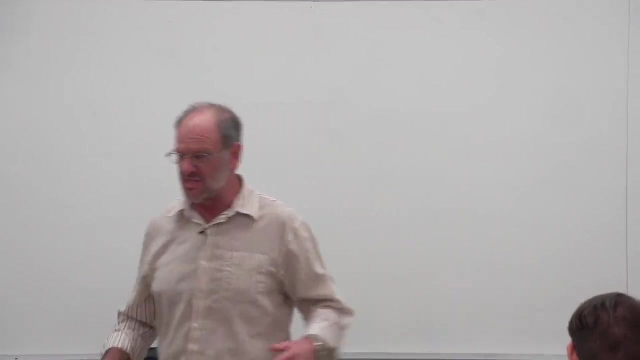 some unit issues. Some students weren't particularly careful in the British units at providing conversion factors so that you could equate, let's say, the left-hand side and the right-hand side of an equation. You know, like if you're trying to say, validate one of the Maxwell relations or something. 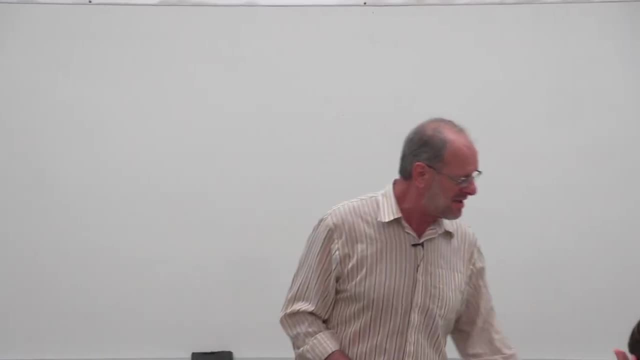 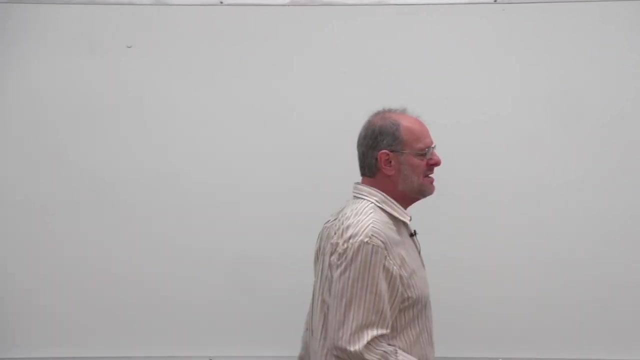 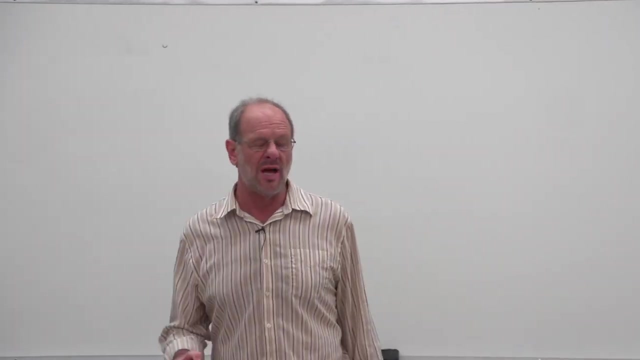 like that, But nonetheless most students did just fine. So no real comments on the homework. that's been returned to you. Again, the usual reminder: your second midterm is coming up in a week. a week from today. There's not going to be any closed book section. Well, 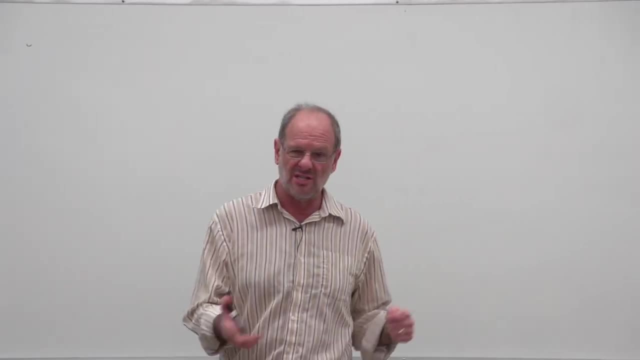 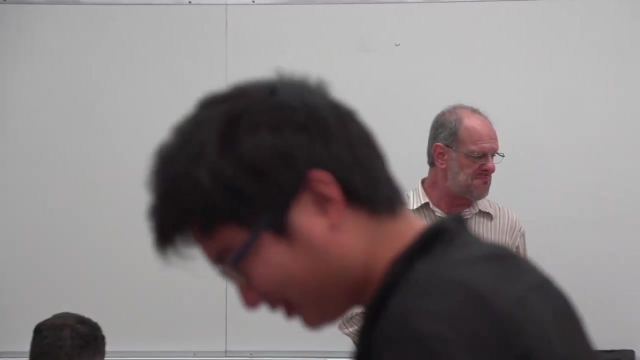 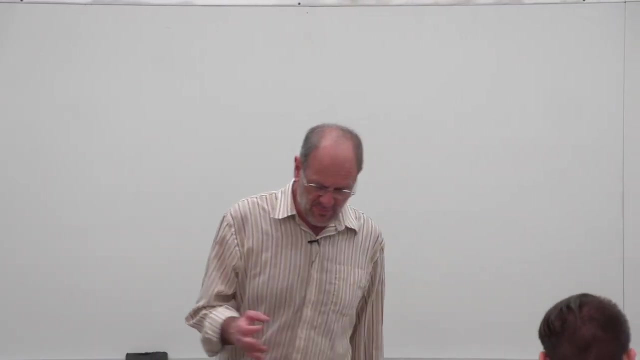 I'm sorry There's not going to be any closed book, closed notes, closed everything sections, Just one section like the previous exam. So closed book. but you can bring a three by five note card with equations and diagrams. These are midterms only. Let me also let you know that. well, you could fill up your 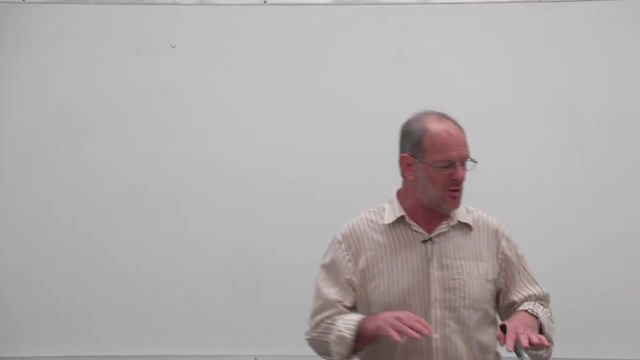 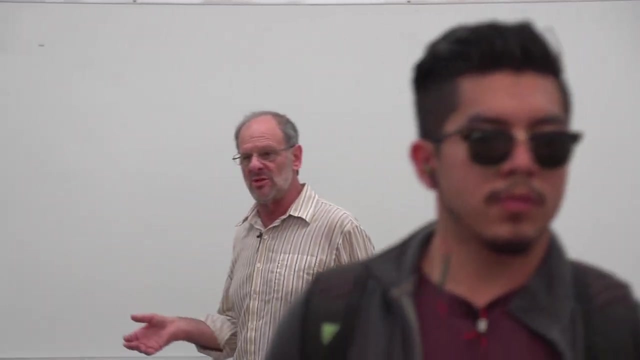 entire card with these various thermodynamic property relations, right, And I don't want you to do that. So let me just tell you all right away that any of the thermodynamic property relations that you would need on the midterm exam will be provided for you, at least the. 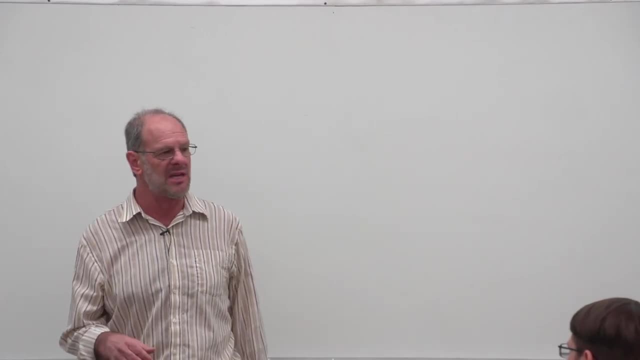 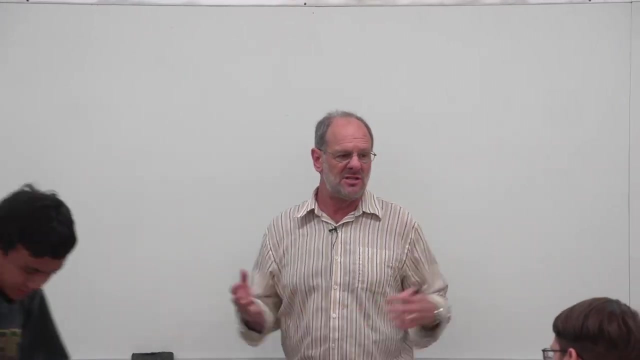 general form of them. You know the partial differential equation or whatever it happens to be. Yeah, to clutter up your diagram, I'm sorry, your note card, with this kind of information. You know all again, all the thermodynamic property relations. you. 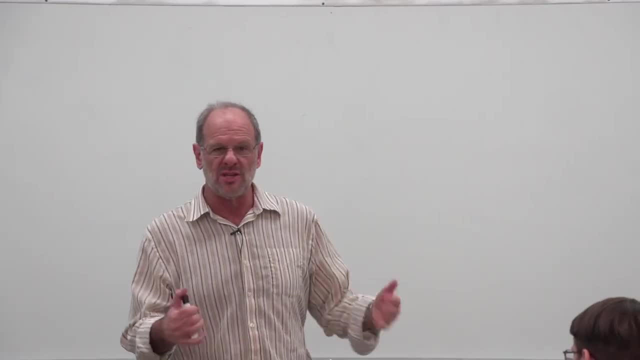 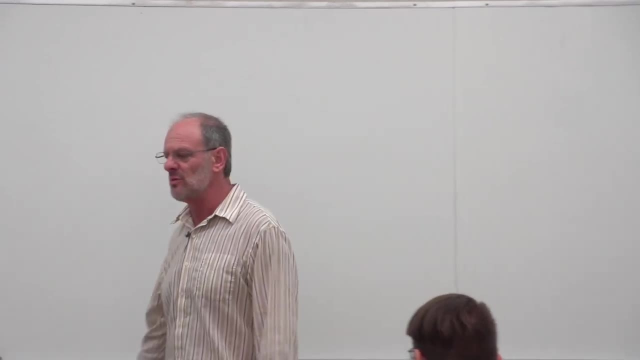 need will be provided on the exam. Anyway, of course you want whatever other information that you need to be on your cards, but just not that. So you know, next week we'll talk more about the midterm. Next Wednesday I'll set aside time. 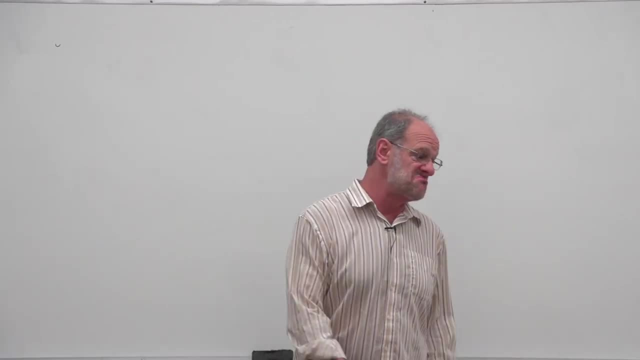 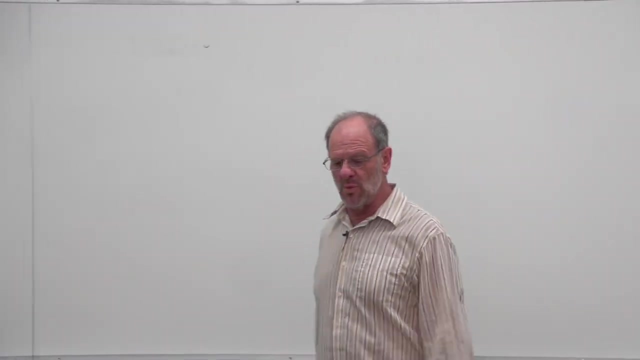 at the end of class, to you know, answer questions. just briefly go over what the midterm is going to be more about. So let's just get back to where we were last time now. We're now dealing with our next topic, which is mixtures And in. 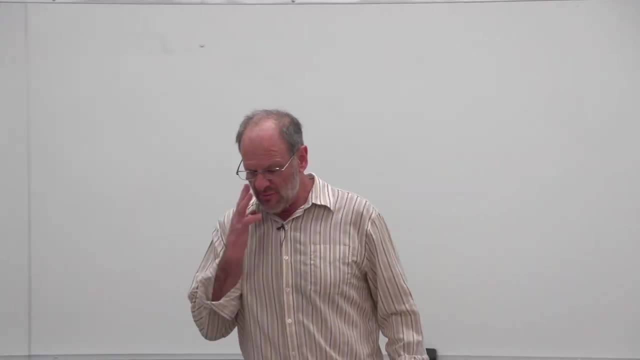 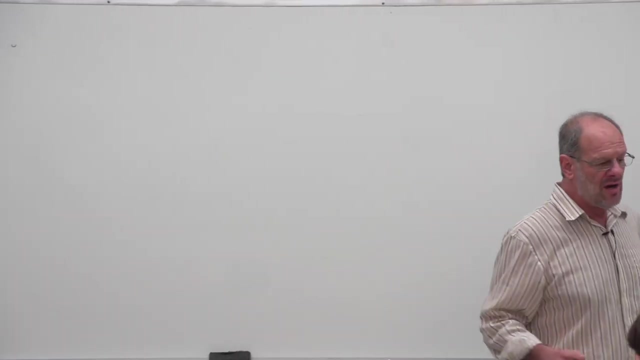 fact, specifically, we're done with general mixtures and we're now beginning to talk about, specifically, air-water vapor mixtures. Now, the air-water vapor mixtures that we're dealing with are atmospheric air, right The atmospheric air. 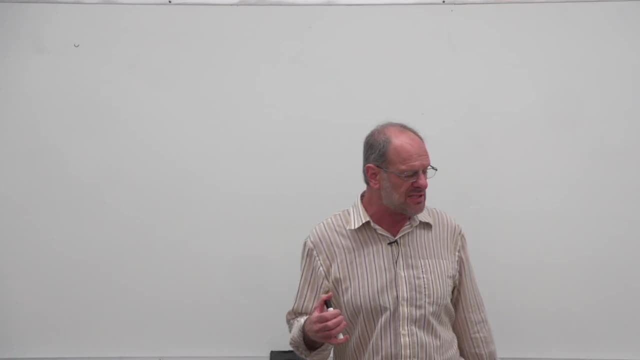 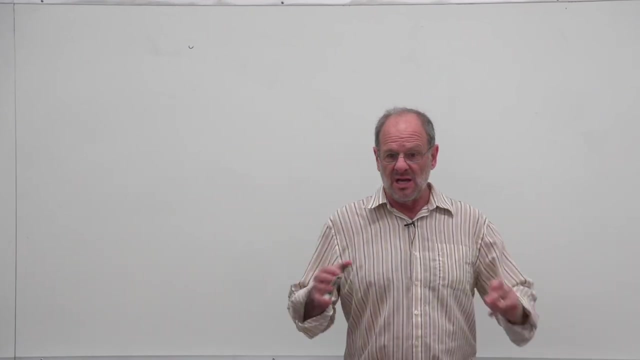 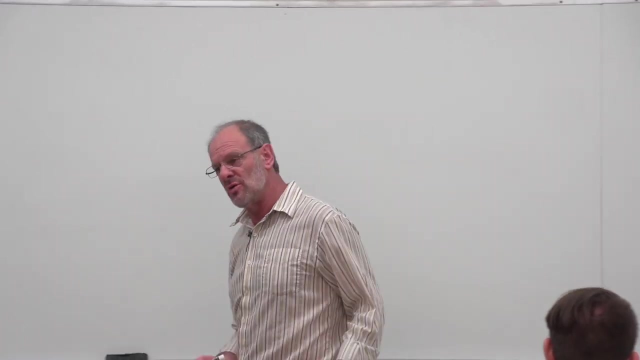 is a mixture of dry air and water vapor. Recall from last time that we're treating both the air-water vapor and the air-water vapor as a mixture of air and water vapor. So the air and the water vapor is ideal gases with constant, specific heats. Let's also keep in mind that you know we do have two components. 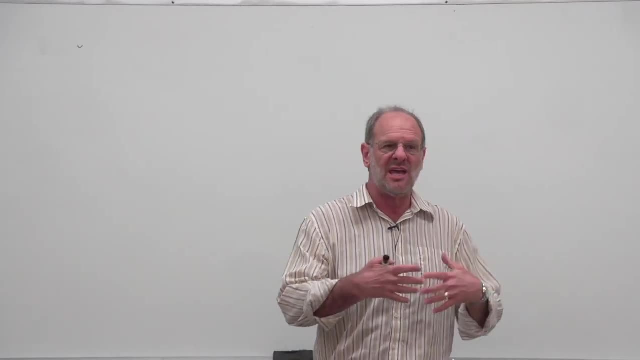 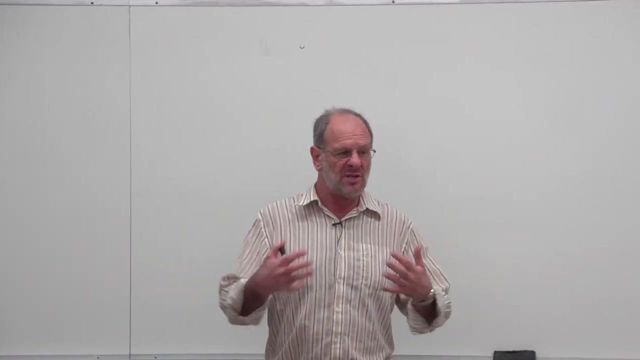 and the components in this air-water vapor mixture do not necessarily behave the way you might think they would, Since we have two different components, each component behaves as if it existed alone at the partial pressure of that particular component. So that's just something we want to keep in mind, that 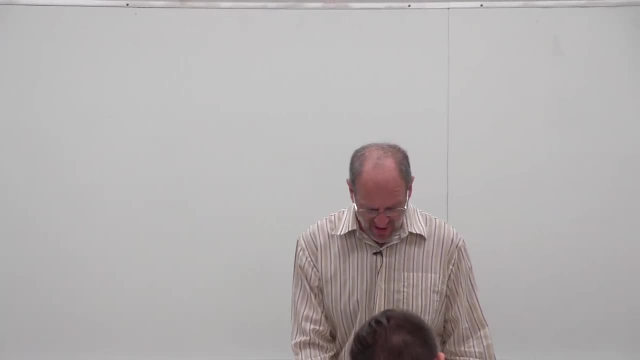 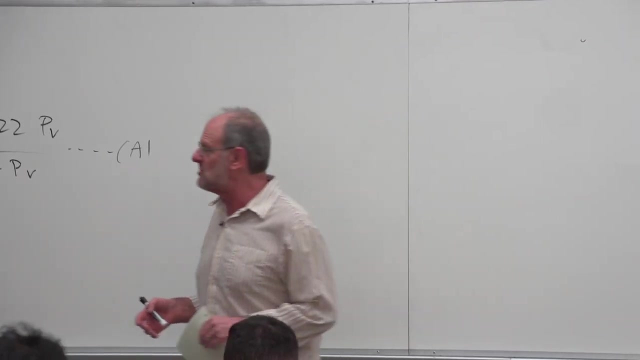 we certainly learned earlier last week or at the beginning of this week. So right now we're talking about again air-water vapor mixtures. There's various terms of interest to us. One of the terms of interest to us is omega, which can. 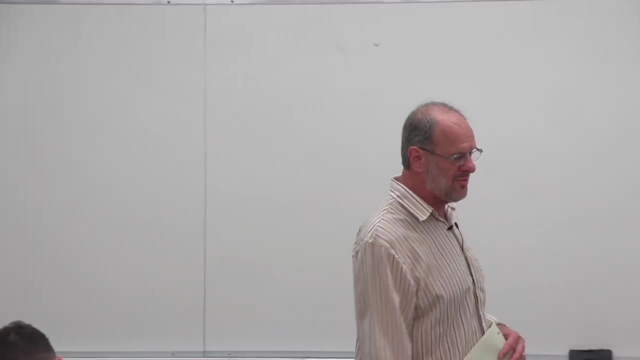 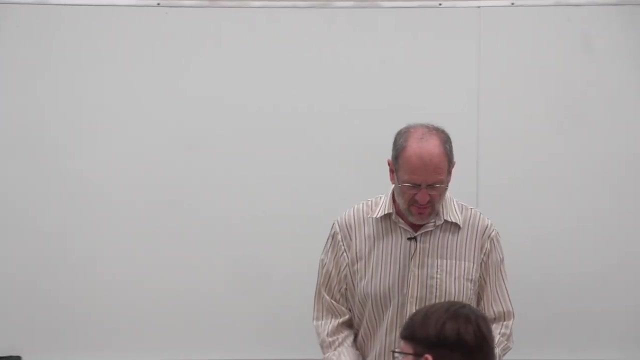 be called the specific humidity, or absolute humidity, or humidity ratio. This is just the ratio of the amount of water vapor to the amount of dry air. Let's also keep in mind that the dry air- even though we know dry air- is really a mixture of. 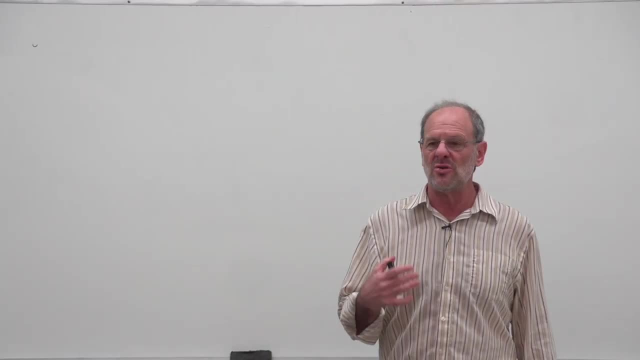 oxygen nitrogen and a variety of other gases. it's a mixture of oxygen nitrogen and a variety of other gases. We're treating it, too, as if it were a single component, and we're just using its average data. That is its apparent molar. 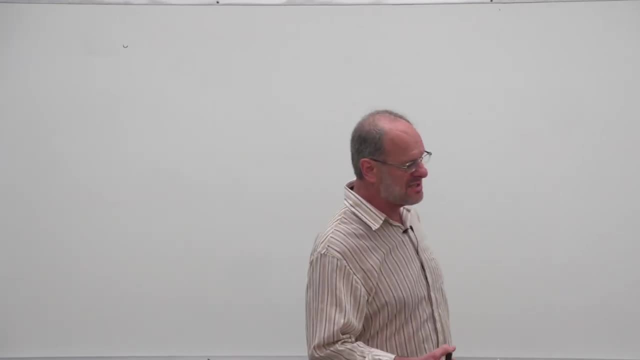 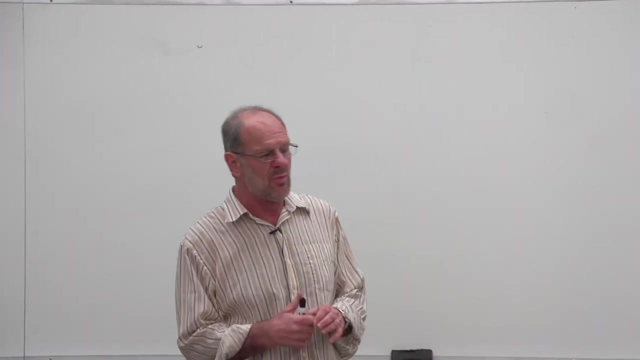 mass and gas constant, its apparent specific heats, et cetera, et cetera, et cetera. So all that data for air is presented in your textbook in the various tables, like table A1 and table A2. So please make sure you use that air data. 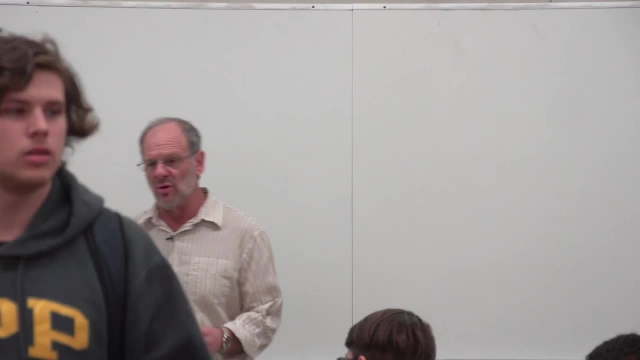 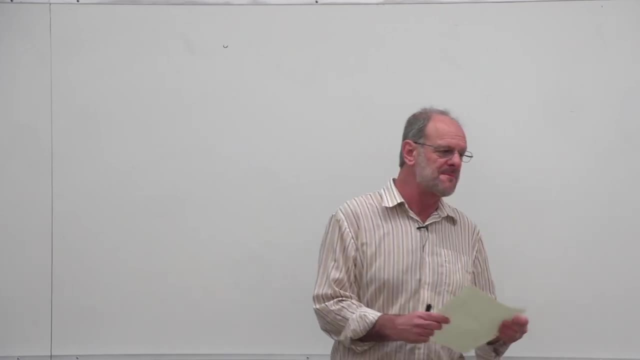 appropriately. Do not consider air to be a multi-component mixture Again, even though we know it is. we're just going to use its apparent molar mass and gas constant data for all of our problems that we're going to solve. So, nonetheless, 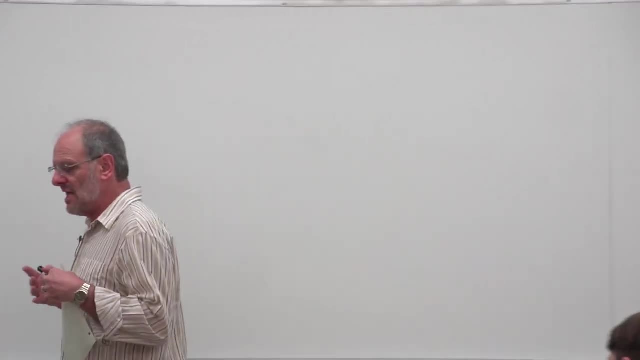 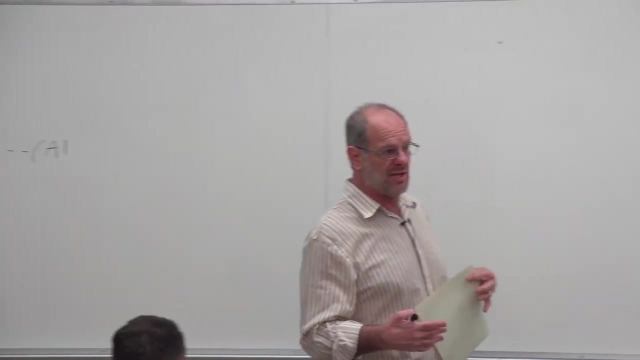 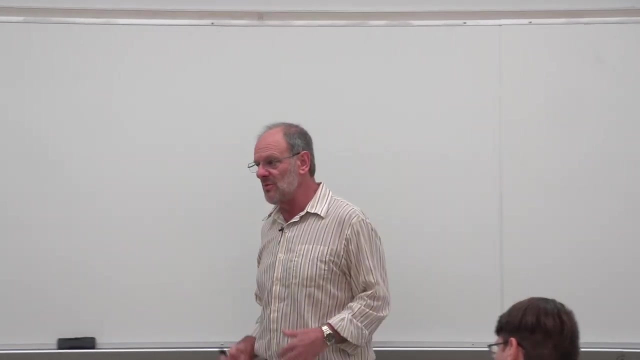 the first thing we talked about last time was omega. We understand that in an air water vapor mixture the relationship between the amount of water vapor and air influences the comfort of that particular air. right With a higher value of the humidity the air becomes less comfortable. With a lower value it becomes more. comfortable, although that's only to a point right. You can have dry air, but at very cold temperatures. that has so little moisture in it that it's not going to have the temperature in it that it hurts almost. Your nose starts to bleed just. 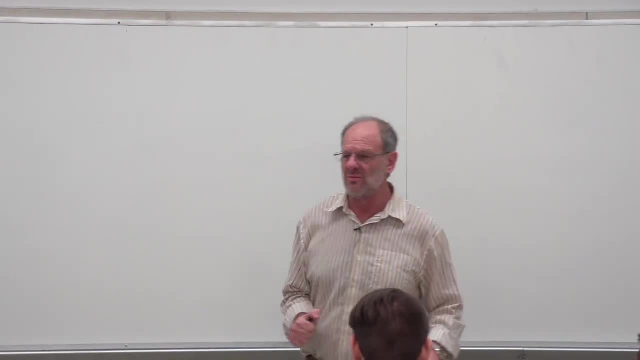 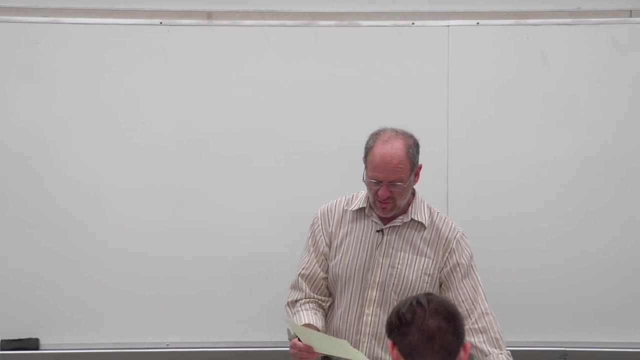 from standing there. just, you know, doing exercise in that kind of an environment, Your skin dries out and all that. So, nonetheless, we do need to understand that there is a relationship between the water and the air. And eventually, when we consider air conditioning processes, you know we'll talk. 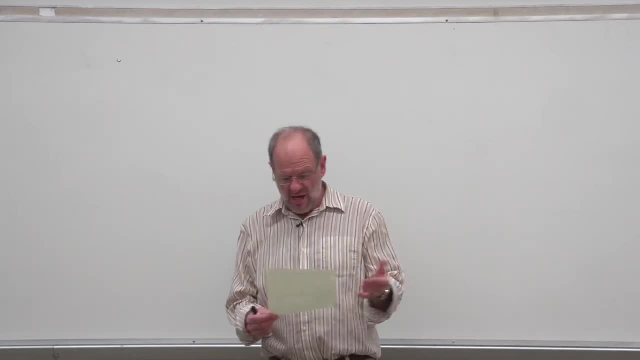 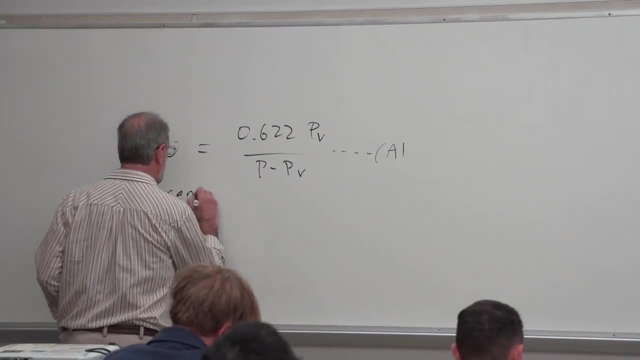 about this in more detail. So, nonetheless, this is the first equation that was derived. It was derived last time as equation A. I'm just going to continue with this now And let's just rearrange this. What I'd really like to do is change this, so it's. 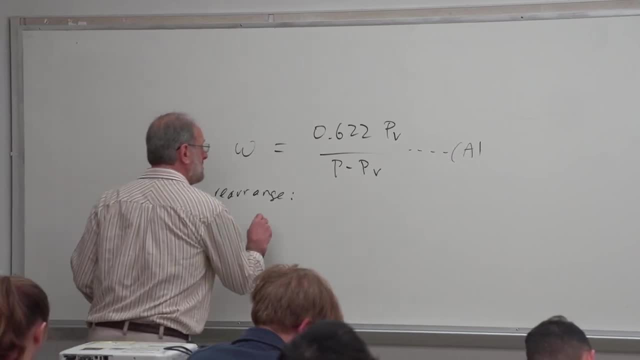 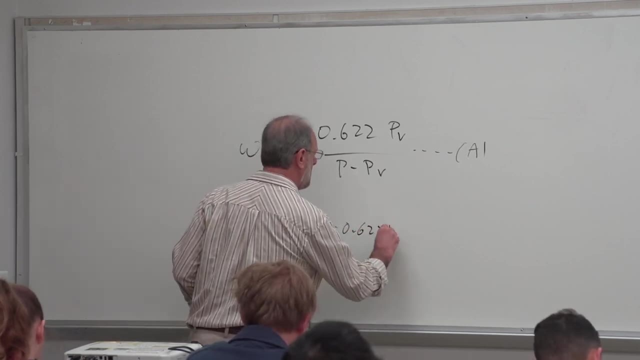 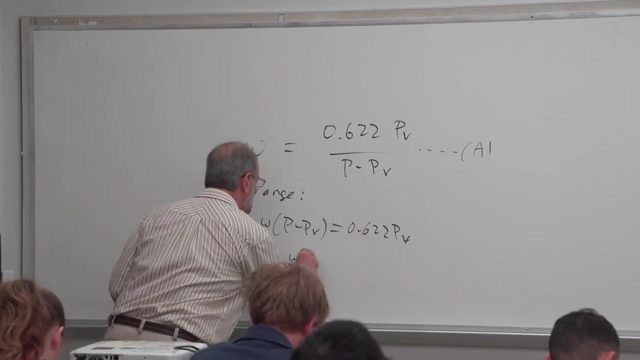 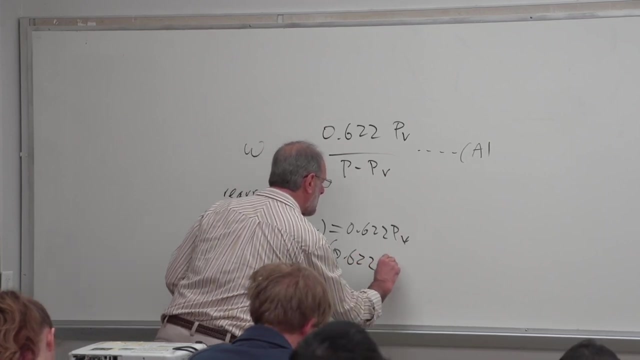 explicitly in terms of PV. So let's just move the P minus PV from the right-hand side denominator to the left-hand side of the equation. Then we'll just rearrange just a little bit. So I'm just going to collect together the PV terms And then, lastly, I'll just 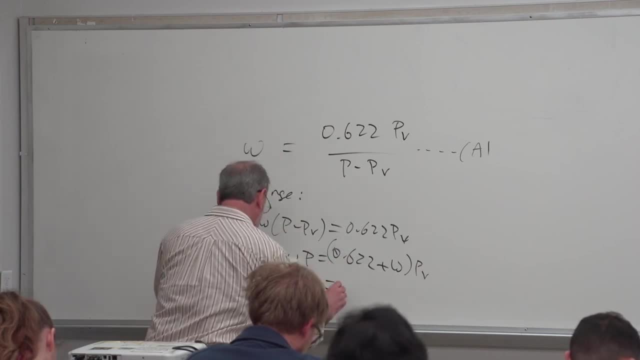 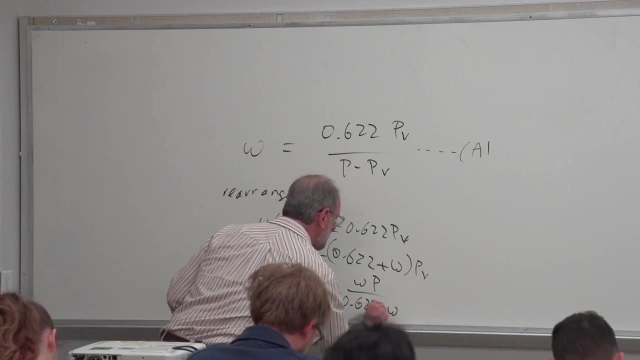 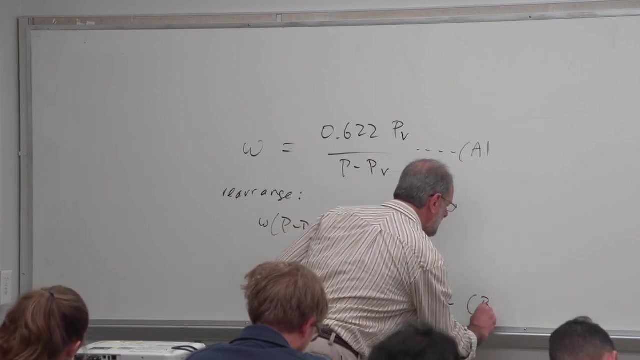 solve this for PV. So PV is just going to equal omega times P over 0.622 plus omega. OK, So this is another equation that is of interest to us. I'm just going to call it equation B. Again, it's really the same as equation A, but it's. 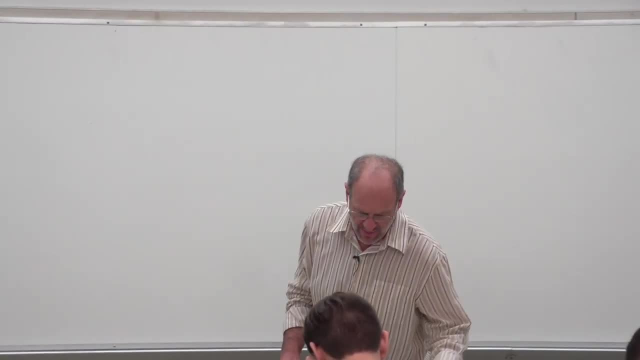 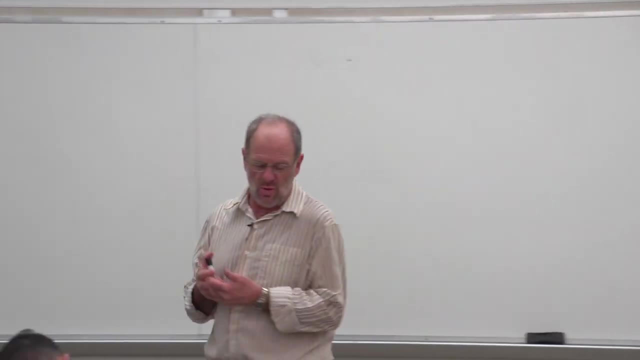 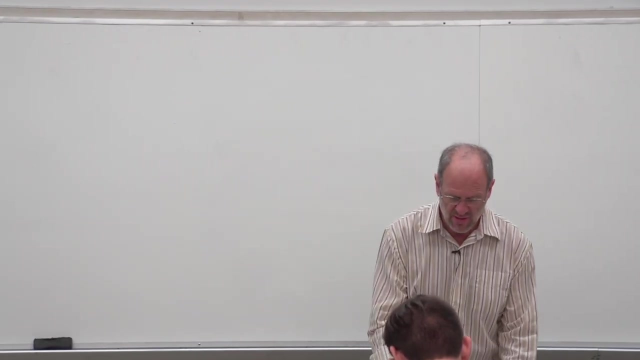 just been rearranged for you. OK, Now, as we continue, let's consider that there's only so much water vapor that can be held within air. OK, Certainly we can add a certain amount of water vapor, But if that amount of water vapor gets, 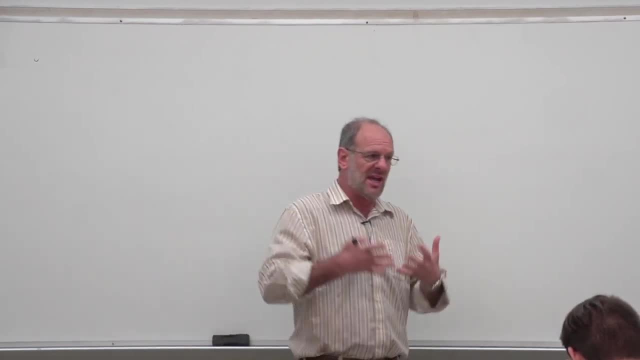 too high, then it can't be held in the air and it's going to have to condense out of the air. When we have water that's condensing out of the air, we just call it dew, right, That's the air that's going to condense out of the air. So 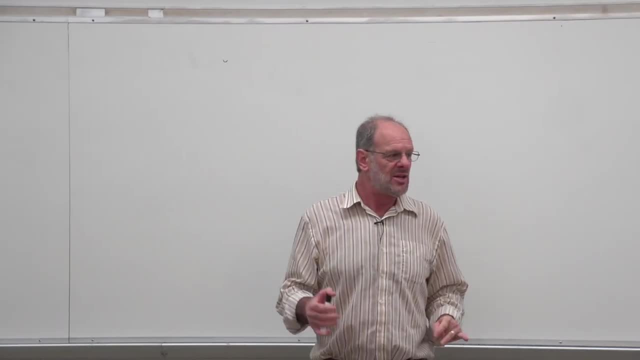 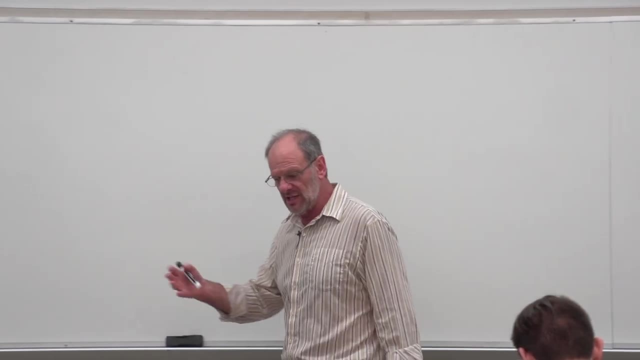 we've seen dew on the grass or on our car in the morning, and all that. So it turns out that this presence of dew is also important to us. There's a temperature that we're going to be able to find in a little while, today, called. 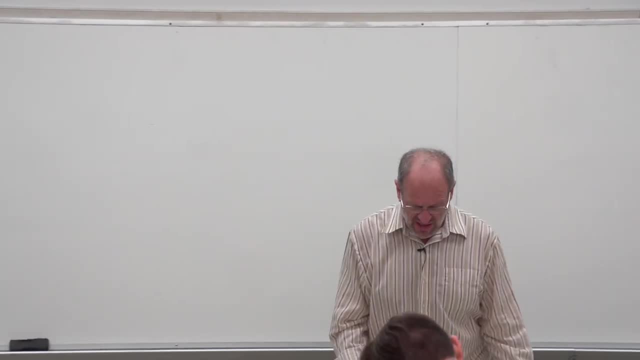 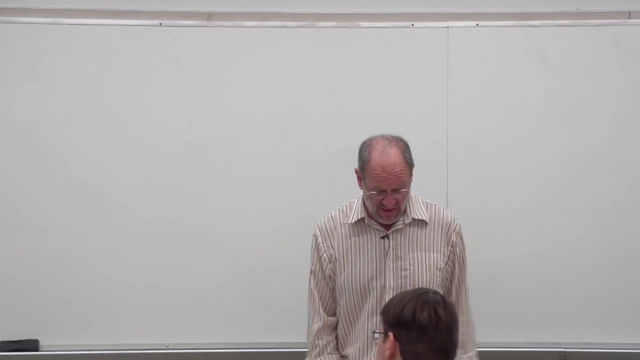 the dew point temperature. But nonetheless let's just note that at any given temperature, air is only able to hold so much water vapor. If we try to add more water vapor then the air is going to condense. I'm sorry, the water vapor is. 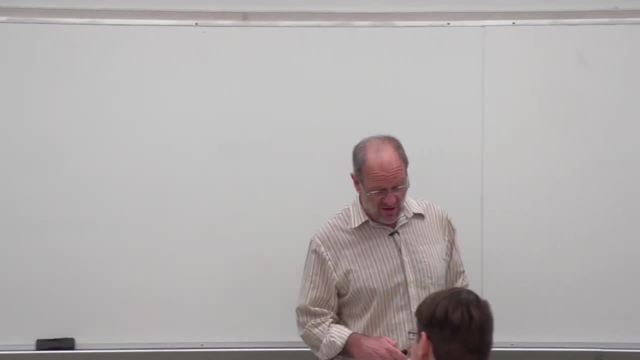 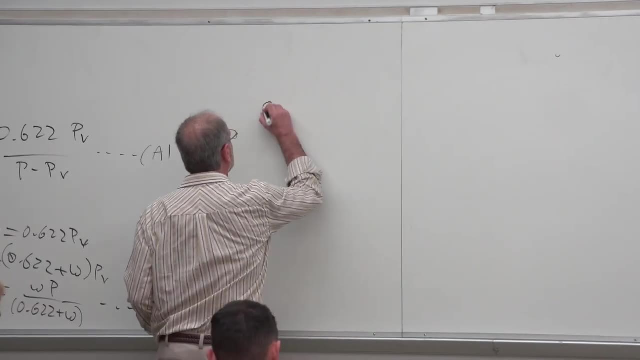 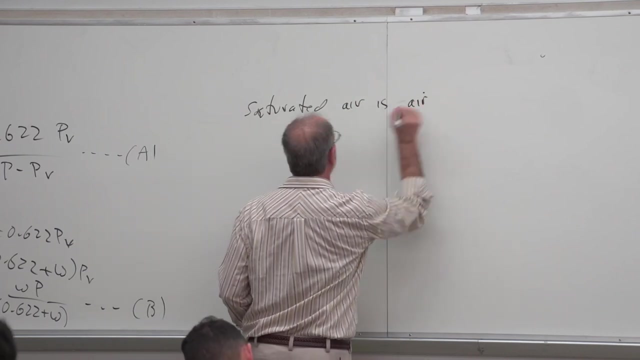 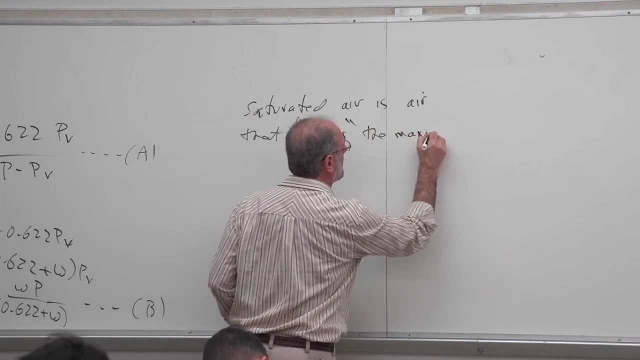 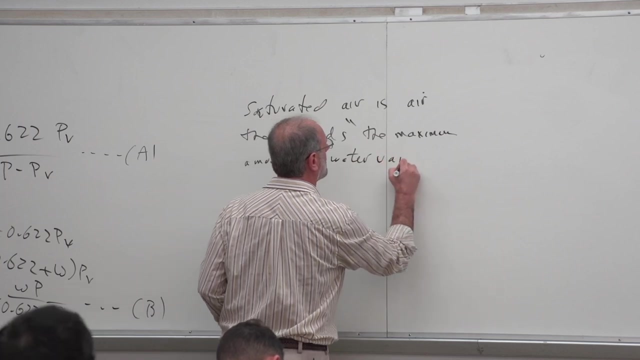 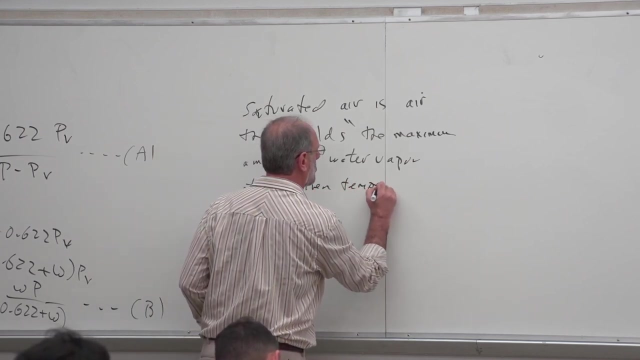 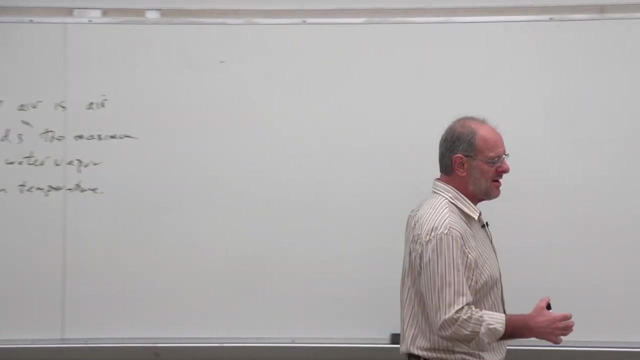 just going to condense out. We use the word saturated air to identify air that's holding its maximum amount of water vapor at any particular temperature. Okay, So saturated air is what I've just been describing. You know we can only have so much air. I'm sorry we don't have so much water vapor that can be held. 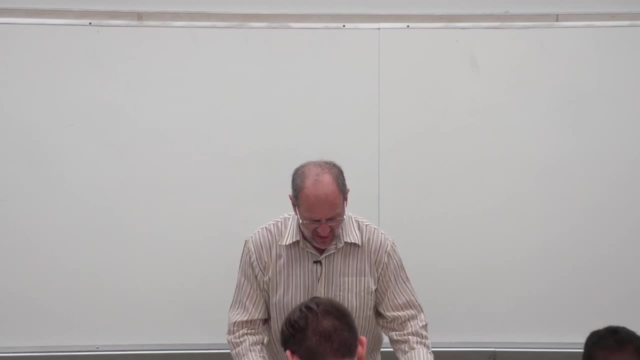 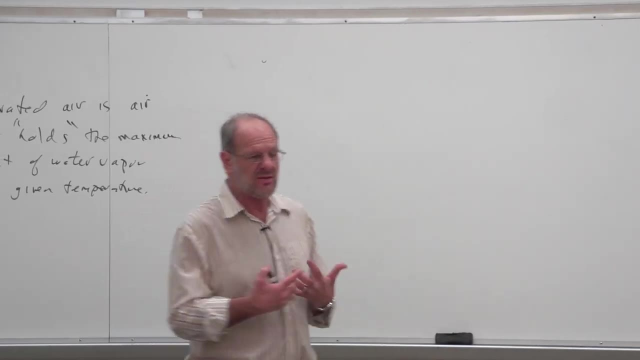 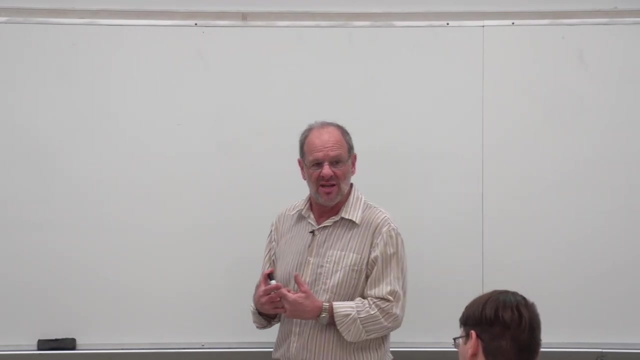 within the airstream as a gas. Now, what would this temperature be? Well, again, mixtures. I'm sorry. when you have a mixture, each component behaves as if it existed, as if it existed alone at that particular I'm sorry. let me rephrase. 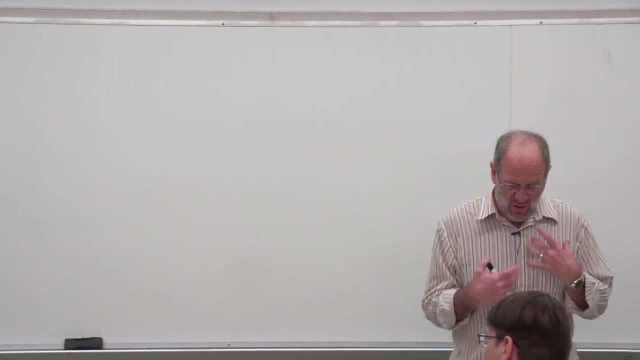 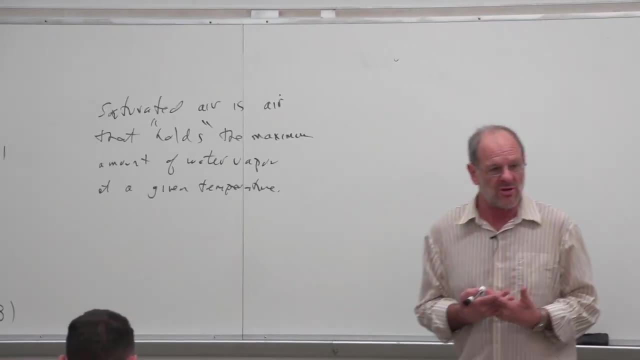 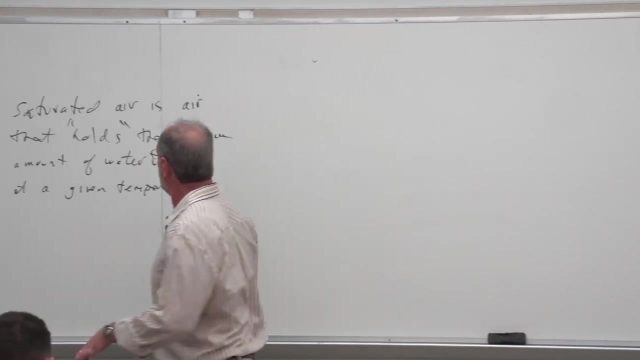 that When we have a two-component mixture, each component behaves as if it existed alone. in the volume of, in this case, the atmosphere, Each one is going to have its own unique partial pressure. right, This partial pressure represents the pressure at which this condensation occurs at, So saturated air is air that. 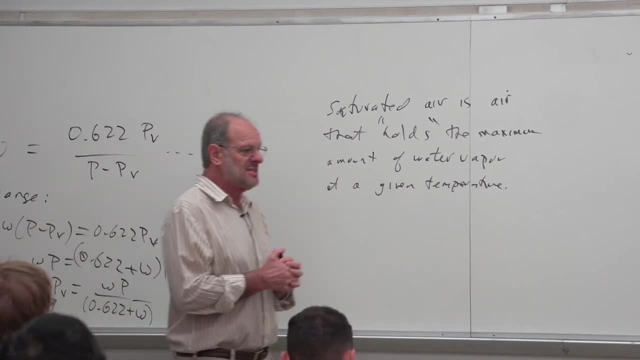 holds the maximum amount of water vapor at a given temperature. This temperature is actually responsible for the condensation. So saturated air is air that holds the maximum amount of water vapor at a given temperature. So saturated air is related to the partial pressure right. The partial pressure is the pressure at 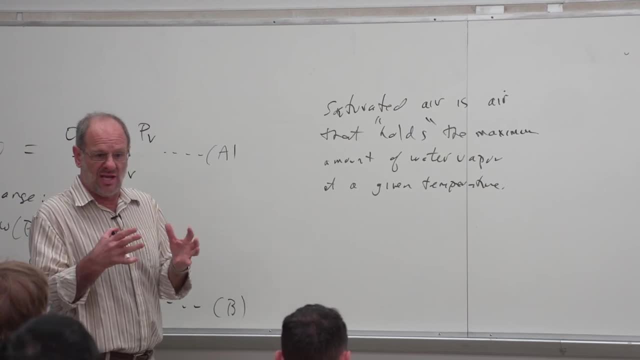 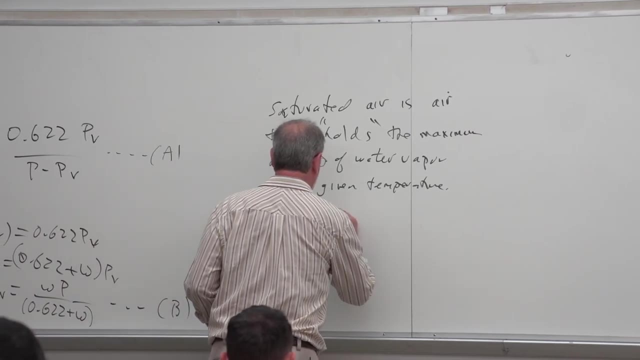 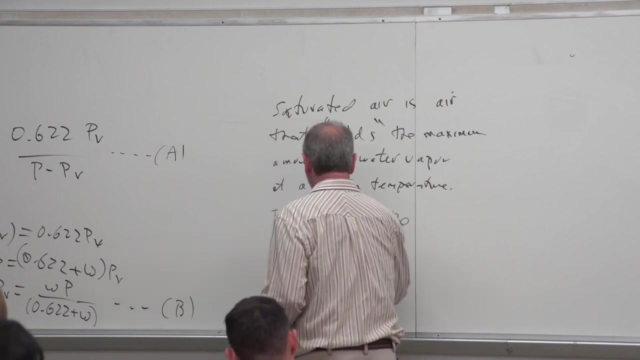 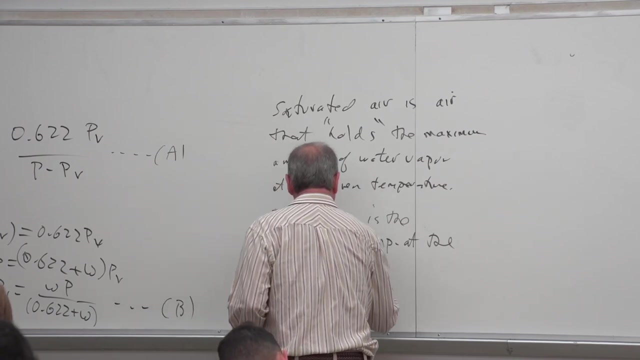 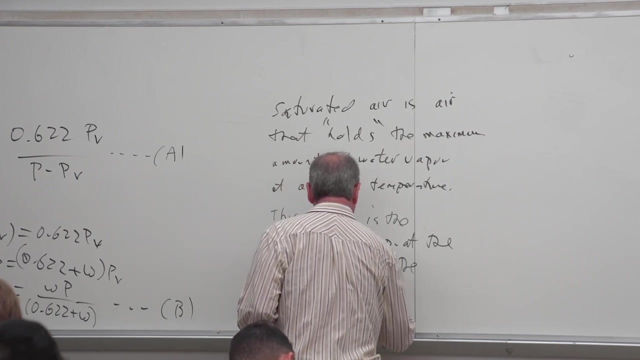 which the water vapor behaves at and when we have a phase change, that phase change is going to occur at that partial pressure. So this temperature is the saturation temperature at the partial pressure of the water vapor And of course you know that PV is how we write the partial pressure of the. 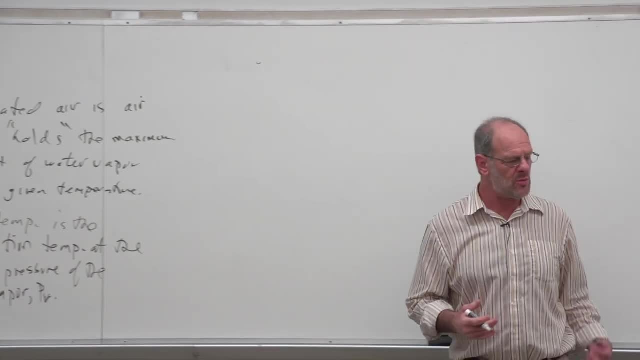 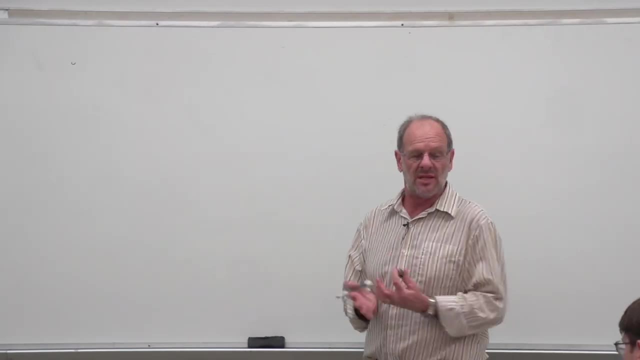 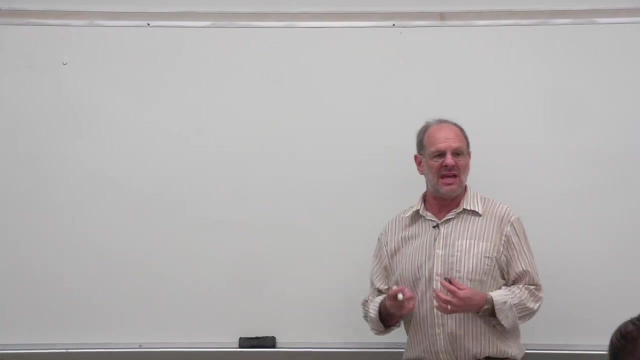 water vapor. OK, So with all this in mind, now we can have a better feeling for calculating what's called the relative humidity. OK, One more thing I want to note here: This maximum amount of water vapor in the air we're just going to. 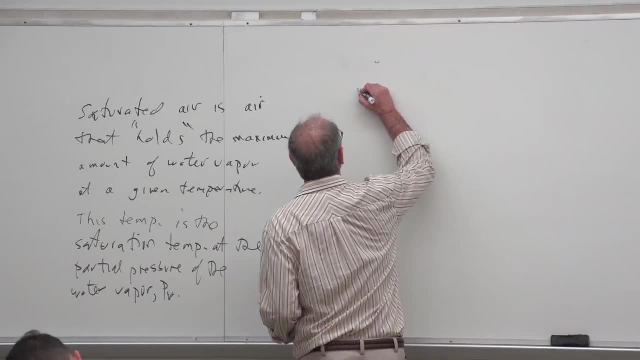 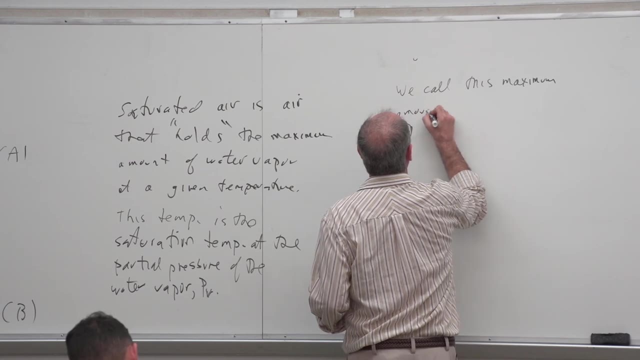 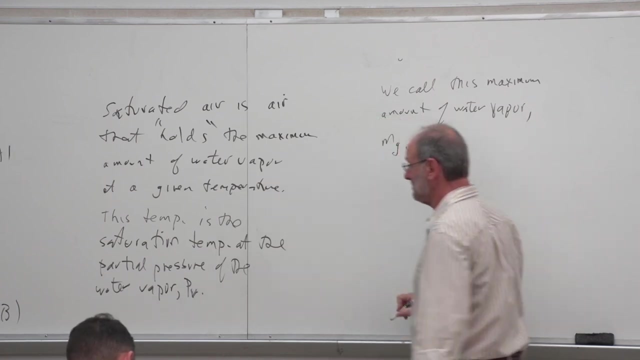 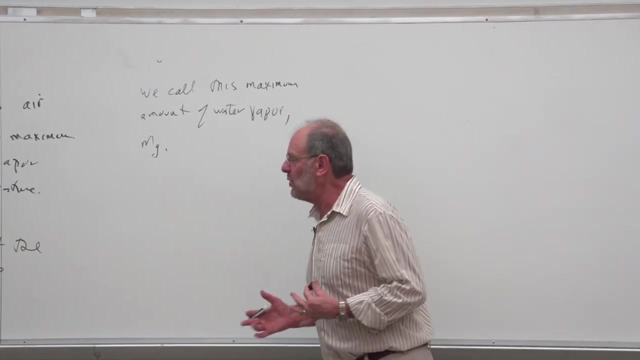 call M sub G. So we call this maximum amount of water vapor M sub G. OK, So now back to the idea of relative humidity. We talked about this briefly last time. The problem with the absolute humidity omega is that the absolute humidity is. 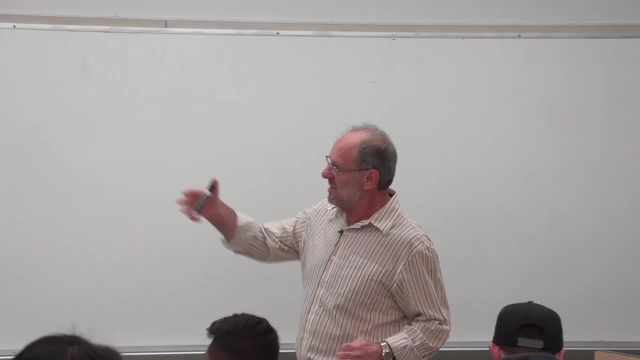 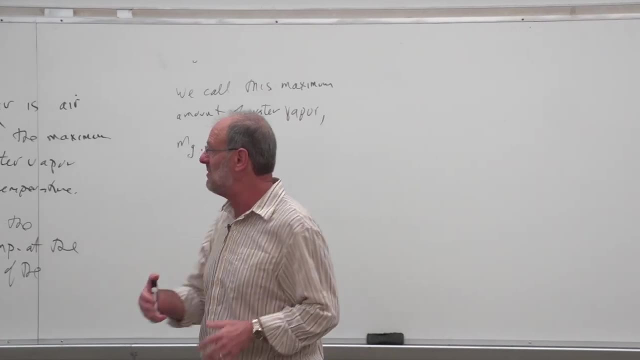 relative. Well, maybe I shouldn't say the problem with it, But one issue regarding it is: it really only tells us the relationship between the amount of water and the amount of air, I should really say the amount of water vapor and the amount of dry air, But often we're interested in how much water vapor. 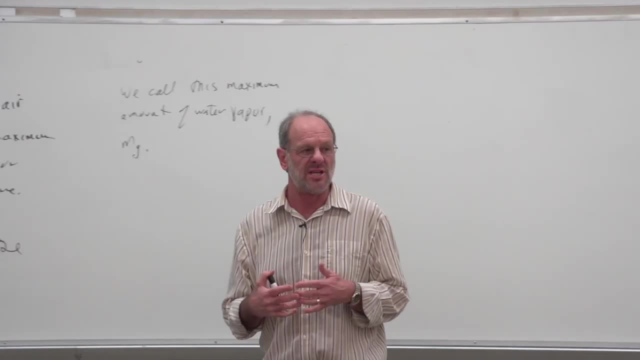 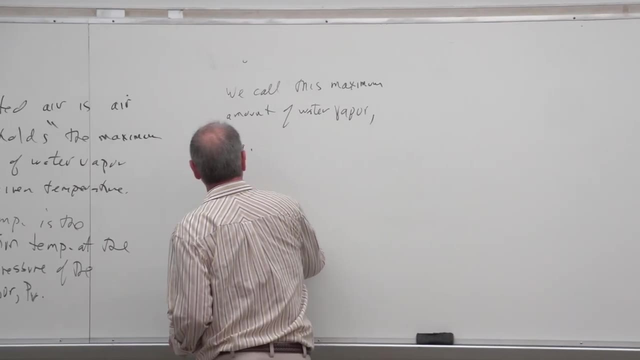 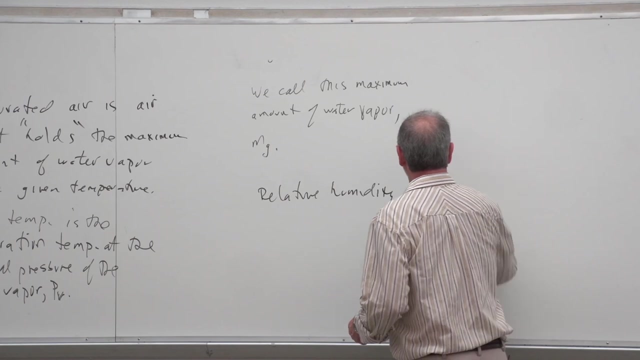 theoretically could be held in the air at any particular temperature, And this is where we come up with the concept of the relative humidity. So we're going to define the relative humidity. First of all, the relative humidity is going to be using the Greek letter phi. 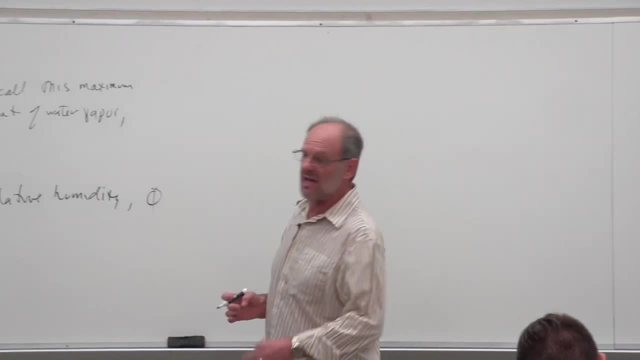 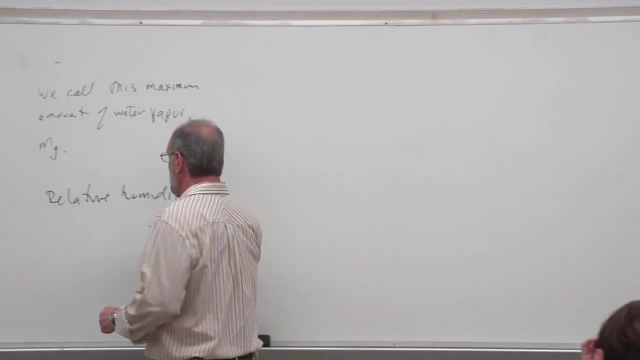 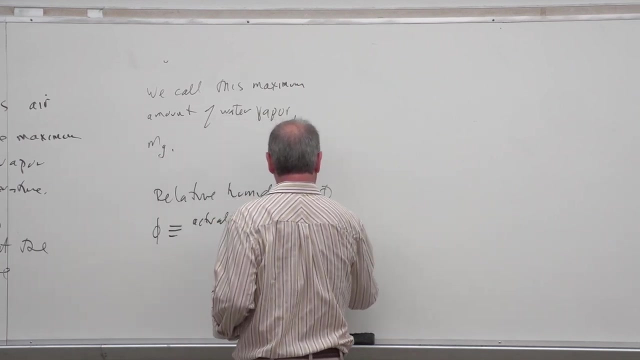 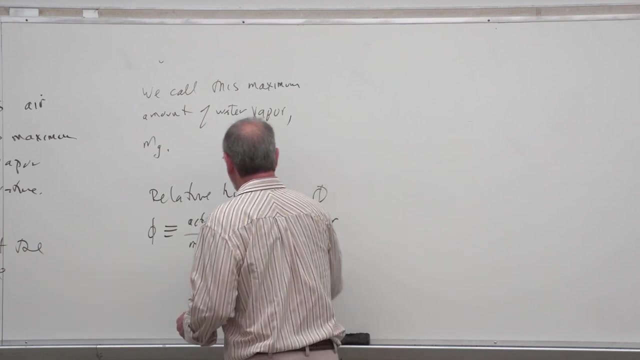 And then we're simply going to define the relative humidity as the actual amount of water vapor in the air divided by the maximum possible amount of water vapor in the air at that temperature. Maybe I should really say actual mass of water vapor in the air divided by the 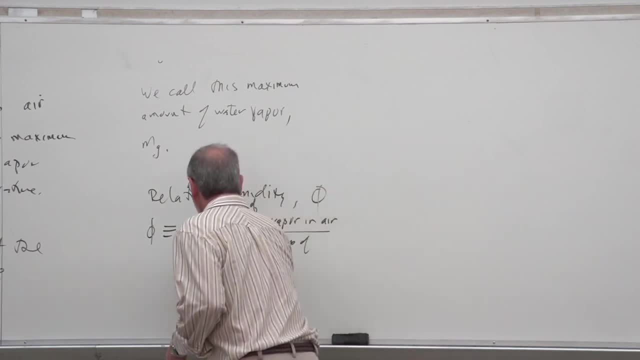 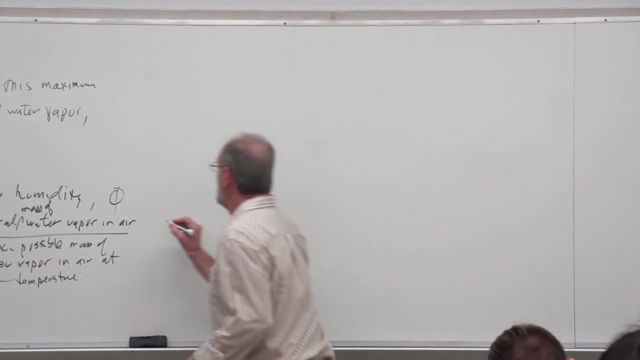 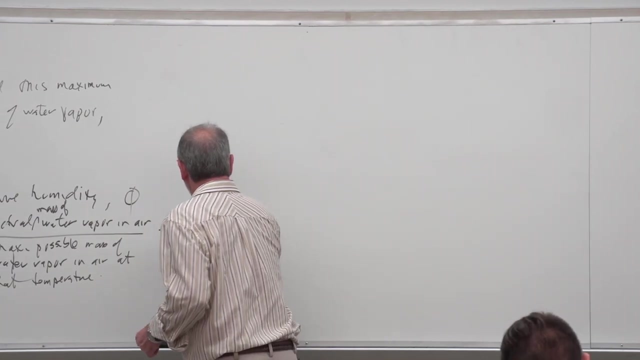 maximum possible mass of water vapor in the air at that temperature. OK, So we know that the amount of water vapor is just M sub V, right, That's the amount of water vapor And we know that the maximum possible amount of water vapor at any 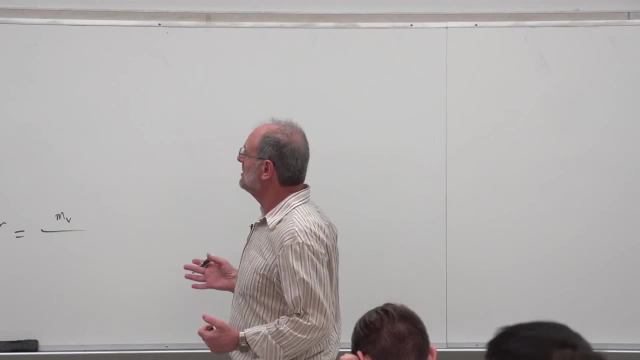 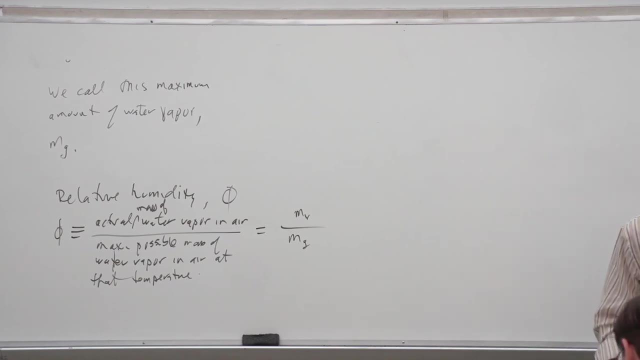 particular temperature, based on our previous definition, is just M sub G. So now what we'd like to do is we'd like to somehow utilize equations that we already know so that we can find a mathematical expression for this, hopefully in terms of some of the other data that we've already seen, specifically in 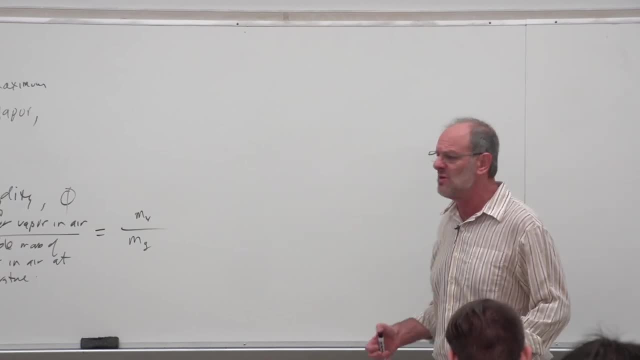 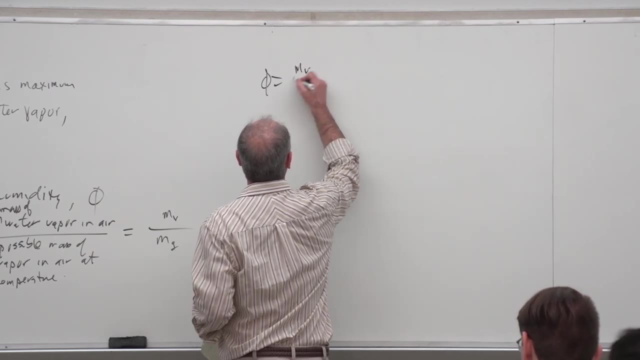 terms of omega, or perhaps some of our partial pressure. So we're going to use that- Perhaps some of our partial pressures, that we would already know. So let's just note- next then Let me just rewrite this- That we're still talking about air, as 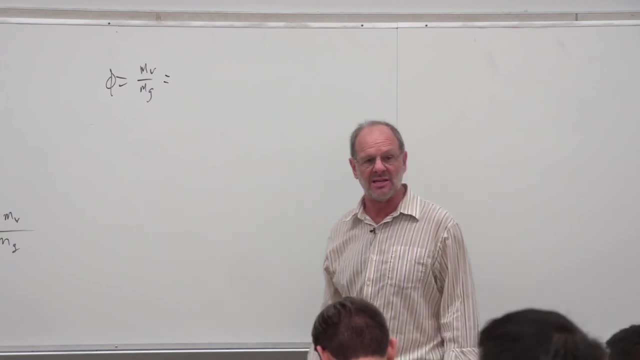 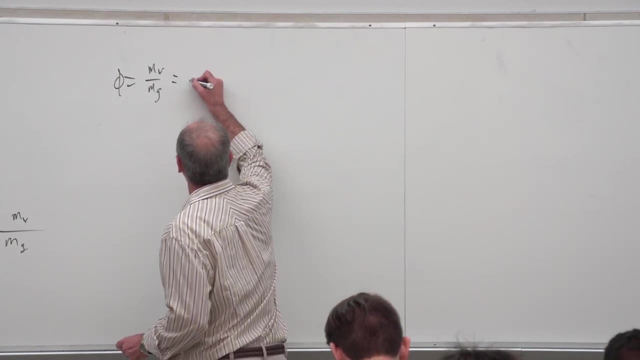 an ideal gas. We're still talking about water vapor as an ideal gas, So we can certainly use the ideal gas equation of state. We know that PV equals MRT, So we could just substitute the ideal gas equation in both for the actual amount of. 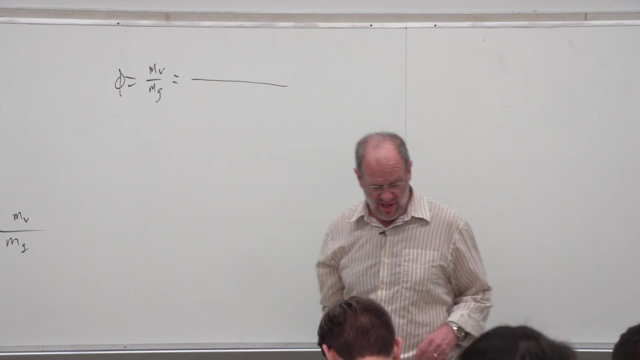 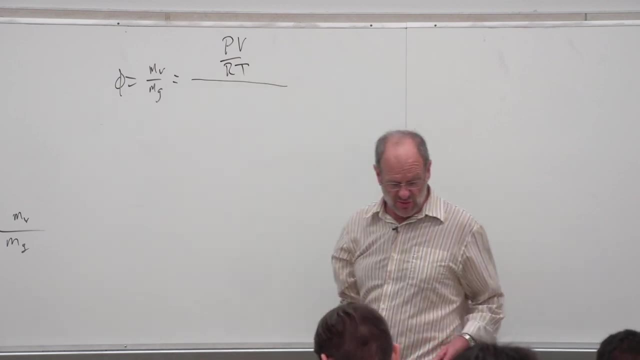 water vapor in the air and the maximum amount of water vapor in the air. So this is just going to be PV over RT, So PV over RT, And let's make sure that we identify this as the water vapor's partial pressure and the gas constant for the 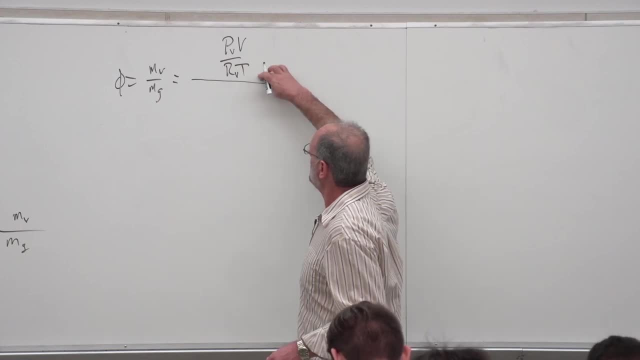 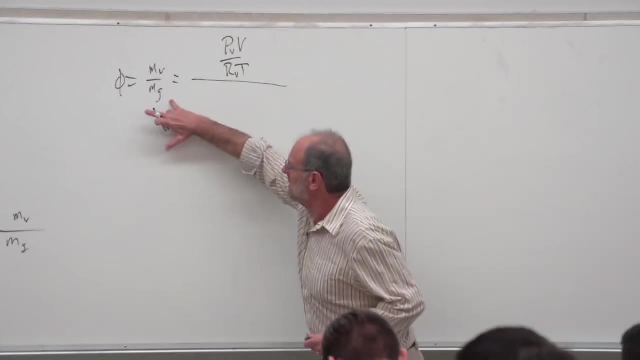 partial pressure, I mean technically the volume and the temperature are going to be for the actual amount of water vapor in the air. But remember that when we try to find Mg, we're assuming that we're at the same temperature. So we're going. 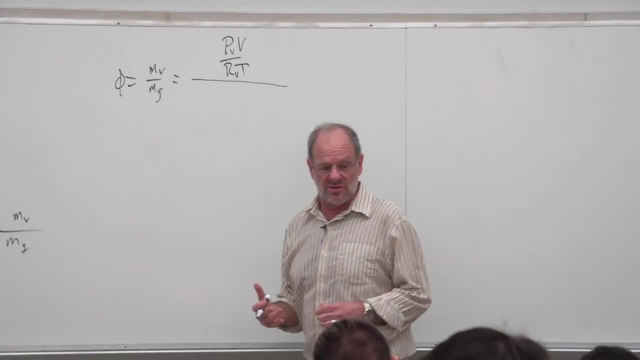 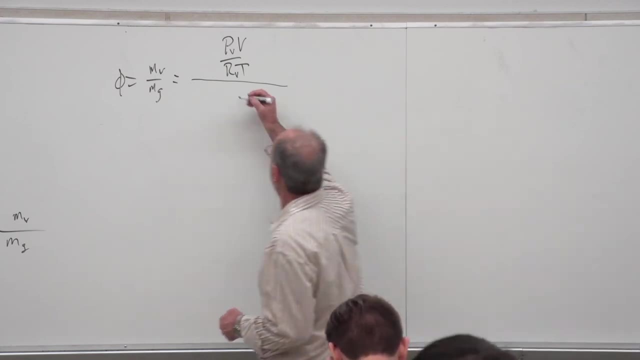 to be at the same temperature. We're assuming, based on our understanding of mixtures, that the volume that's assumed to be occupied by each component, in this case the water vapor component, is going to be the same, So we could just write. 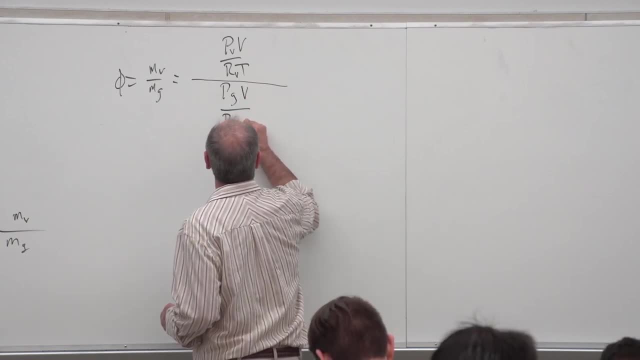 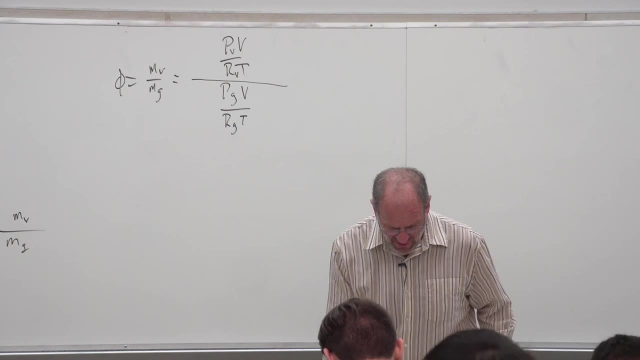 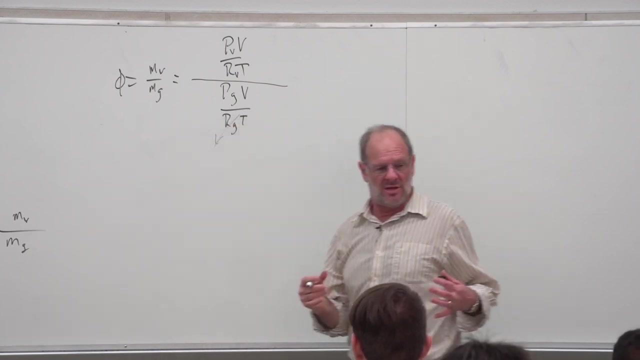 this, then, as PGV over Rgt. Okay, And let's note further that even Rg- I mean this- is just the gas constant, right? It doesn't matter whether we're talking about the actual amount of water vapor or the actual amount of water vapor, But 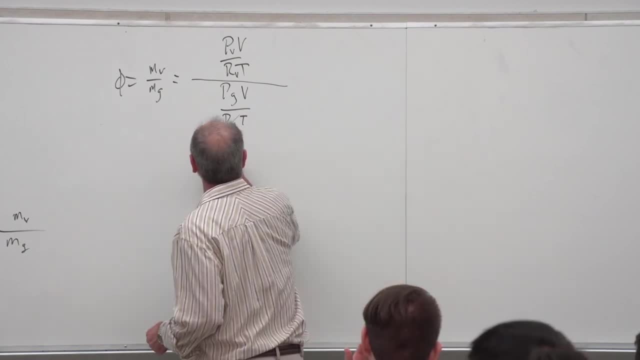 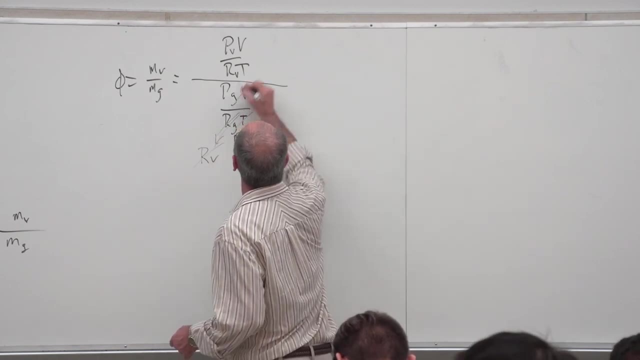 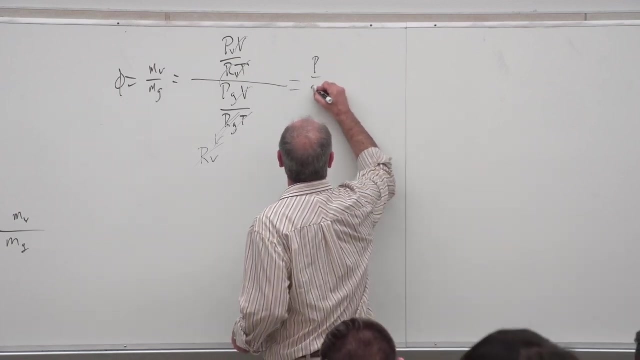 it's just the gas constant. It's a constant, It's equal to RV. So, with all this in mind, essentially everything cancels out. The gas constant cancels T constants, T cancels V cancels. All we're left with, then, is P over P sub G. So 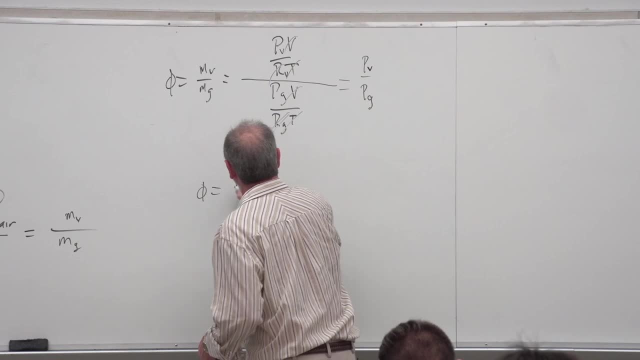 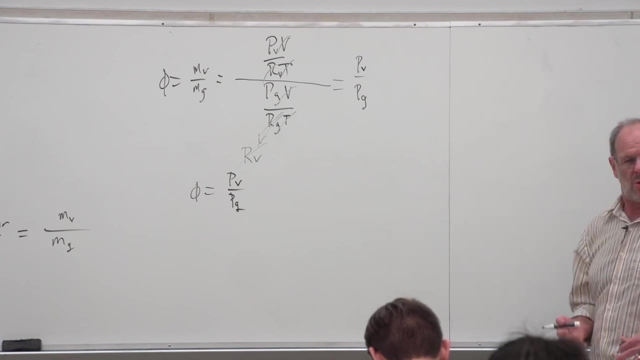 the relative humidity. whoops, I'm sorry. PV over P, sub G. The relative humidity is just going to be the partial pressure of the water vapor divided by the partial pressure of the water vapor at its maximum value, And let's keep in mind that. 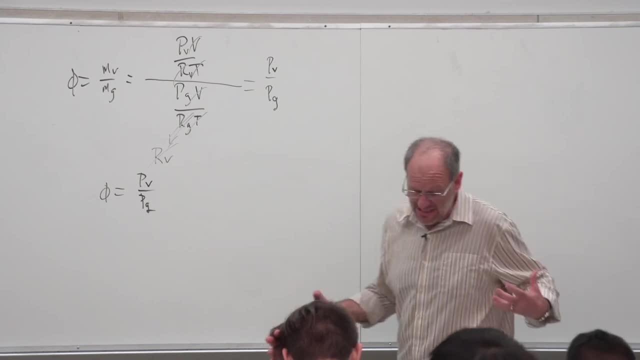 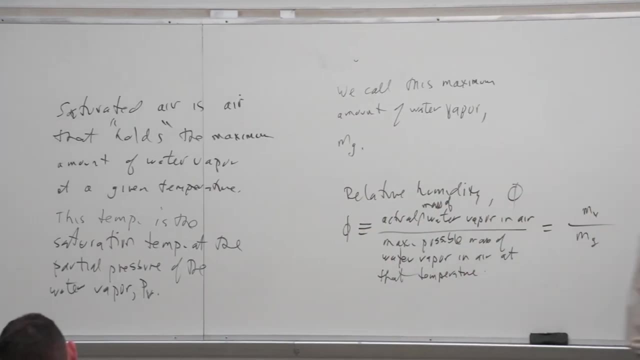 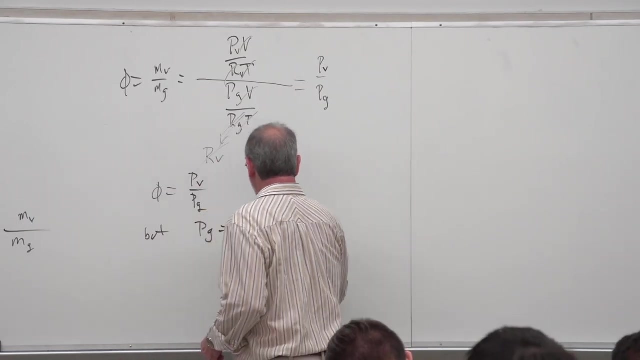 as was just discussed before, this pressure is nothing more than the partial, I'm sorry, is nothing more than the saturation pressure at the existing temperature. So I'll just note here: But PG is equal to Psat at the temperature of the air. 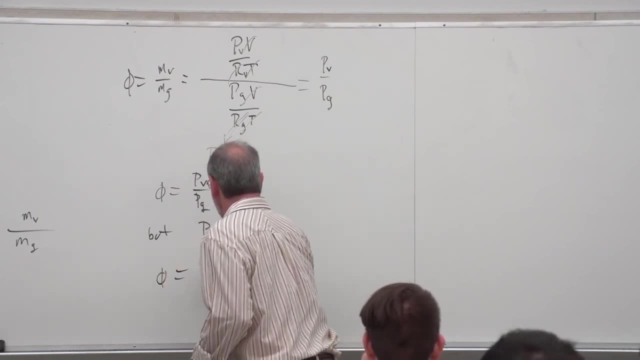 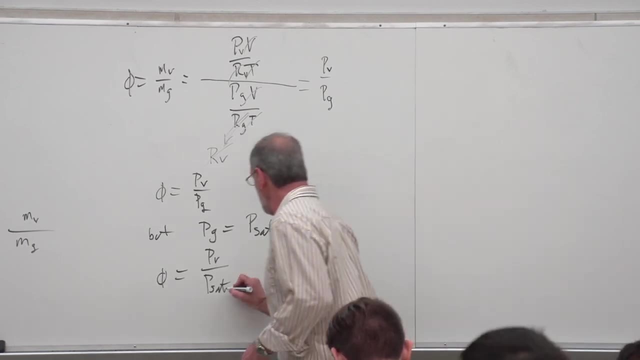 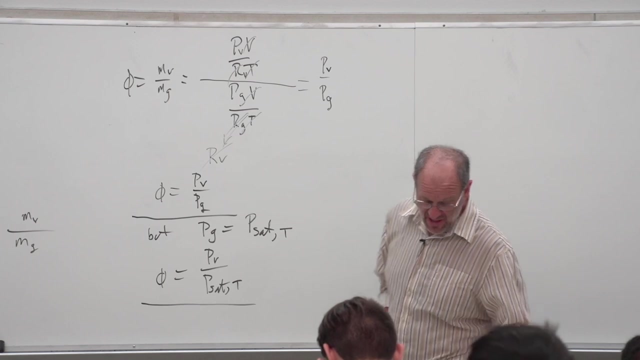 So, phi, we'll just write now as PV over Psat, And again, this would have to be at the appropriate temperature. So this is the general equation. This is just another way of writing, essentially the same thing. The next thing I would like: 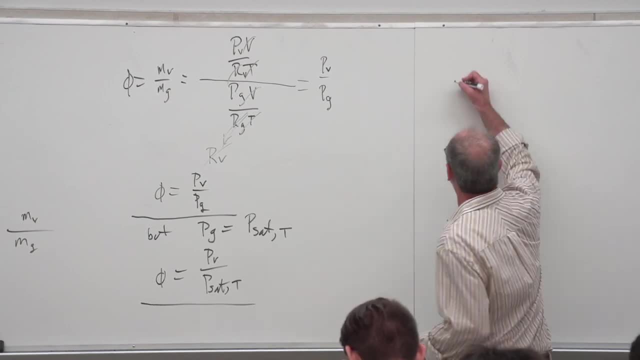 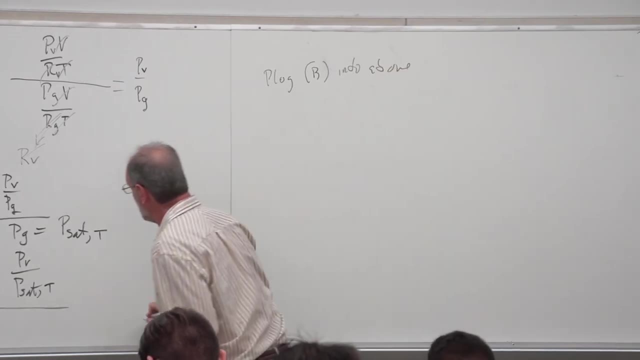 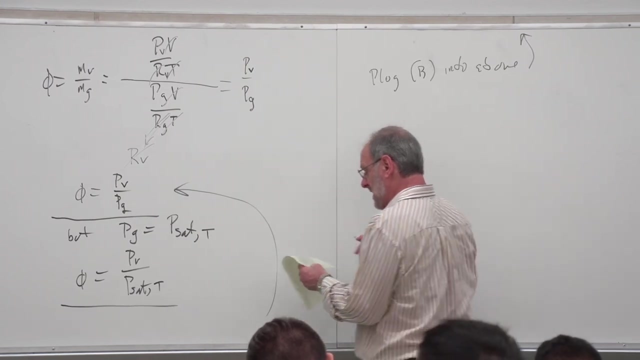 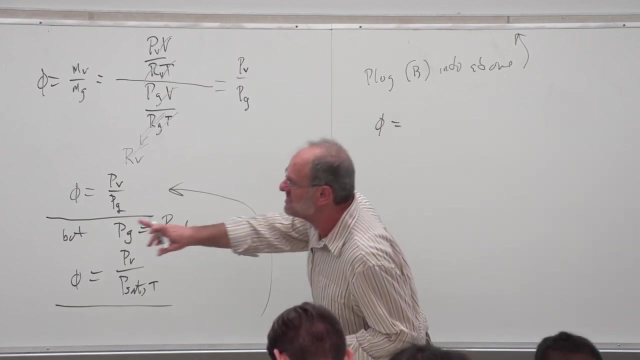 to do, though, is I'd like to plug B into the equation above, And I'm actually going to plug it in To this upper equation, So let's just plug in our numbers. We get that the relative humidity now is equal to, so equation B has been written in terms of PV. 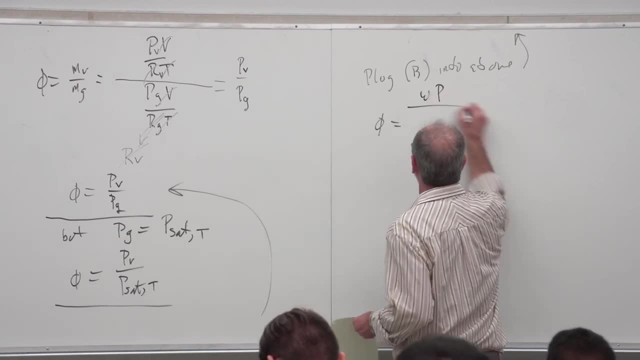 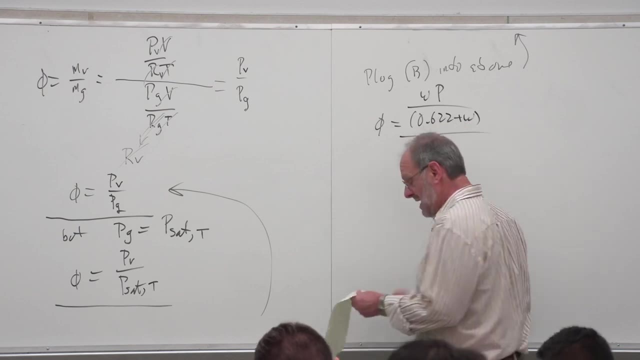 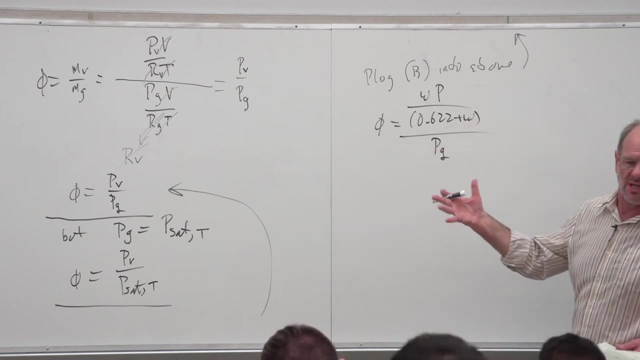 So instead of PV I have omega times P And then divided by .622 plus omega, And then this whole thing has to be divided by the saturation pressure at that temperature. I'll just leave it as PG- And this is really consistent with the. 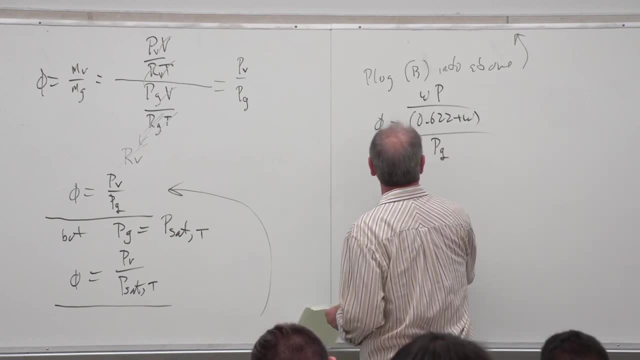 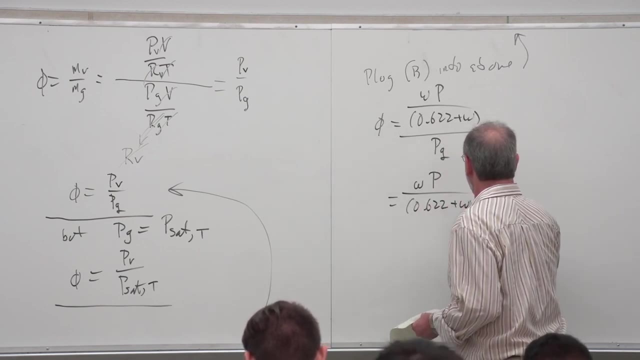 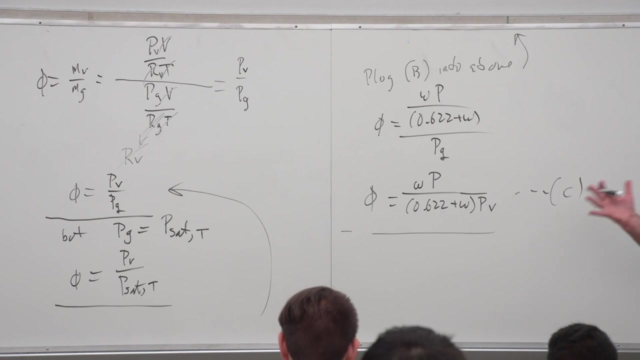 notation in your textbook. And then this just has to be rearranged a little bit So W, I'm sorry, omega times P, And then over .622 plus omega times PV. So this equation I'm going to call equation C, And you know this is a good 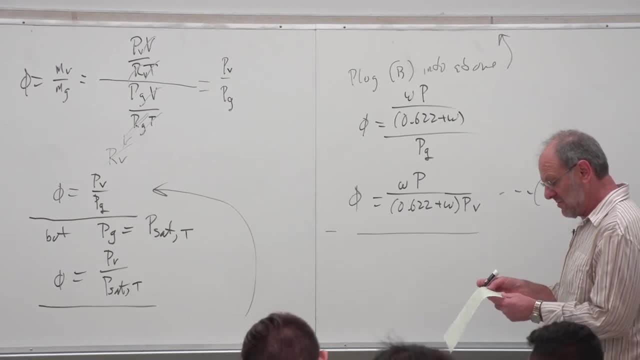 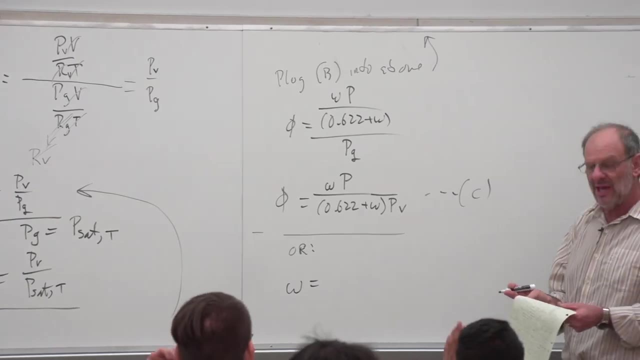 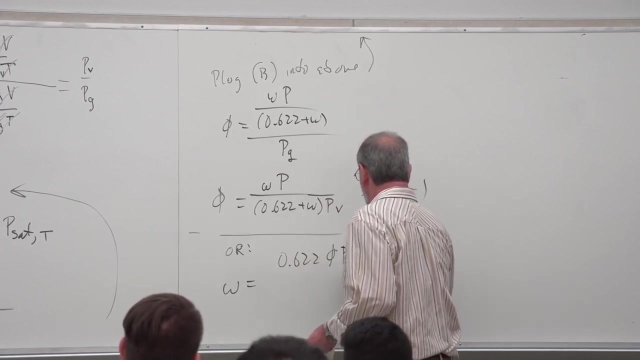 relationship between the absolute humidity and the relative humidity. Sometimes we rearrange this equation to express it in terms of omega, And I'm not going to go through all the steps here. But if we do so we get .622 times the relative humidity, times the saturation pressure at that particular temperature, And then 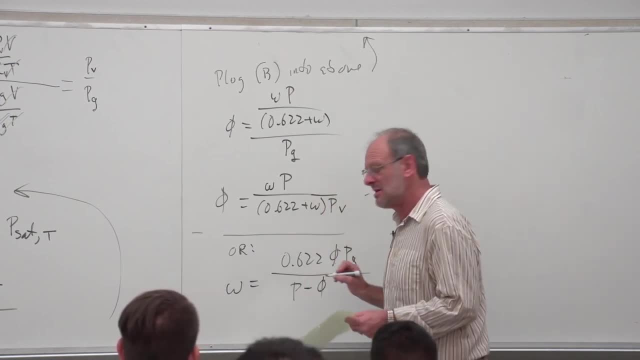 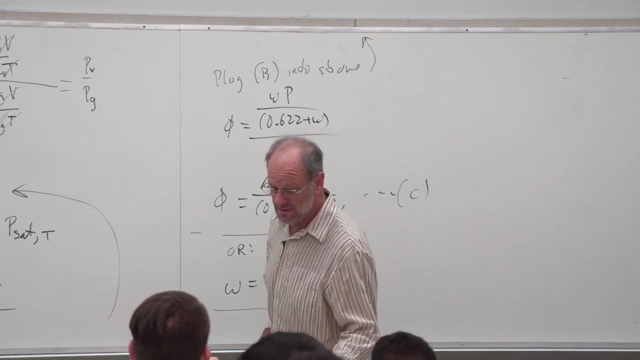 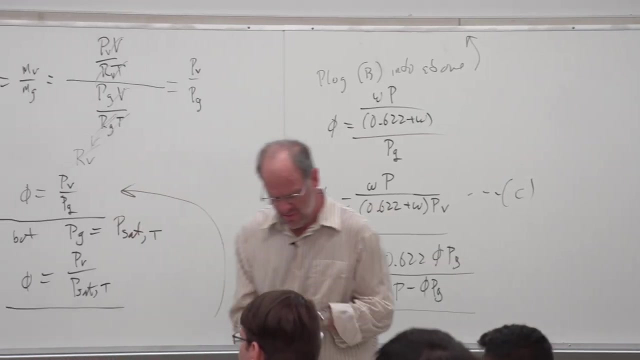 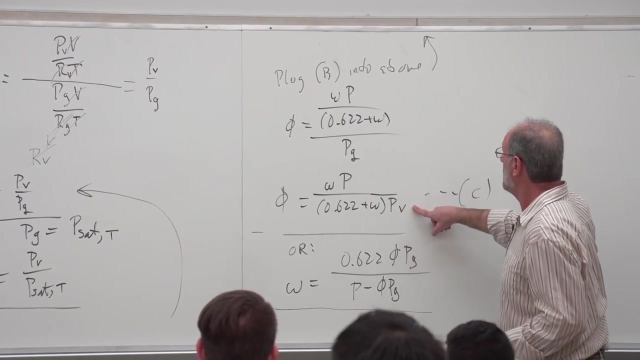 divided by P minus the relative humidity times, that same saturation pressure. So this is another way of writing equation C. Yes, For equation C shouldn't it be PG, not PV? Well, I've subbed in You're talking about here. I've substituted in. Oh wait, 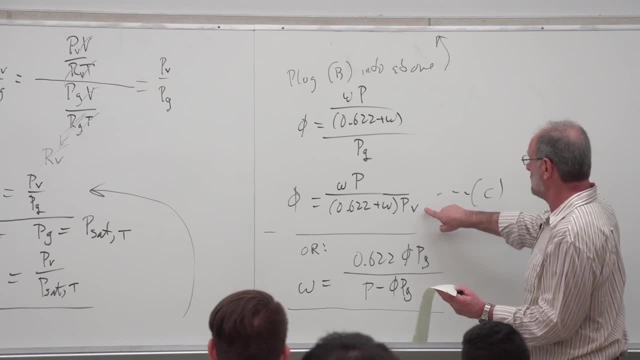 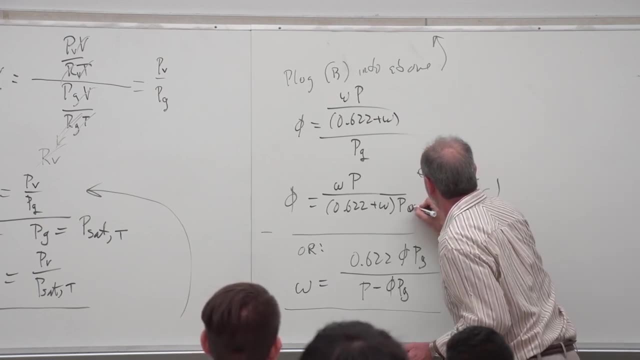 Did I miss something? Yeah, this should be PG. Yeah, I've just made a typo as I've gone from one step to the next, So you're right. Sorry about that. Right, so this is PG. The PG should stay in the denominator And the PG should stay in the denominator. 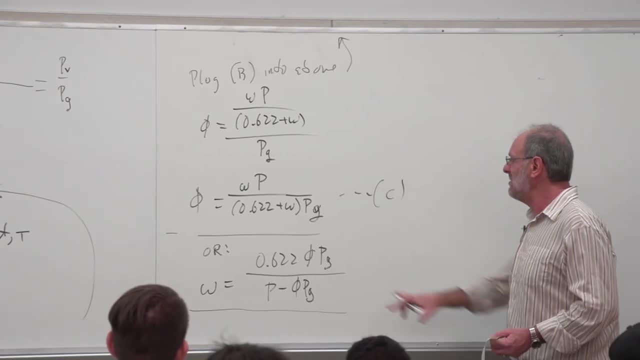 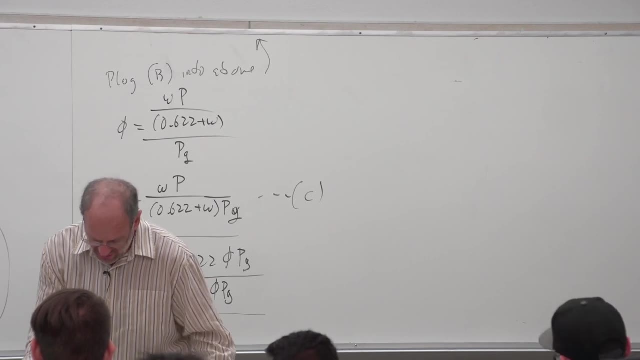 denominator and I just wrote it wrong, So please correct your notes. And yeah, then, these are pg's here, as shown. Okay, Well, I will certainly give you an example problem here shortly, but we're not quite there yet. So a couple of. 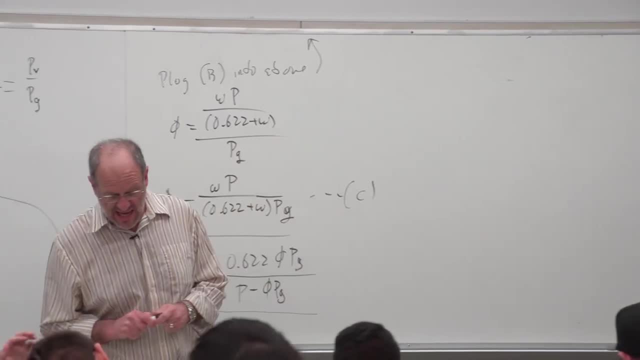 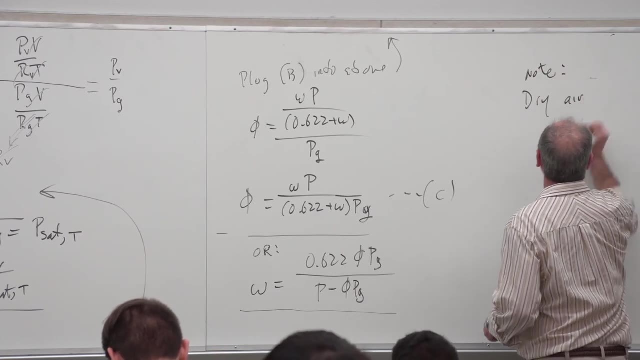 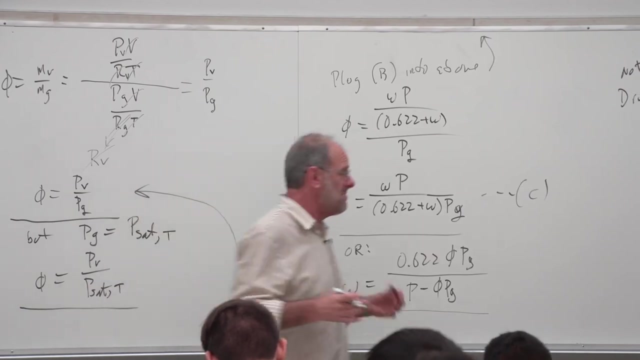 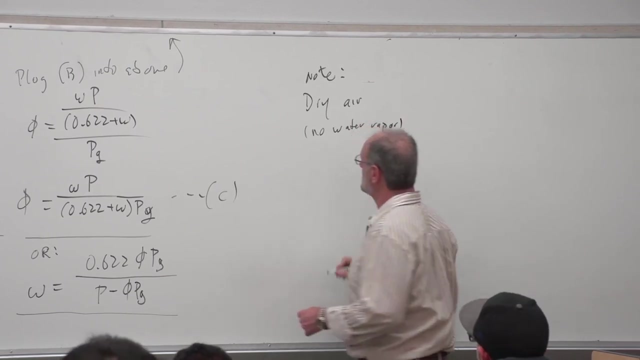 things to note. now, If we happen to have dry air, then I would note that we use the phrase dry air to refer to air that has no water vapor in it. Okay, So dry air means no water vapor at all. This is extremely unusual anywhere in the 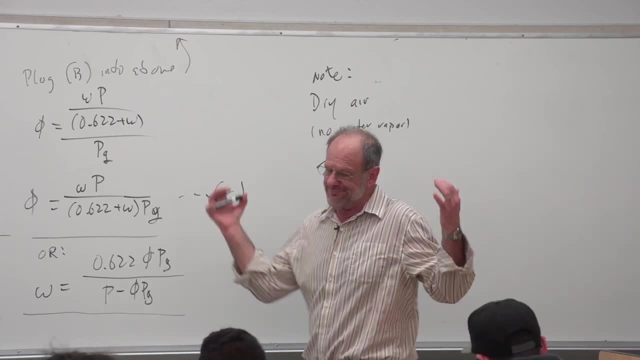 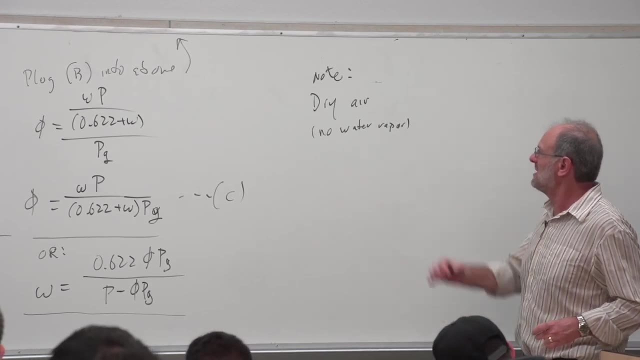 world. I mean, you can go into the middle of certain deserts of the world, you know, like Death Valley or the Sahara in some places, and there's no water vapor at all in the air. Or, you know, maybe it's down to some small fraction of a. 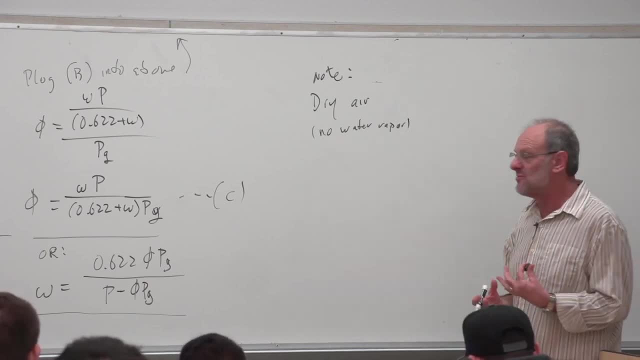 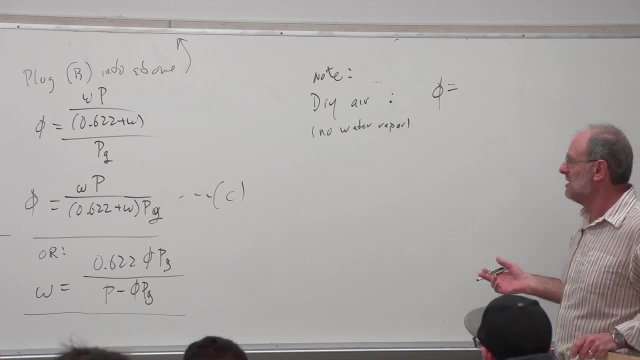 percent. But here we'll just say in general: if we have a lot of air, then we have dry air. That means there's no water vapor. And what would the relative humidity be? Well, it would have to be zero, right, I mean, if there's no water. 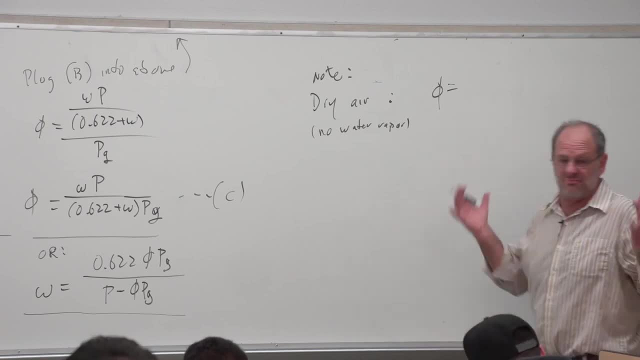 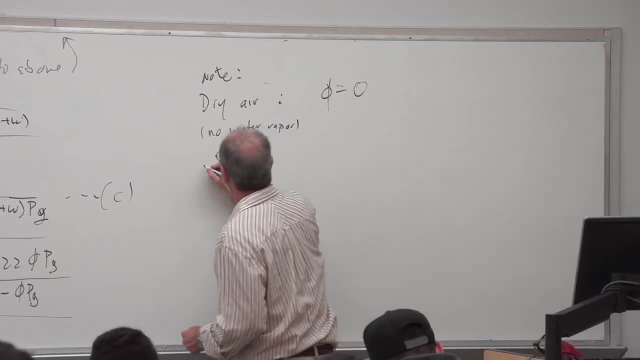 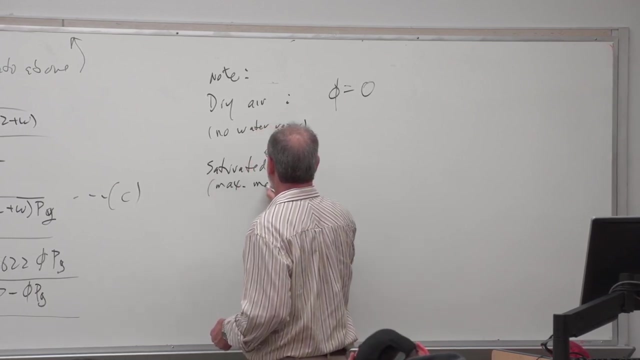 vapor in the air, then well, there's zero in the numerator, just based on our definition of the relative humidity. So this is equal to zero, right? On the other hand, if we have saturated air, okay, this means we have the maximum mass. 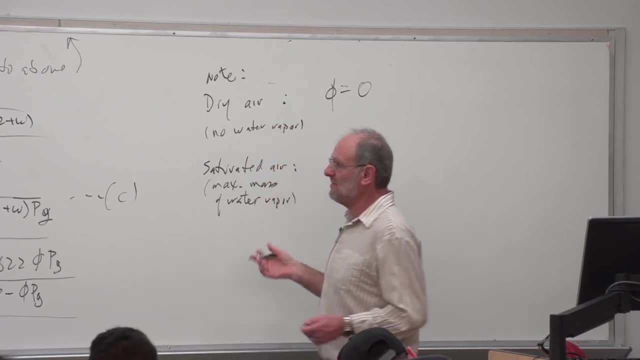 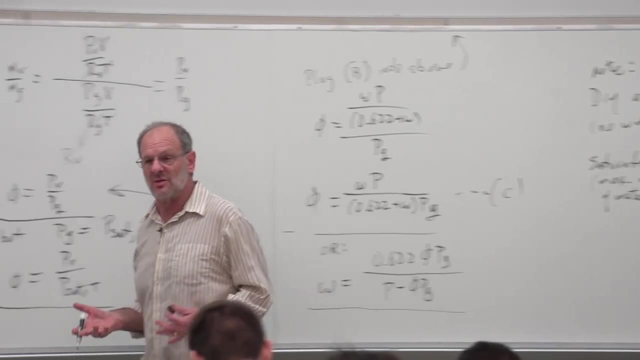 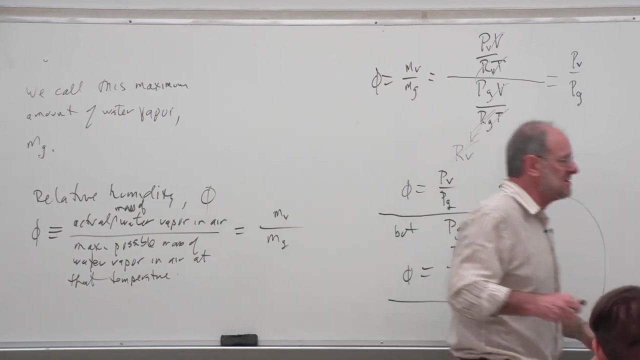 of water vapor Right At the given temperature, as defined earlier. In that case, what would phi be? Well, in this case, phi is just going to have to equal one right. I mean. after all, the actual amount is the same as the maximum amount. mv equals mg. So 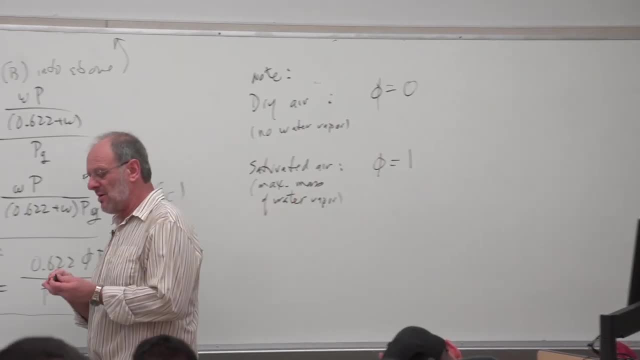 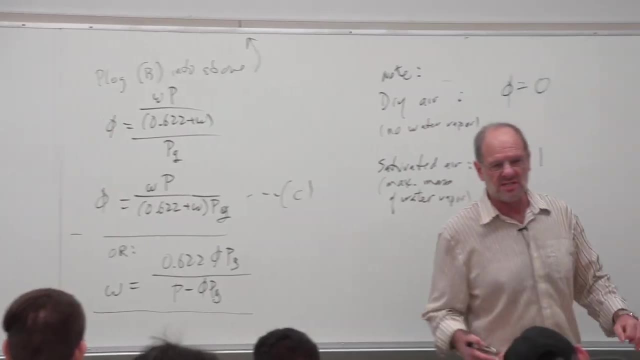 this is just going to equal one. So when we talk about humidity, like on the television and our weather report, the relative humidity is always between zero and one, right I mean it's often expressed as a percentage, so between zero and 100%. 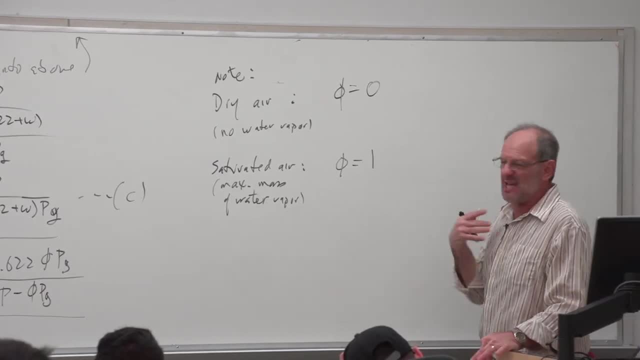 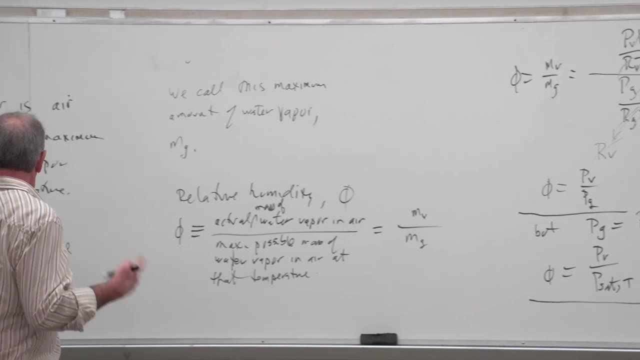 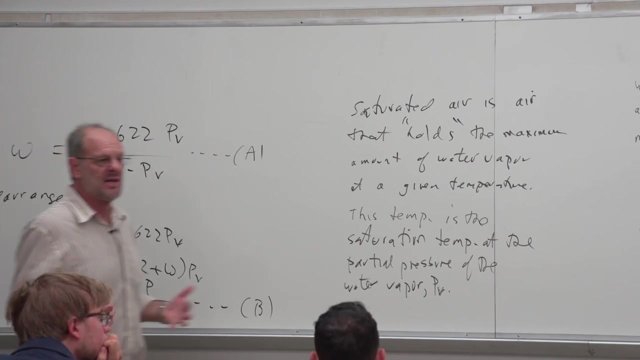 You know this is interesting but again, personally I would much rather we understand absolute humidity. I mean, the relative humidity again is interesting, but in solving problems relative humidity is meaningless to us. We need the actual relationship between the amount of water vapor and the dry air. So 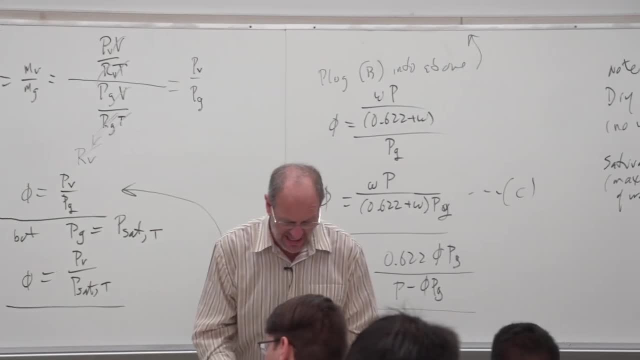 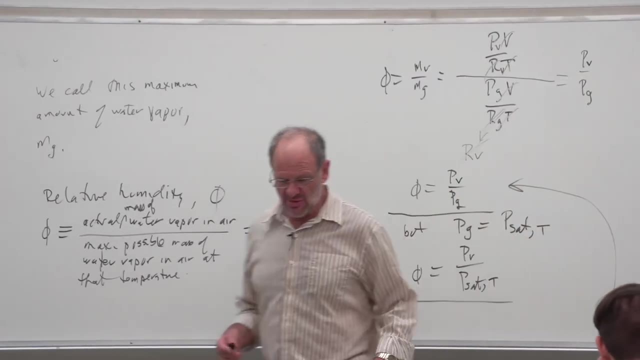 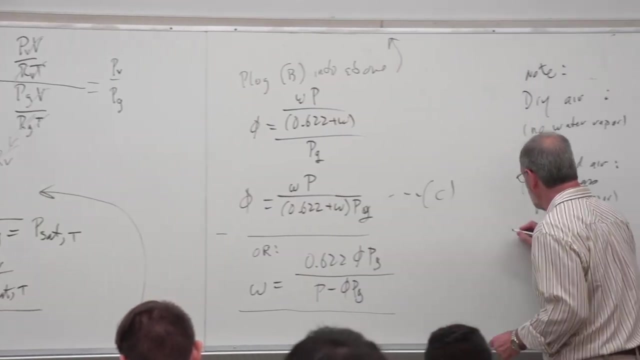 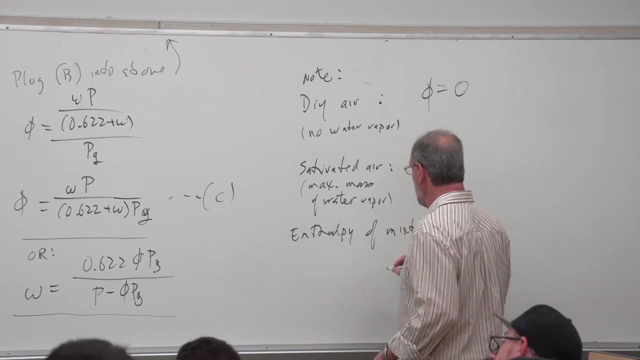 we would typically use omega data, not phi data. In other words, absolute humidity, not relative humidity. Now, another thing that we're going to need as we start going through problems is the enthalpy of our air-water vapor mixture. So let's look at that next. So if we look at the enthalpy of the 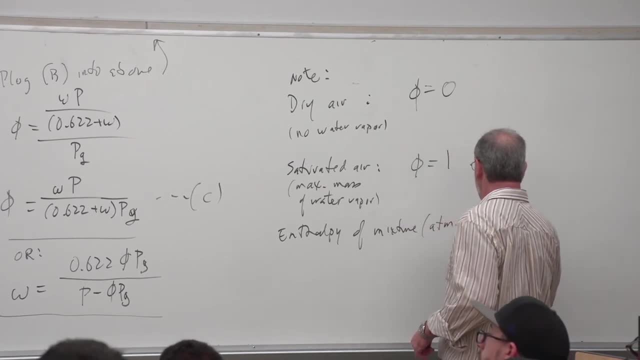 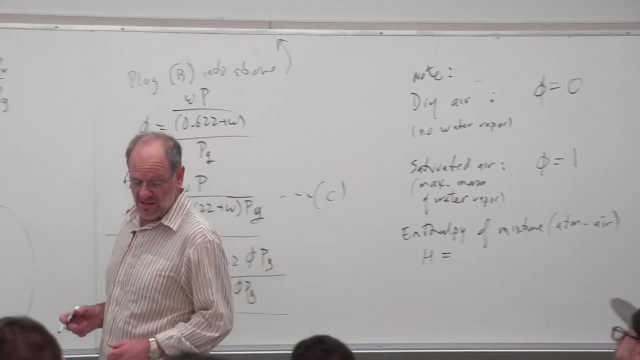 mixture. now, should I use the word mixture or should I just call it atmospheric air? It's the same thing, right? But we would note that the enthalpy of the atmospheric air is just going to be the sum of the enthalpy of the two. 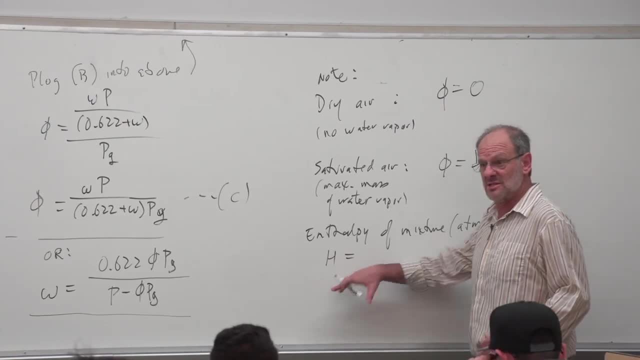 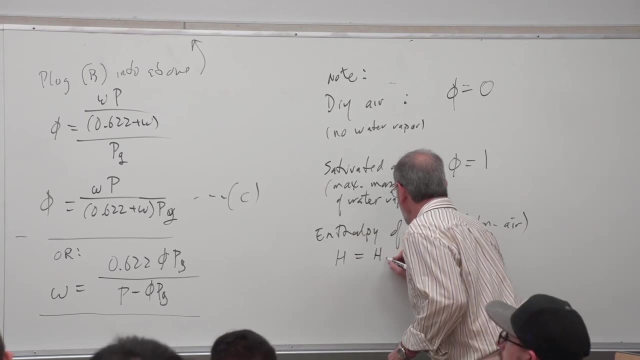 components. okay, And note, this is a total of the total air vapor mixture. So this is the total enthalpy. This is a extensive property. So for mixtures, as we saw last time, it's just the sum of the total enthalpy of each component. So 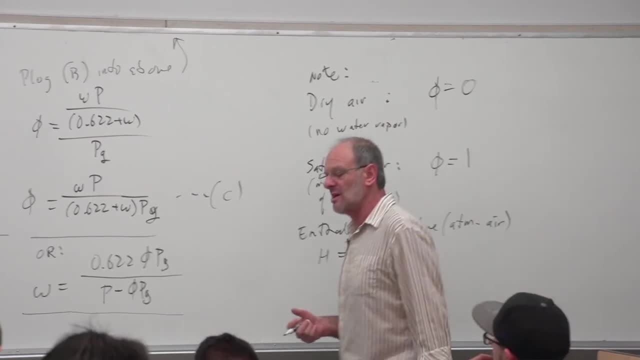 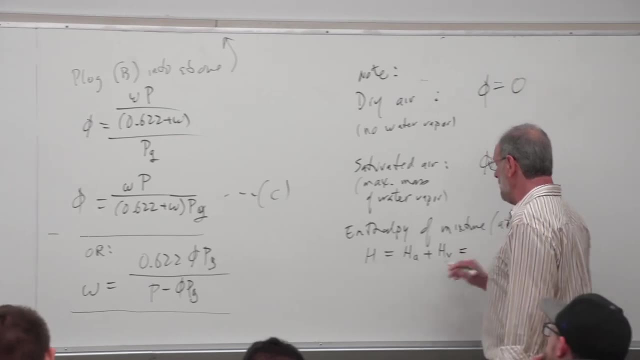 we'll just write this as HA plus HV. Again, we recognize that A represents the dry air and V represents the water vapor. Then I just want to note that the enthalpy of the dry air is just the mass of the dry air multiplied by the 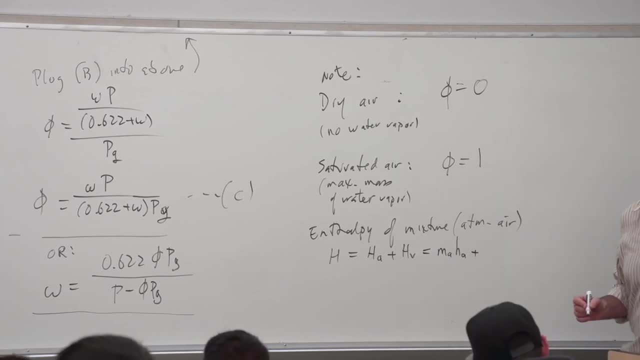 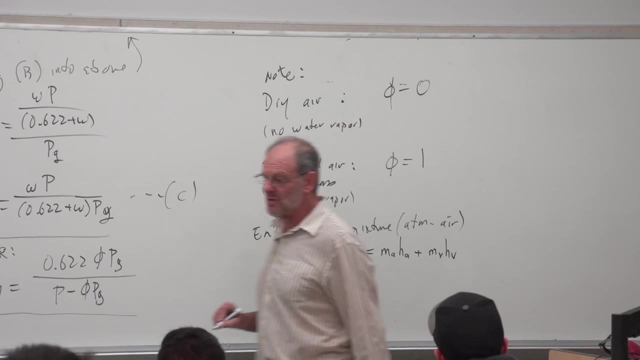 enthalpy per unit mass, In other words the specific enthalpy of the dry air. So the specific enthalpy of the dry air And then same for the water vapor. It's just the mass of the water vapor times the specific enthalpy of the water vapor. 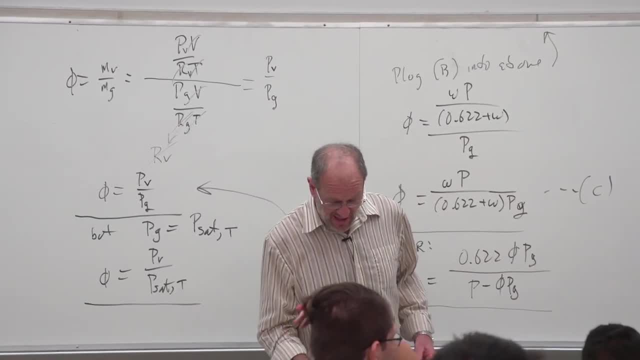 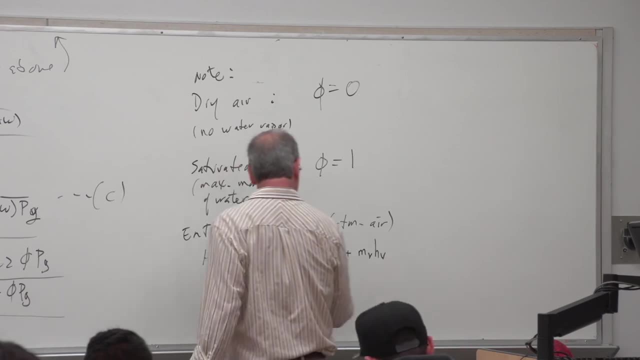 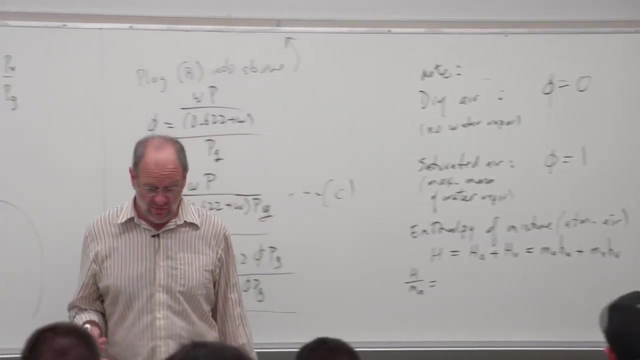 Again, enthalpy per unit mass. So we have that equation And then what we typically do is we divide out the MA term. So we would note that if we divide out the MA, so H over MA, well we're just going to use lowercase H for this. 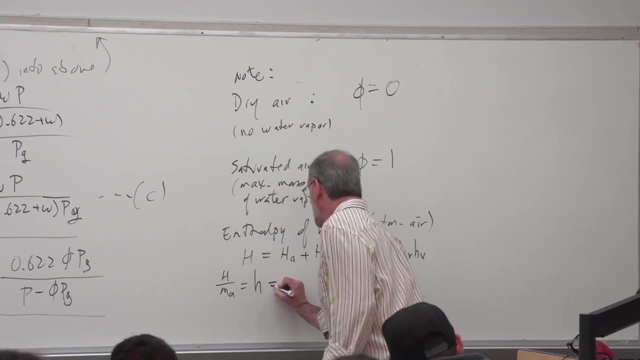 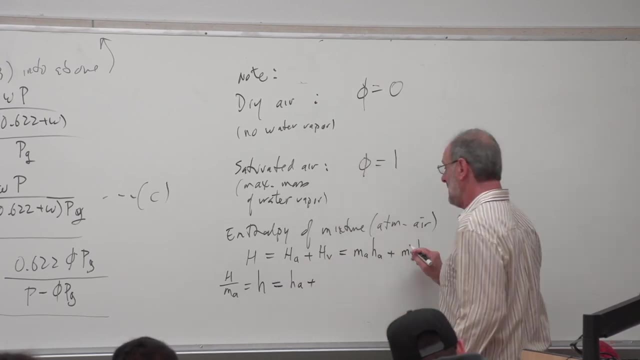 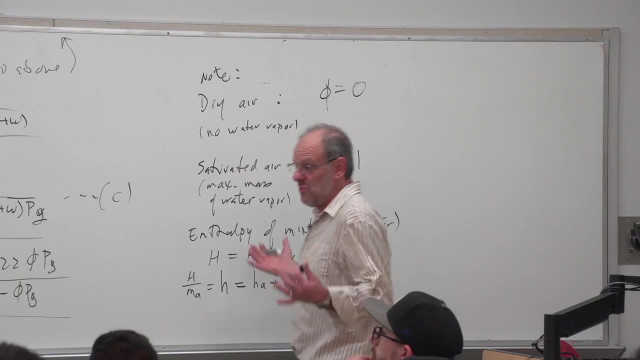 And this is going to now equal. well, again, I've divided out the MA, So this is just HA plus, And then MV over MA, times HV, And, of course, MV over MA. well, that's our definition of our absolute humidity. So I'm just going to replace: 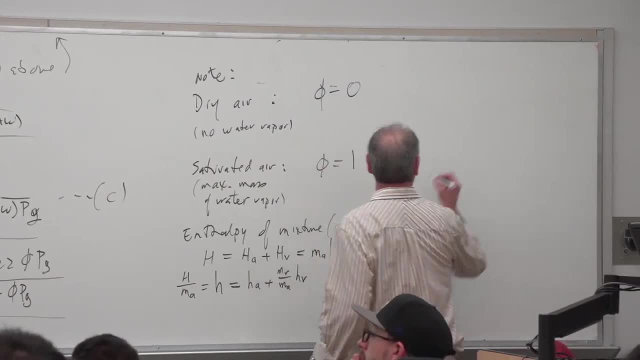 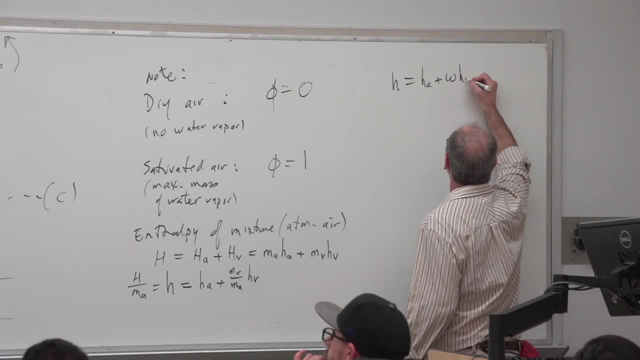 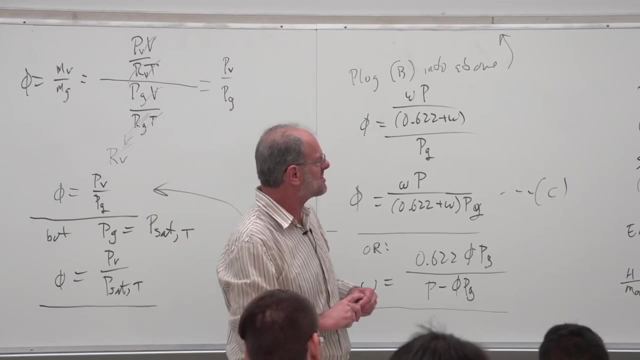 just going to use lowercase H for this, And then we're just going to use lowercase H, So it's going to be just HA plus omega times HV. Okay, Now we do have to be really careful with this particular enthalpy term. We might notice that, yes, it. 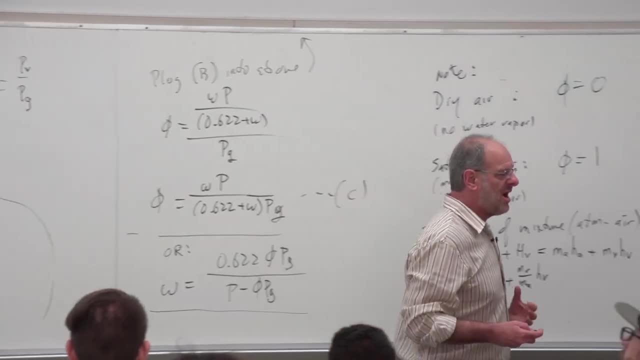 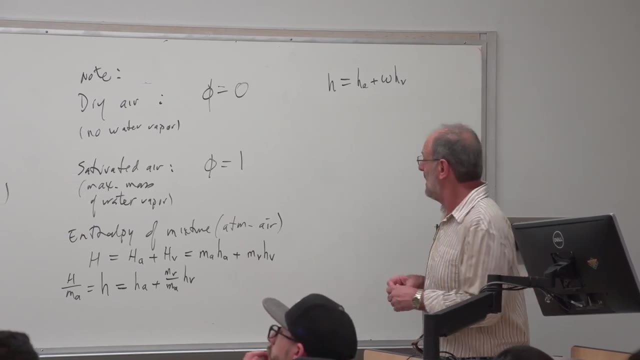 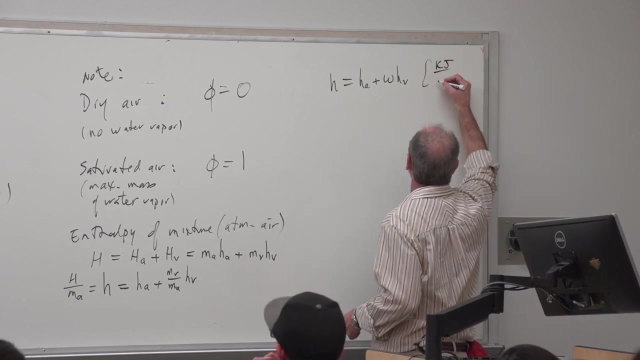 is a specific enthalpy, but the units are not energy per unit mass of the atmospheric air. that is the air-water vapor mixture. right, I'm divided by the air mass. So the units on this term are actually energy units, say kilojoules. 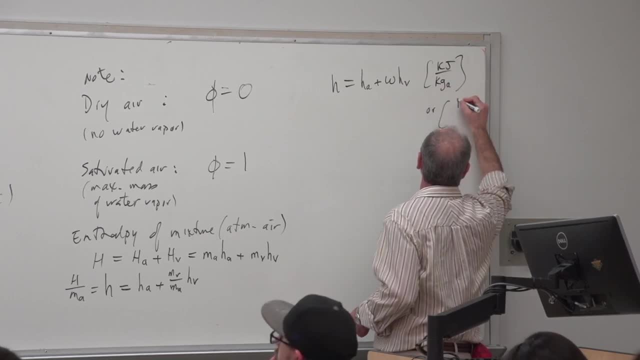 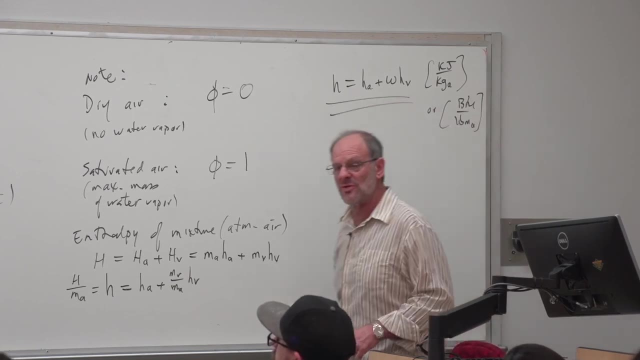 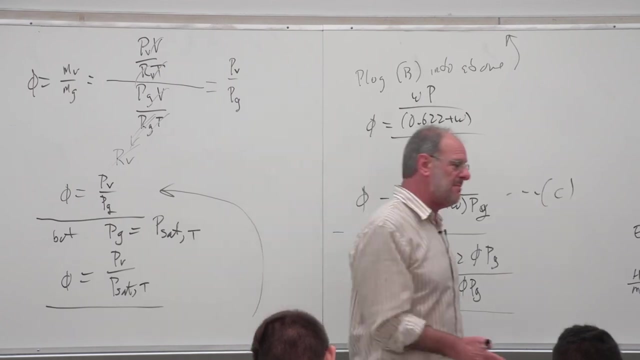 and then per kilogram of air right, Or it could be BTUs per pound mass of the dry air. So we do have to be particularly careful with the units as we're solving this type of problem. OK, Now, this is customary. I suppose that maybe. 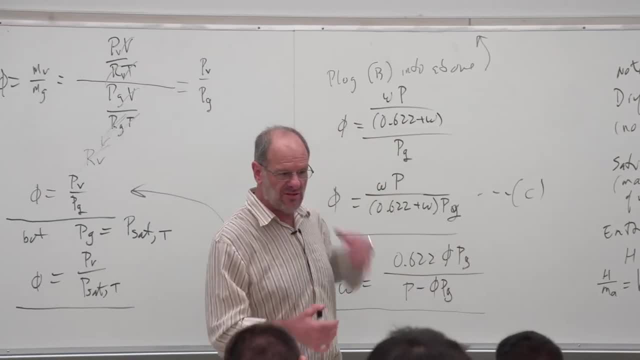 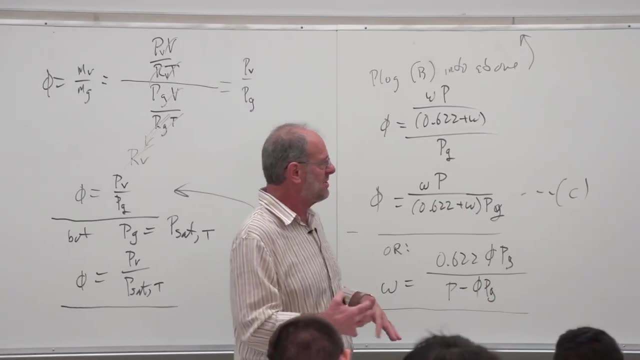 some people that study or work in thermodynamics have their own set of enthalpy tables or enthalpy data for mixtures and perhaps have data on enthalpy on an energy per unit mass of the mixture basis. But that's not customary, That's not. 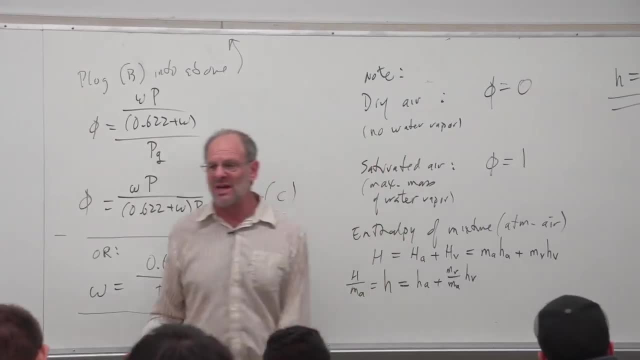 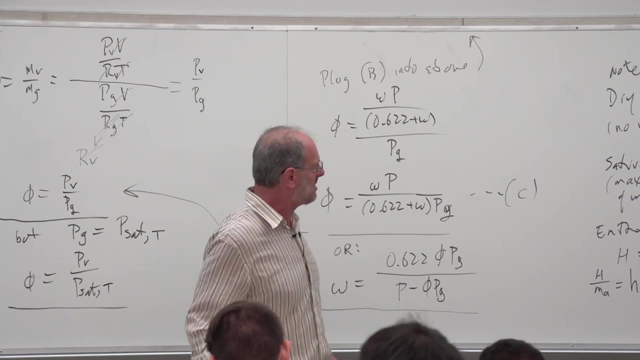 what we're going to do. It's not what's done in your textbook. All the data is per unit mass of dry air, So this is how we're going to find enthalpy in this particular class. Now there is another thing that should be noted here. Keep in. 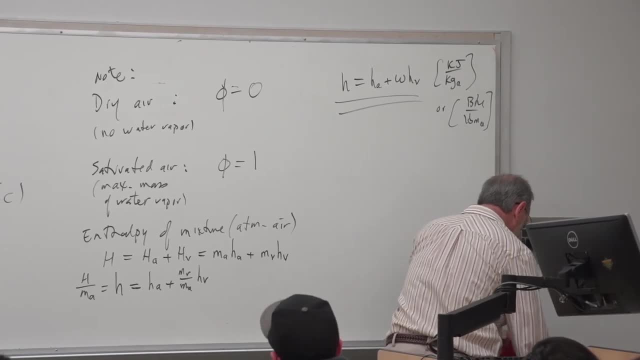 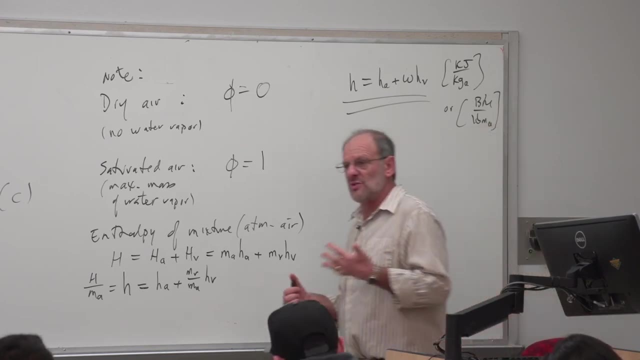 mind that the enthalpy, as we're treating both components of our atmospheric air as an ideal gas with constant specific heat, we should recall that enthalpy is only a function, at least for ideal gases, right, It's only a function of 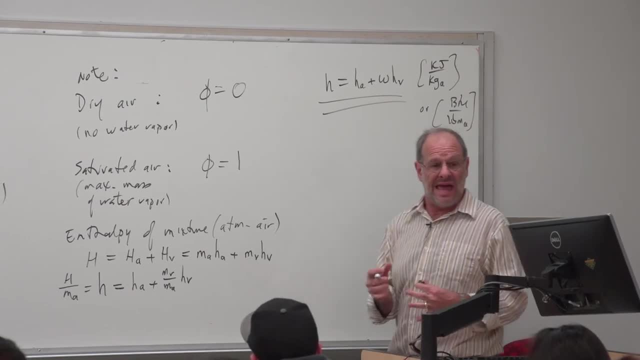 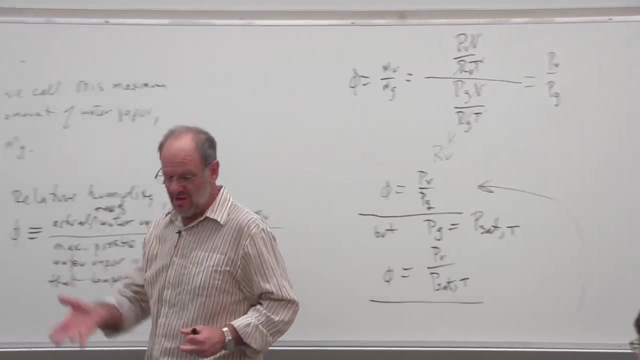 temperature. It doesn't matter, actually, how much water vapor is in the air, right? It doesn't matter what the partial pressure of the water vapor is. Certainly we can add water vapor into the air all the way up to saturation And, yes, that will certainly affect the partial pressure of the water vapor, right? 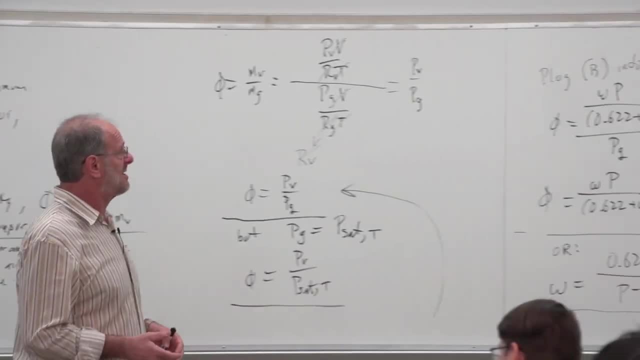 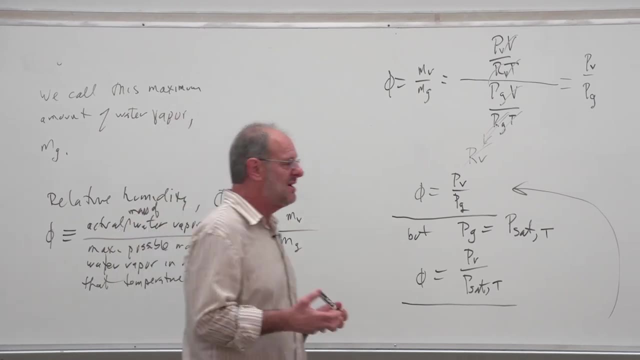 The more water, the more partial pressure, But pressure doesn't. I'm sorry, but enthalpy data doesn't depend on pressure, right? It's only a function of the pressure. So it's only a function of the pressure. So it's only a function of the. 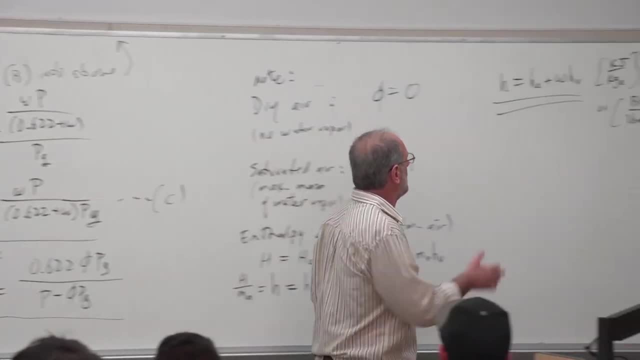 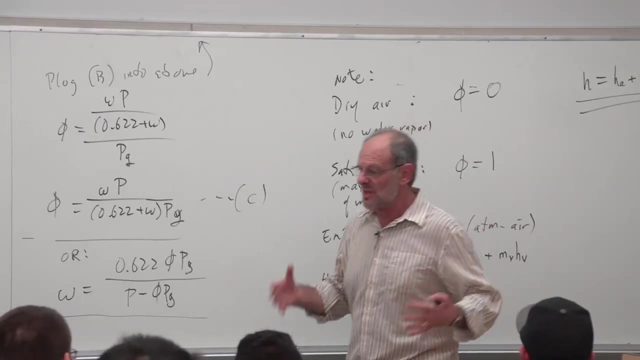 temperature. So we might note that HV, while it certainly will vary depending upon the partial pressure, it's always going to have the same value, regardless of the amount of water vapor in the air. And again, it's only going to be a function. 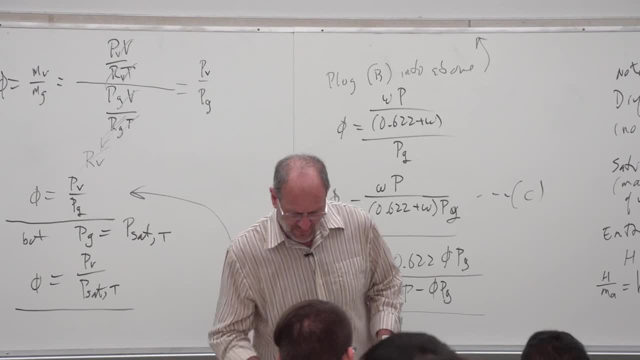 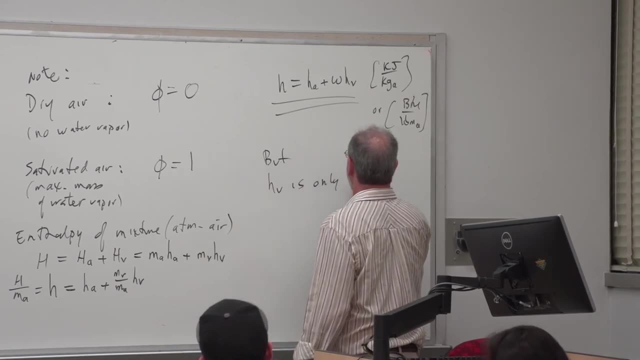 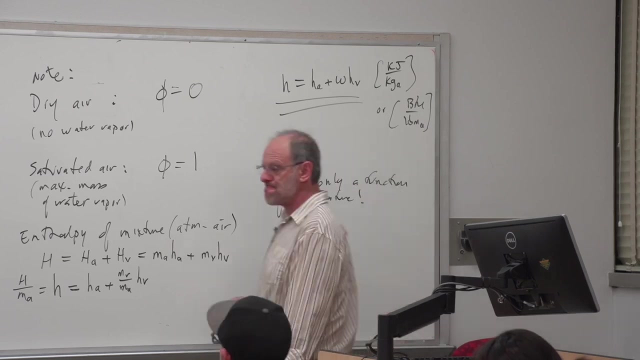 of that particular temperature. So HV is only a function of the partial pressure. So HV is only a function of the partial pressure. So HV is only a function of temperature. OK, Again, we know this for an ideal gas. So how does that affect? 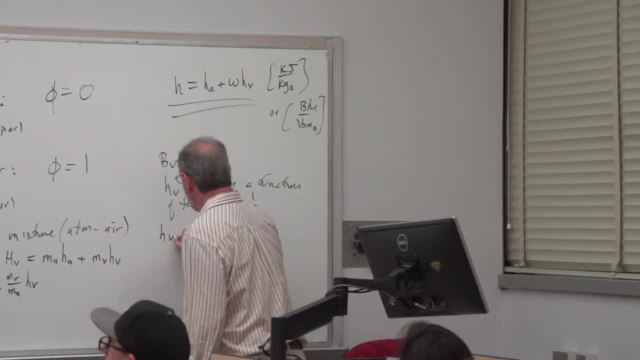 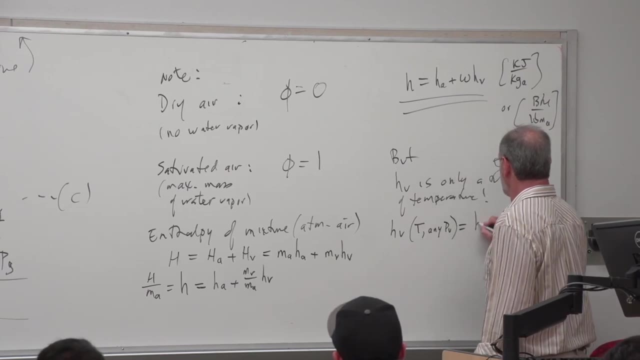 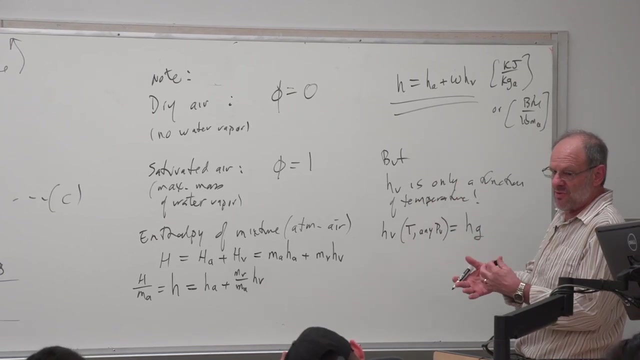 us Well, HV at a particular temperature and at any partial pressure. well, this is just going to equal HG, right, The enthalpy of the saturated vapor. I mean it's a vapor, It's going to be the same, whether it's a saturated vapor or it's. 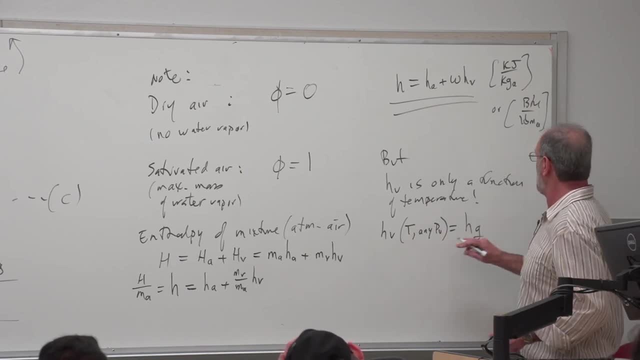 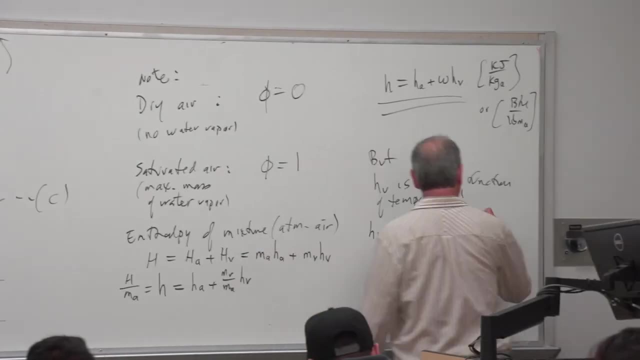 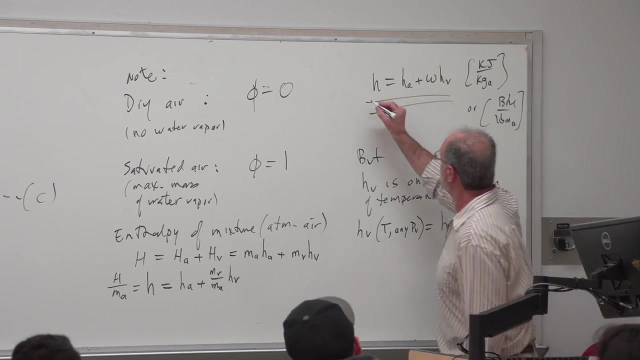 not a saturated vapor. If it's something much less, it doesn't matter. It's just doesn't really matter. So this is just going to equal HG at that particular temperature. OK, So with this in mind, let's just modify our equation above. So 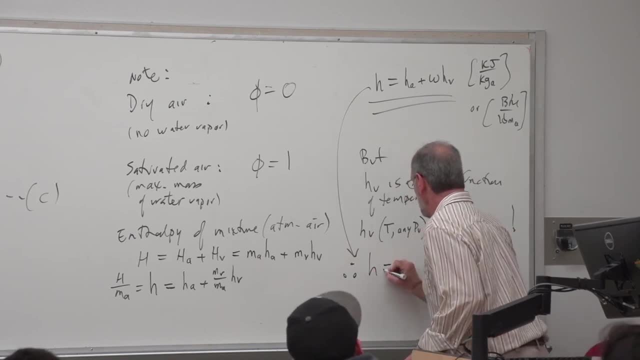 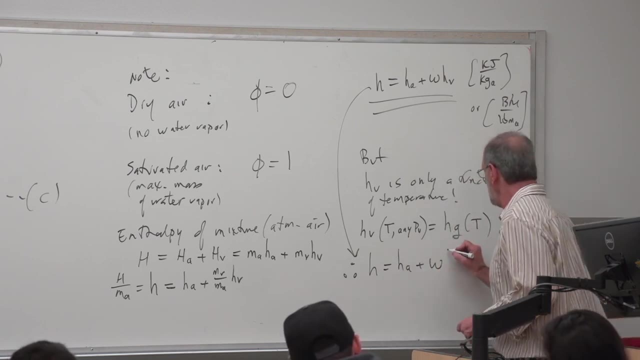 therefore, we will just say that the enthalpy of the mixture is the enthalpy of the dry air plus omega, and then times the enthalpy of saturation. HG, Really, I say enthalpy of a saturated vapor at the given temperature. OK, So this is the 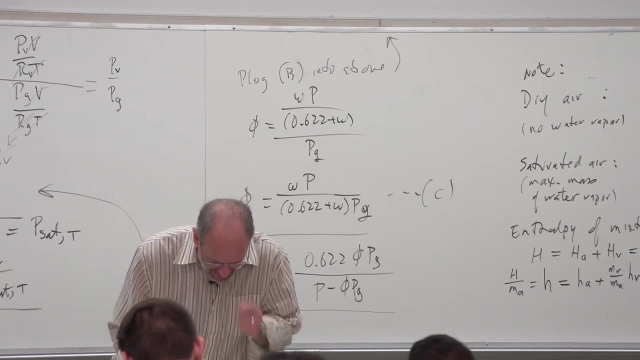 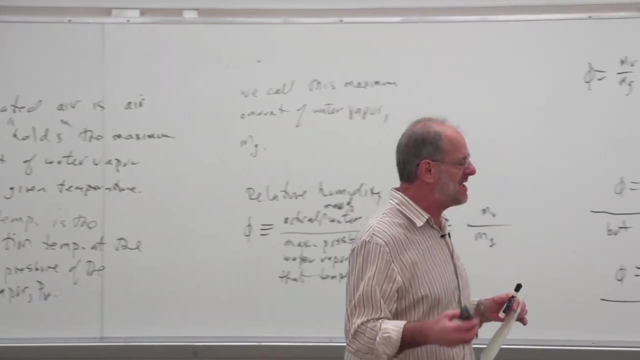 equation that we're going to use as we find our enthalpy data. Now we would be able to find all of our enthalpy data in the tables. In fact, maybe I shouldn't say we would. We can find all of our enthalpy data in the tables, But we're 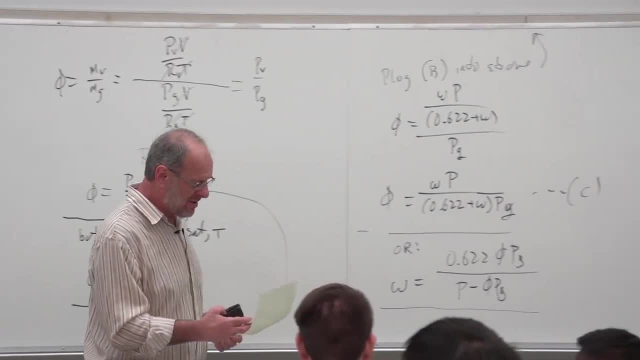 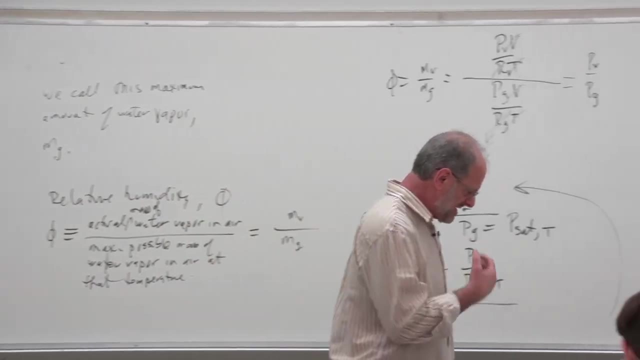 going to have to be really careful the way we're going to do this. We're going to use the tables And here's our little bit of a problem. OK, If we look into our thermodynamic property tables, the reference state for water vapor is not. 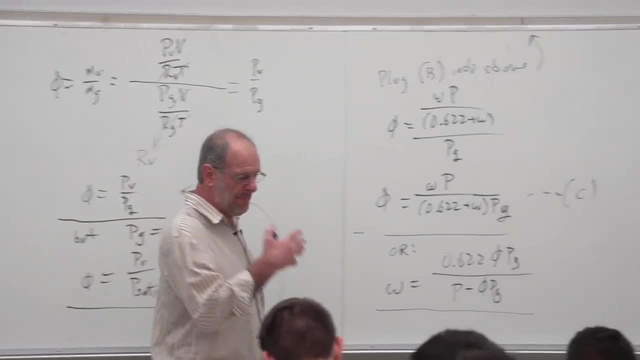 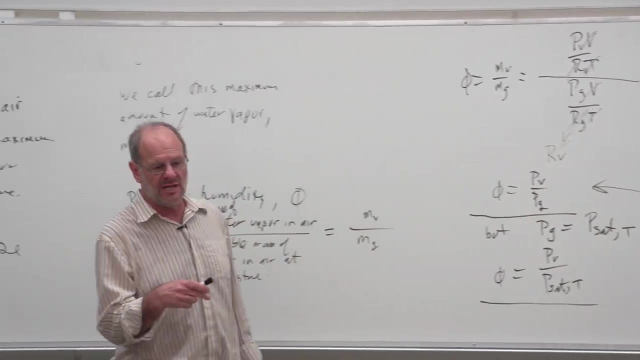 the same as a reference state for the dry air. You may recall way back in ME301, hopefully whoever you had for 301 discussed this- But if you're using data like enthalpy data in one equation for more than one component, you need to make sure. 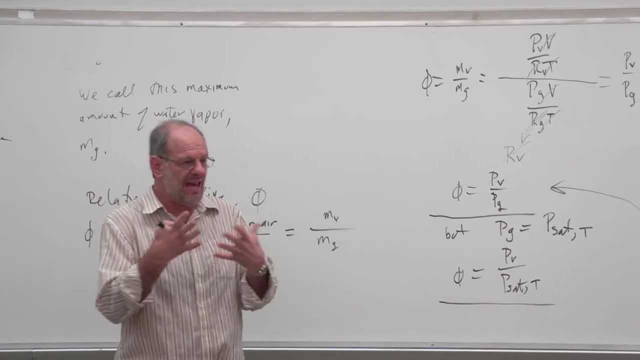 that the reference frame, the reference state, if you will, is the same as the reference state, if you will, for that enthalpy data is the same for each of those components. It's not the same in our book. OK, If we look at the table. 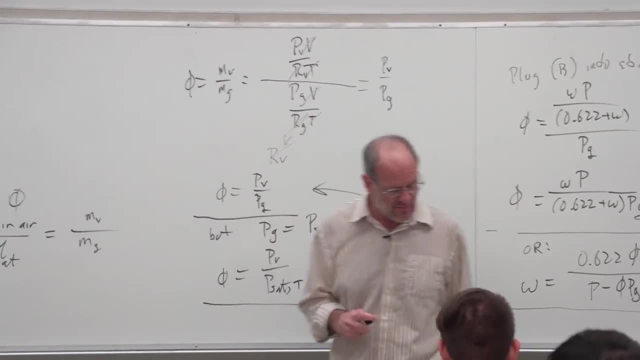 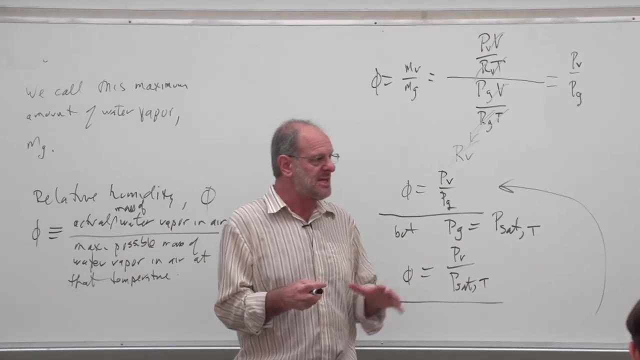 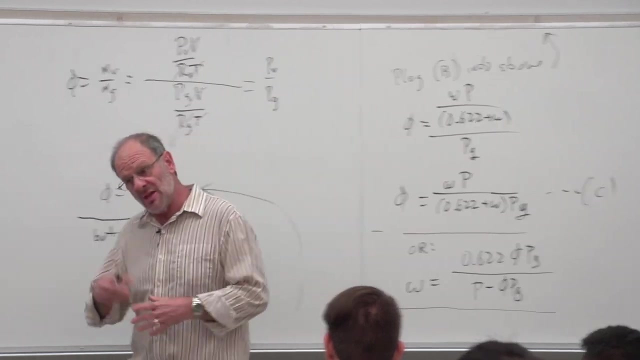 well, we're talking about water vapor here. So if we look into the table- let's say A4, A5, like that- those are water data And that has a value. of H equals zero for a saturated liquid at zero degrees Celsius. On the other hand, if we 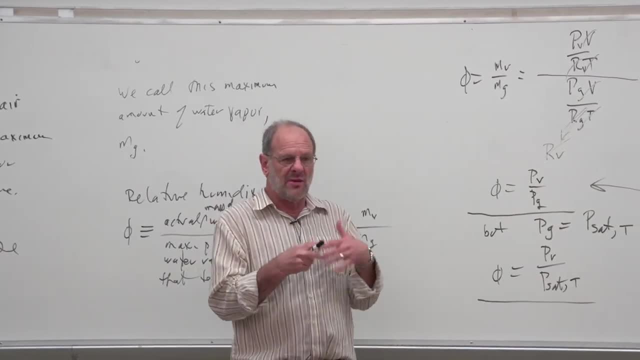 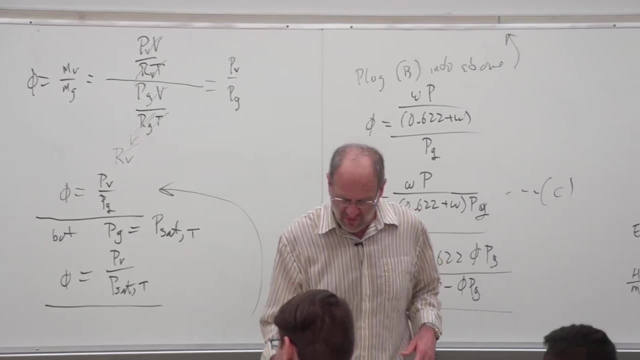 look at the enthalpy data for air, the reference frame is the same for air. So the reference frame is for H, equal to zero, at zero degrees, absolute. OK, They're different. So what we have to do is we have to recognize that and make sure that. 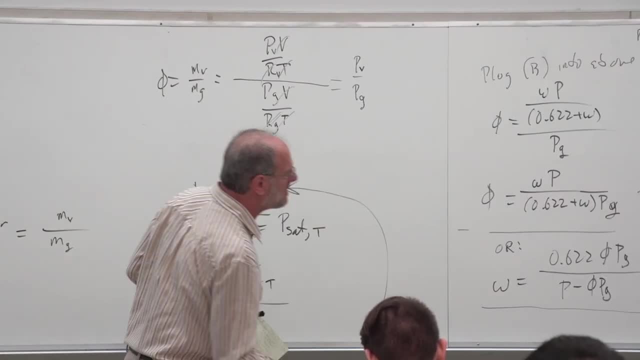 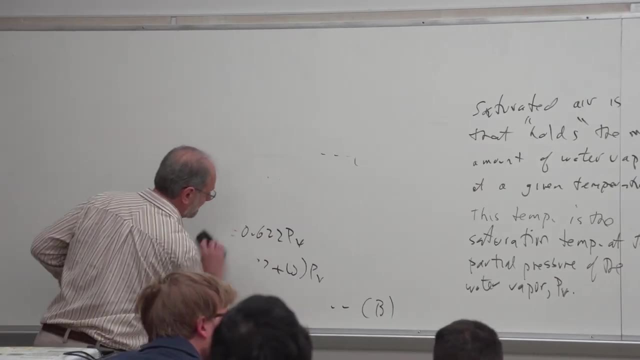 when we're using our enthalpy data in this one particular equation, that we modify it appropriately so that each of our enthalpy terms have the same reference state. OK, So the way we do it typically is this: We assume that the 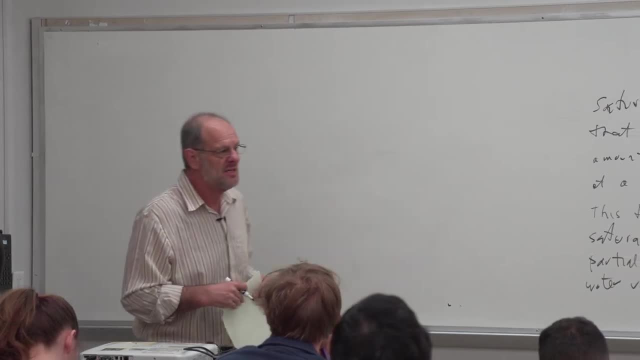 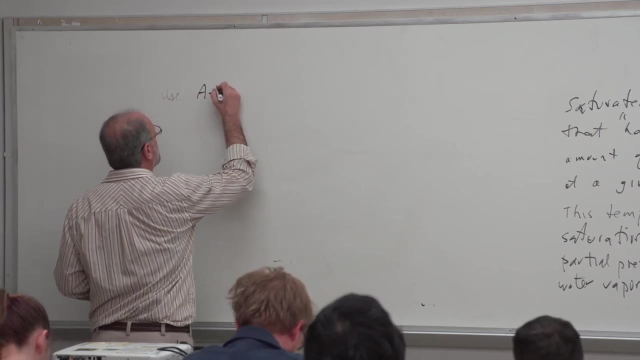 reference state in our water tables- table A4,, 5,, 6, is the same as the reference state in our water table, So that's going to be the one we're going to use. So we're going to use. well, we're talking about saturation data, right? So we're. 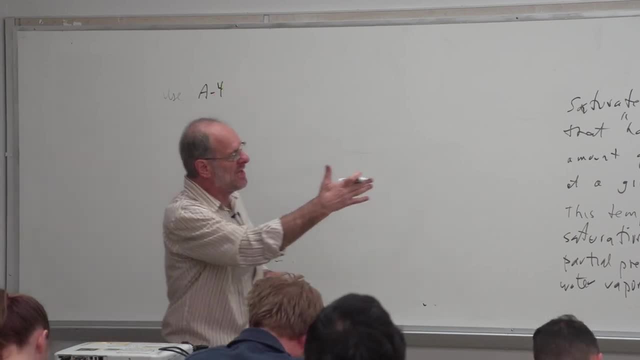 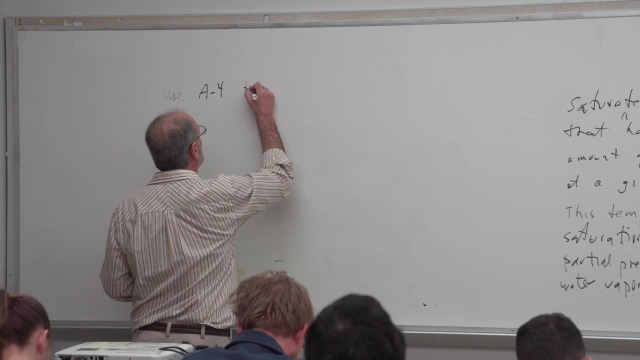 typically talking about A4.. Remember, we're going to need HG, We're going to need the enthalpy of the saturated vapor at a particular temperature. So A4 is our temperature table. So we're going to use A4 in order to find HG. OK, And 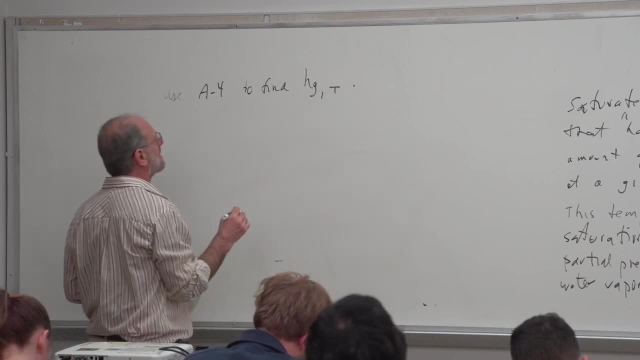 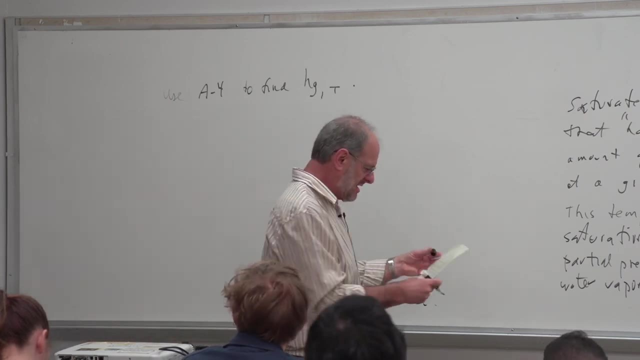 this would be at whatever the particular temperature is OK, And that's going to be HG. That means we're going to have to do something different for the dry air component, And we'll get to that in just a moment. OK, So for right now, let. 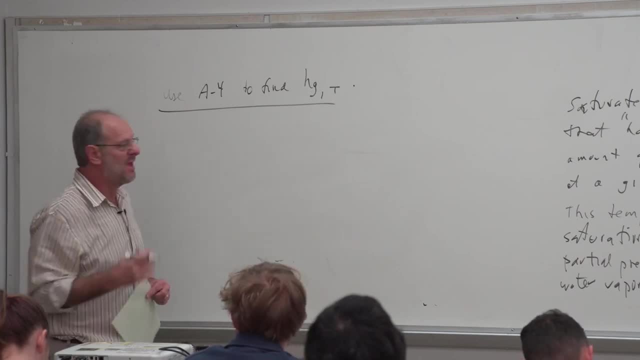 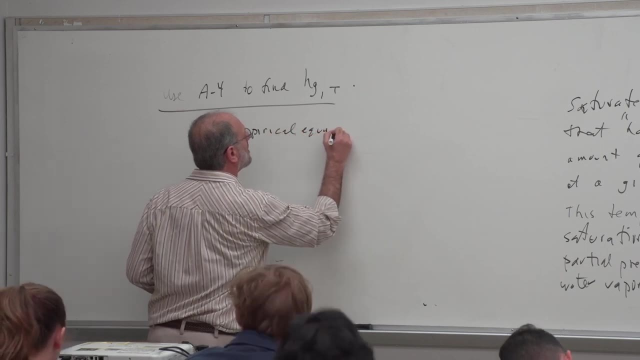 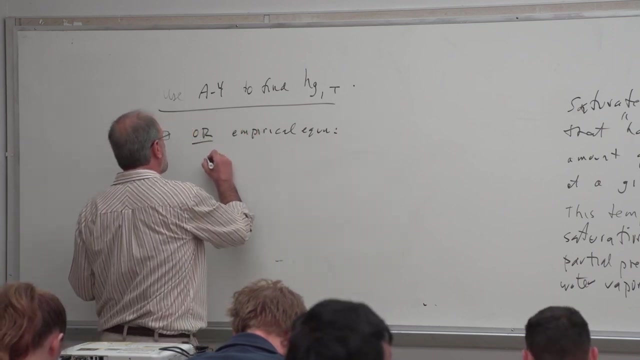 me first note that this is what we could use. However, there is an empirical relationship that's presented in the textbook. I believe it's equation 14.4 and 14.5.. It says HG is equal to 2500.9.. So we're going to have to do something. 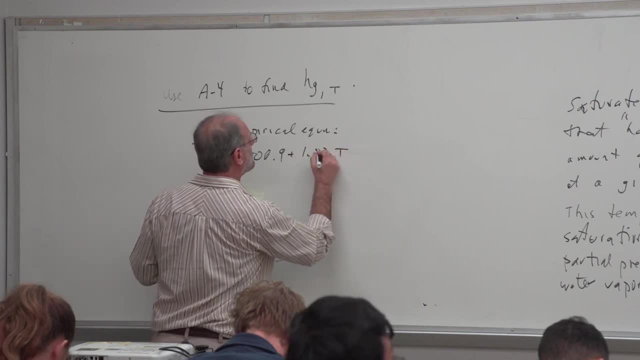 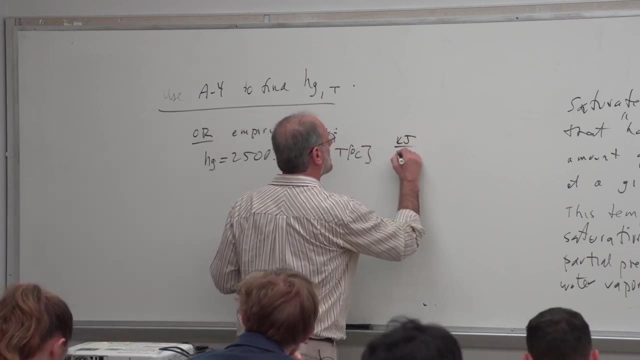 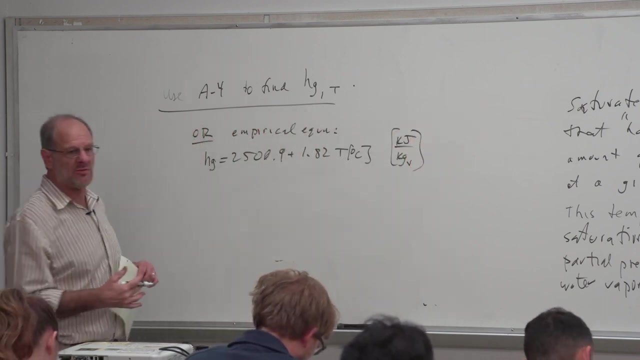 different: 2500.9 plus 1.82 times the temperature, And this temperature has to be in degrees Celsius. This is going to give you enthalpy on a kilojoules per kilogram of water vapor basis. Please note that as an empirical relationship it 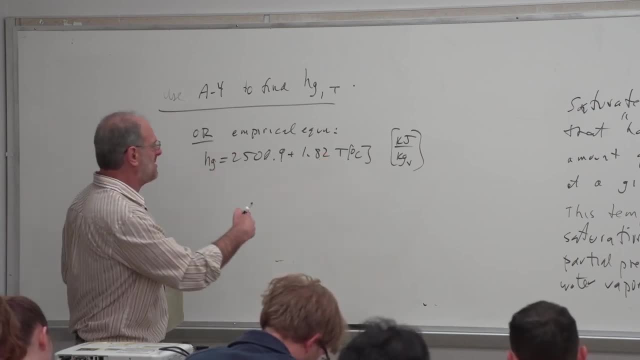 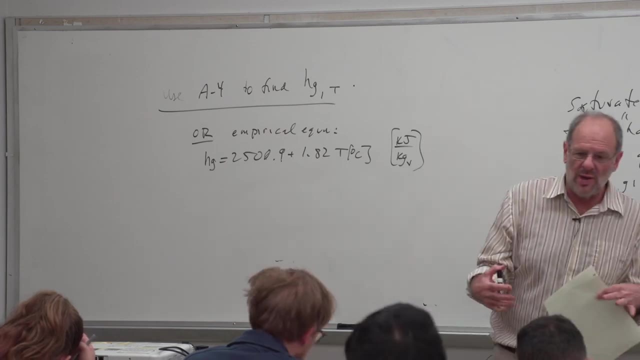 is a function of temperature in the appropriate degrees for that relationship, And it has to be in degrees Celsius. So I know that previously we've talked about how any time you use temperature within an equation, you're going to have to use the absolute temperature scale right, Rankine or Kelvin. This is an 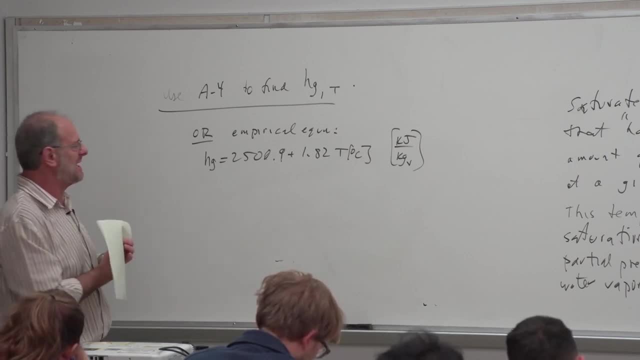 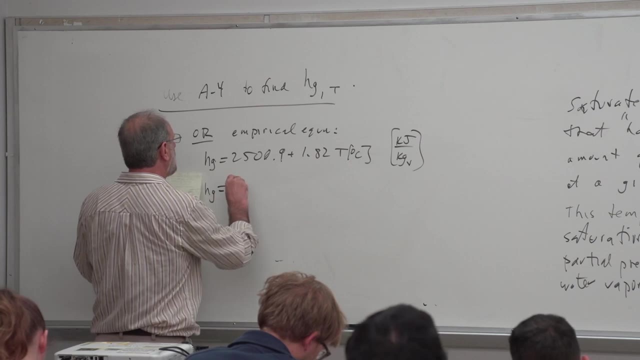 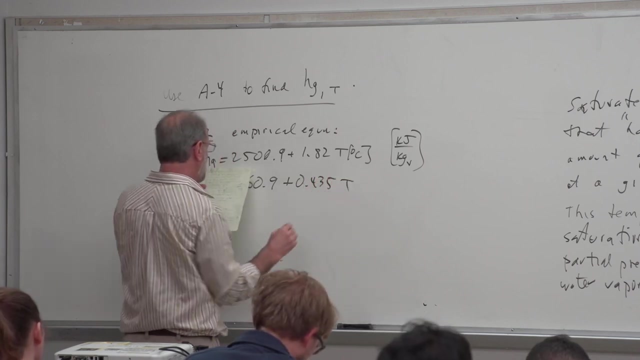 exception right. This is because of the nature of this particular data. So this is what we use in the SI system. In the British system, if we chose to use this equation instead of the tables, it's 1060.9 plus 0.435 times the temperature. 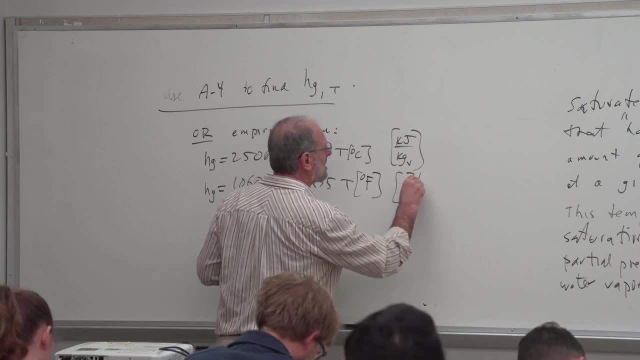 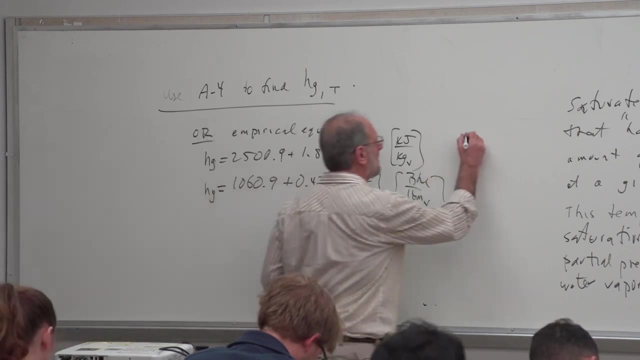 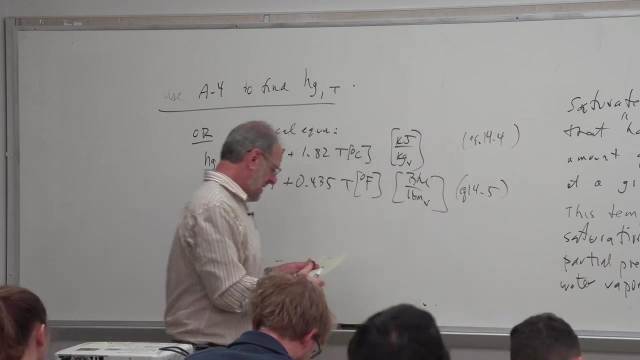 And this temperature is going to be in Fahrenheit, And this will give you BTUs per pound mass of water vapor. Okay, So either one. we want Equation 14.4 and 14.5.. So this is where you're going to find those in the book. All right, So if this is what we do for the 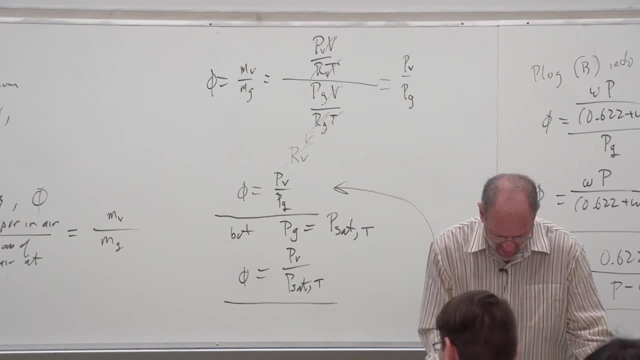 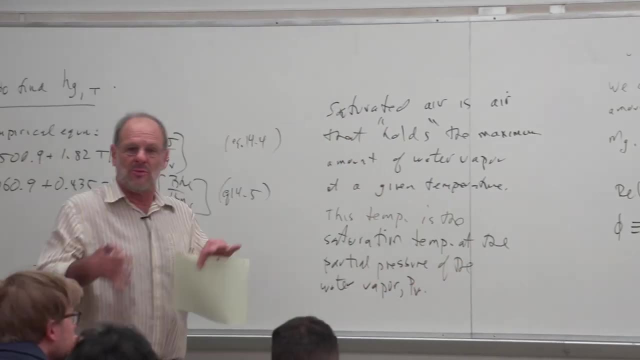 water vapor. what do we do for our dry air component? Well, we do have air tables on our book, right, We've seen them, They're table A17. But again, we can't use them. right, The air tables A17 and A17.. So we can't use them, right, The air. 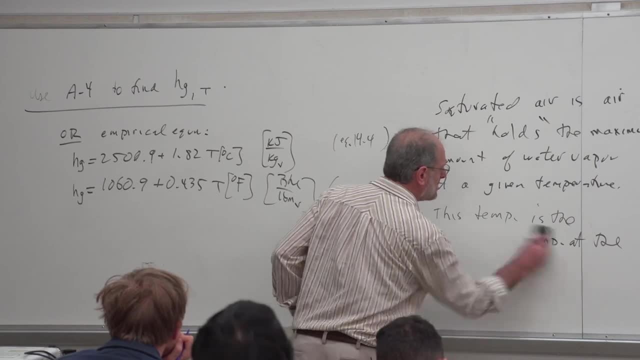 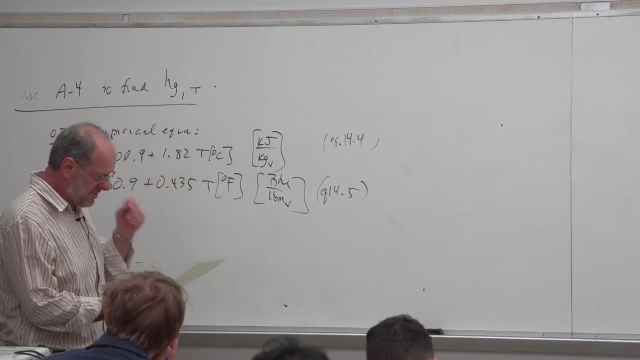 tables A17 have a different reference state than the water tables. So what do we do? Well, again, one would have to use some sort of an empirical relationship that deals with this, And this is also described in your textbook. So let's just 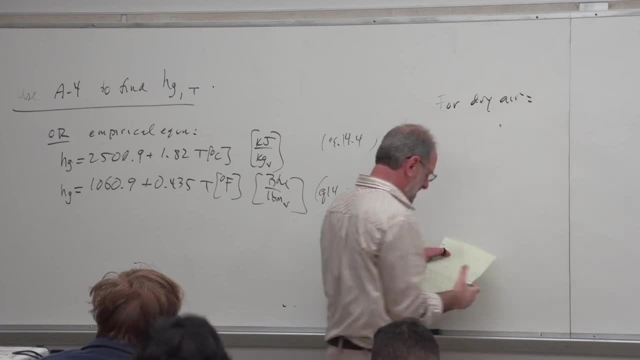 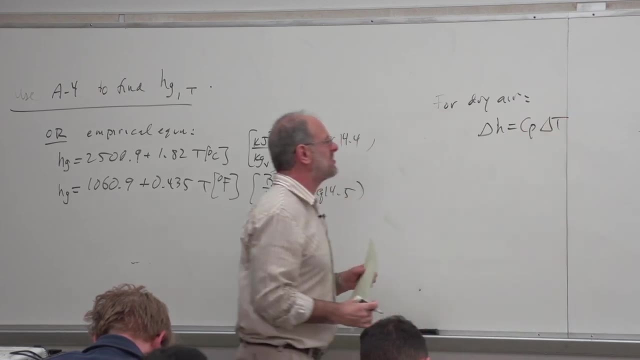 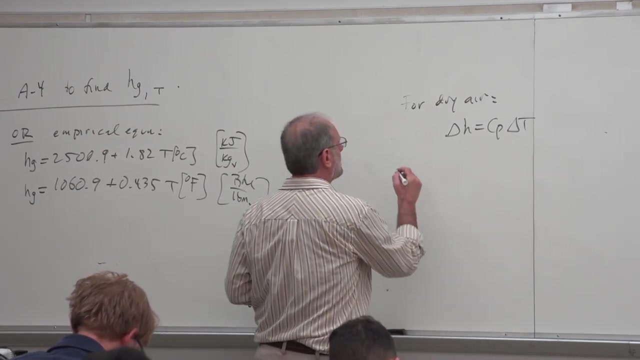 look at it this way For dry air. first, we'll note that any enthalpy change delta H is going to be CP times the temperature change. right, We know that for an ideal gas with constant, specific heats. We would also note that the enthalpy 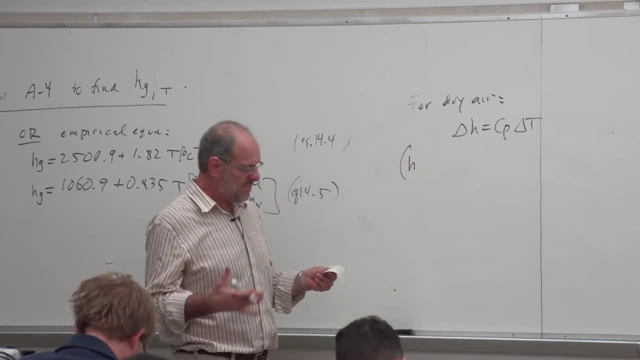 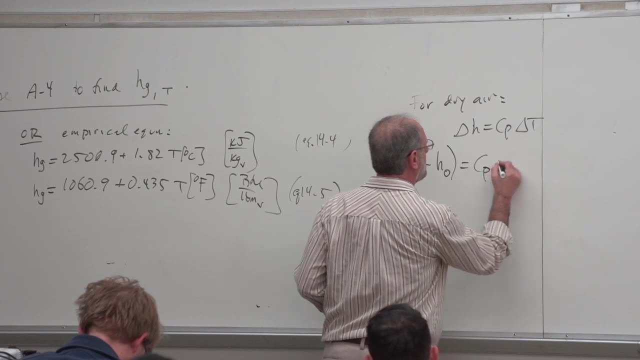 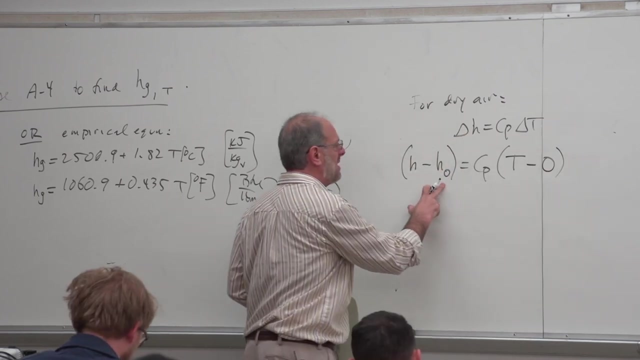 well, the change in enthalpy is just going to be the enthalpy at our particular temperature minus, let's call it the enthalpy at zero, And this will then equal CP times our particular temperature minus. well, the enthalpy at the temperature. 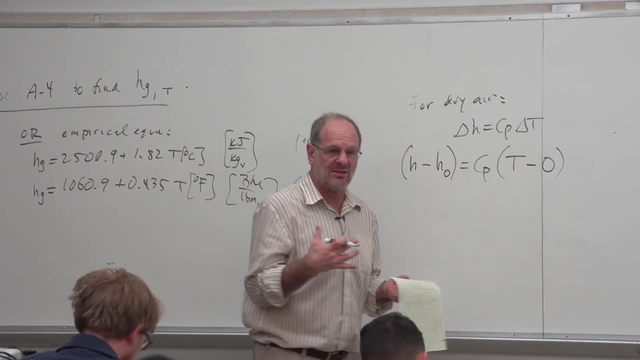 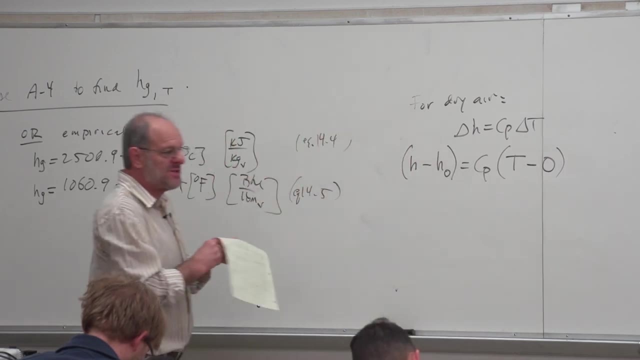 of zero And by convention, we're going to be using Celsius over the temperature or Fahrenheit again. So this equation then, well, if we use the same reference state as we did for water, the enthalpy is zero at zero degrees Celsius or zero. 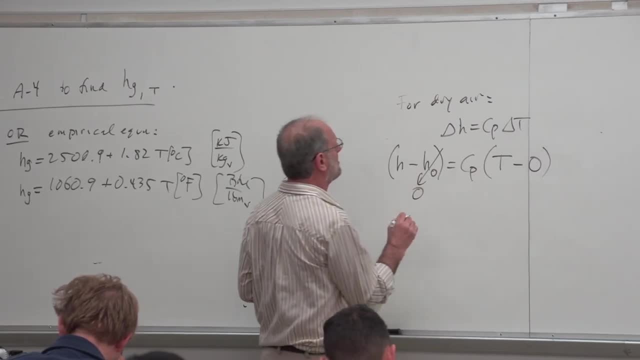 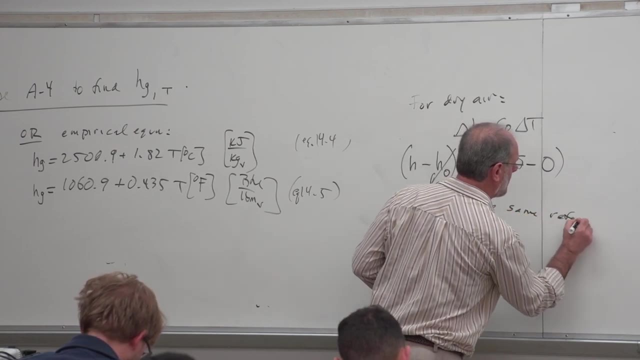 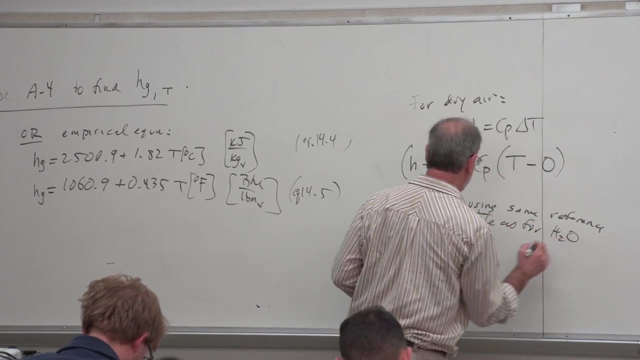 degrees Fahrenheit. So this term is going to be zero. OK, And again, note that this is using the same reference state as for water. OK, So this is going to be equal to zero. So that's equal to zero. So basically, H is just going to equal. 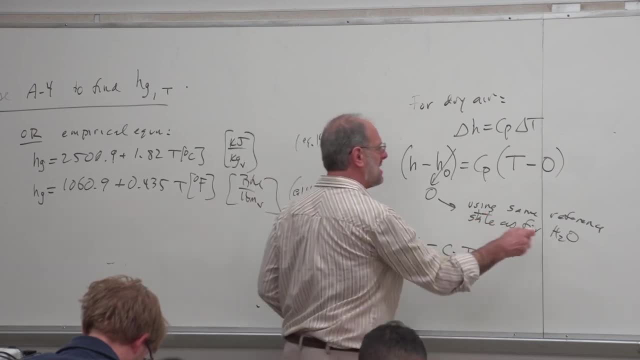 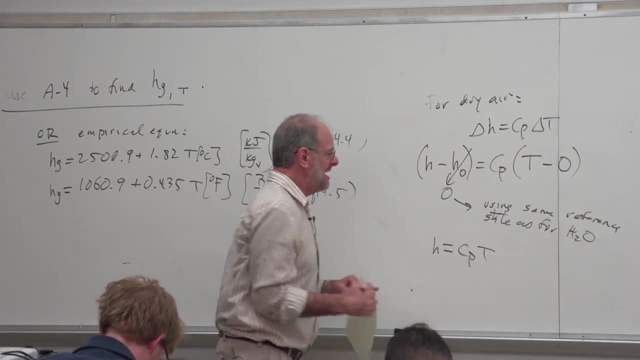 CP times T, But again, the same reference state for water assumes that H is zero at T equals zero. So this is just T And again, since we're using Celsius or Fahrenheit, this temperature again is going to be in one of those appropriate. 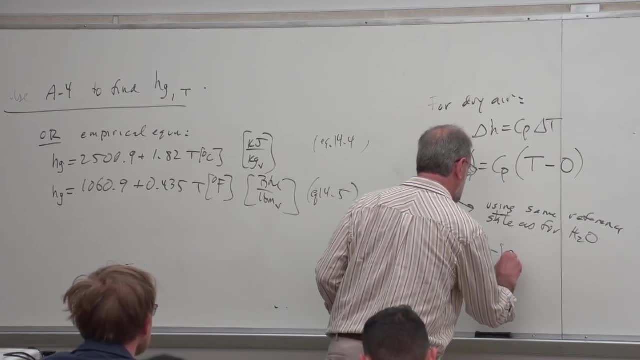 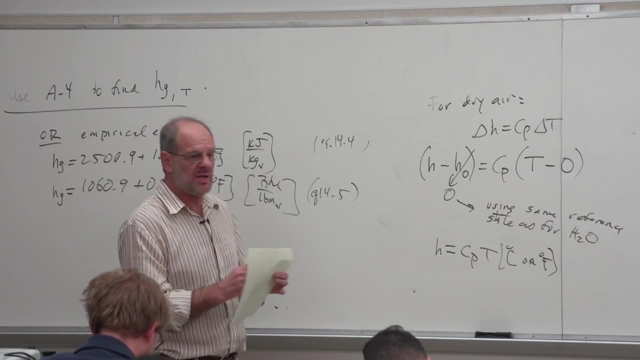 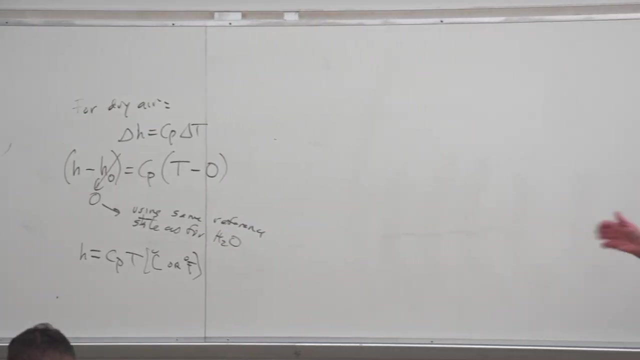 temperature scales, So this is either going to be in Celsius or in Fahrenheit. OK, So with all this in mind, all we really need to do is go into our tables and look up a value of CP, And then we'll be able to simply find the enthalpy at. 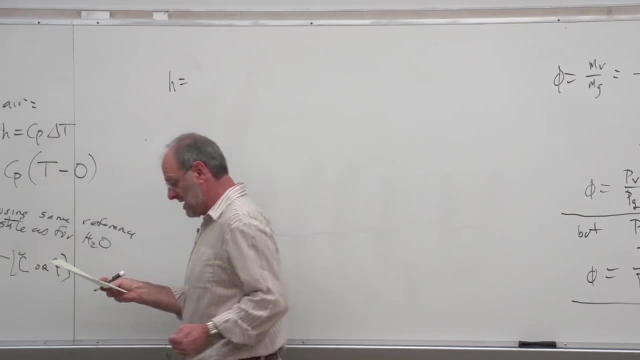 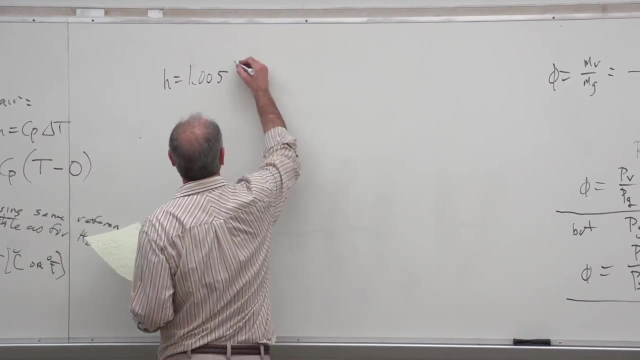 any particular temperature. So if we look first at the SI system, this is just 1.005.. That's our specific heat And that's going to be in kilojoules per kilogram, per degree C, And then times the temperature Indicates the temperature. 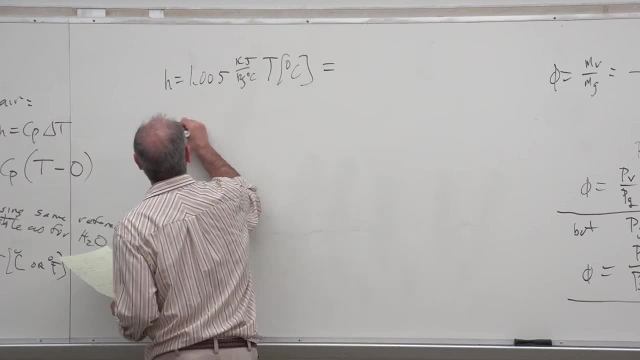 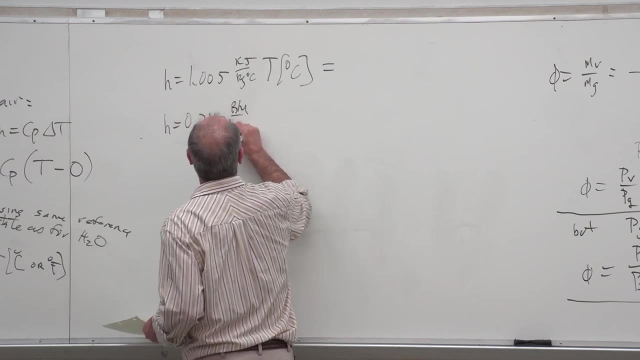 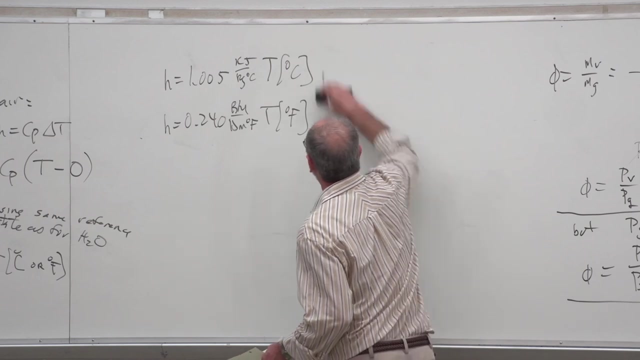 In degrees Celsius And then in the British system CP is 0.24.. So that's going to be BTUs per pound mass degree F And then times the temperature in Fahrenheit And that's going to give you the enthalpy. And let's be really. 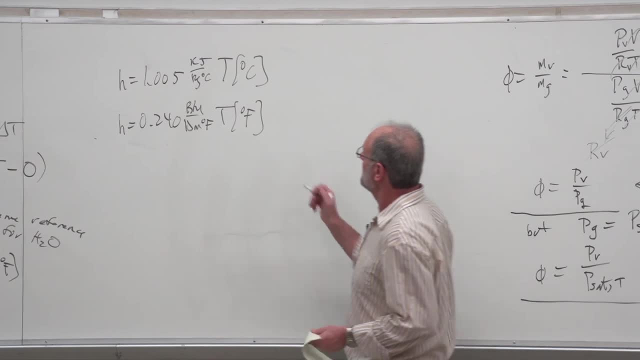 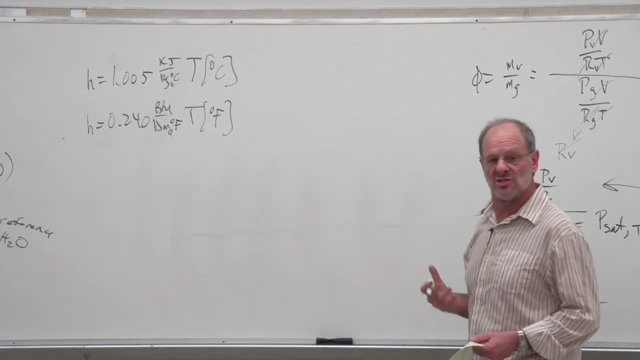 careful with the units again. right, These are air data. So this is just the dry air component. Perhaps we should put a little subscript A here on those mass terms, just to remind us that this is just for the dry air. So this is going to. 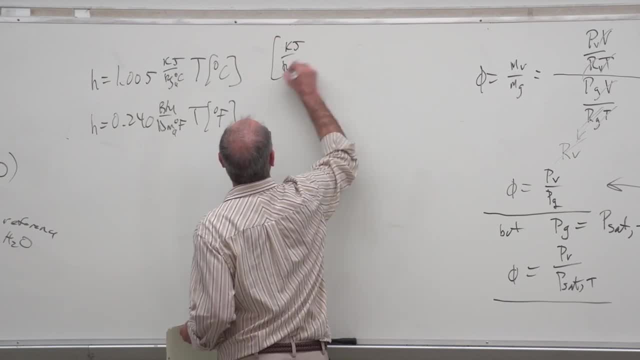 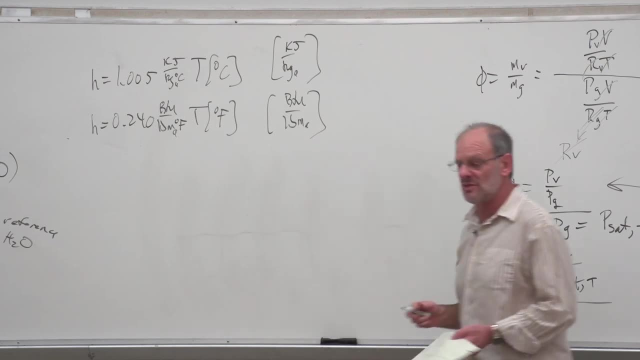 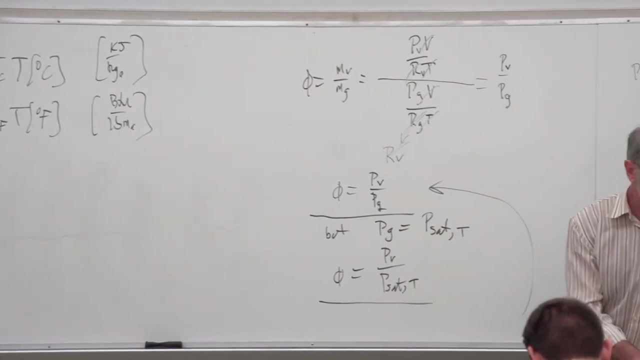 be in kilojoules per kilogram of dry air if we use the upper equation, Or BTUs per pound mass of dry air. if we use a lower equation, Again, though, we need to use Celsius or temperature data in order to get these particular enthalpy terms. 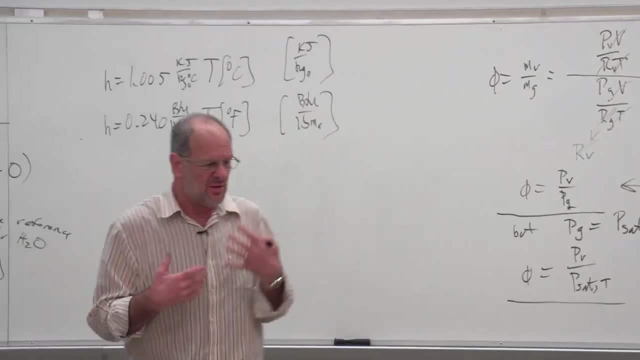 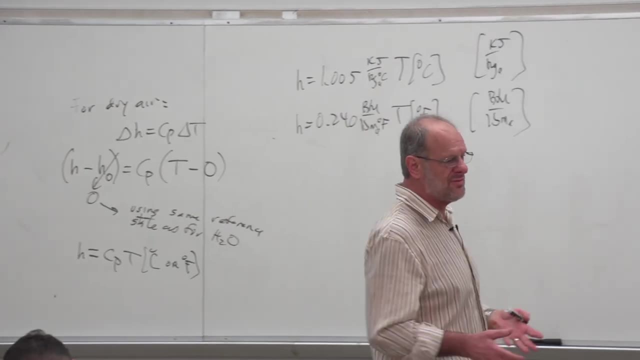 So I know that we really haven't talked much about this whole thing, but I do think this whole idea of reference frames and you know how all of our enthalpy or internal energy data is actually given relative to a reference frame- I mean, if you look in your book it does discuss it, way back in chapter I. 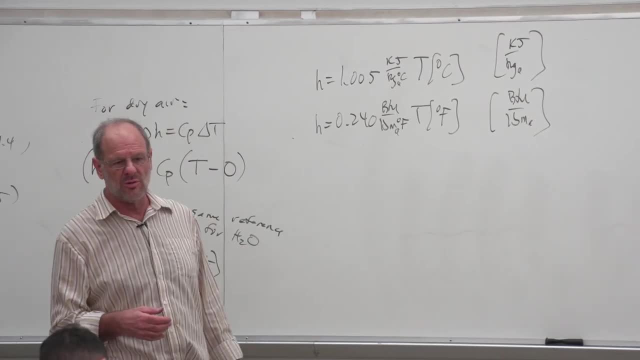 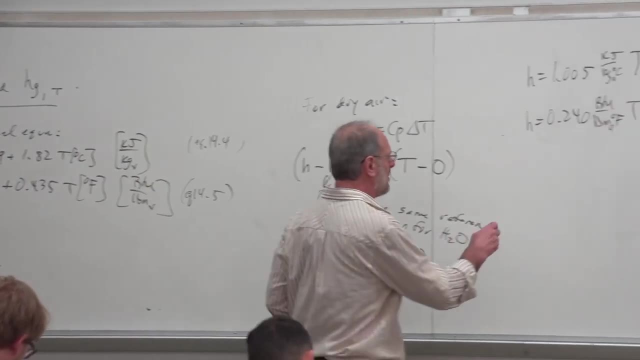 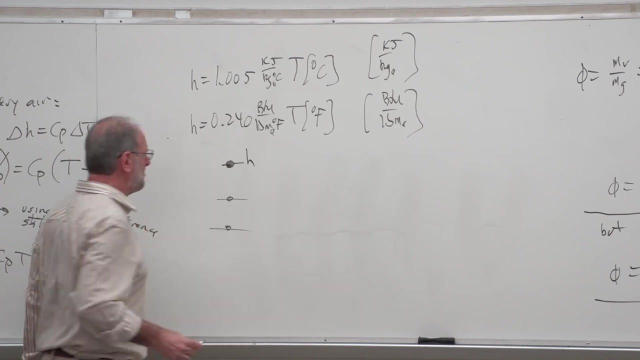 guess it's chapter three where you're first being exposed to these property tables, But nonetheless you'll just have to essentially accept this, that the reference frames are a little bit different. I mean, maybe one way to think about it is, you know, let's say this is my thermodynamic state point. 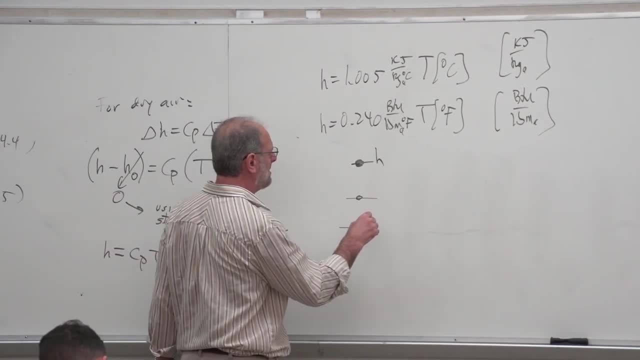 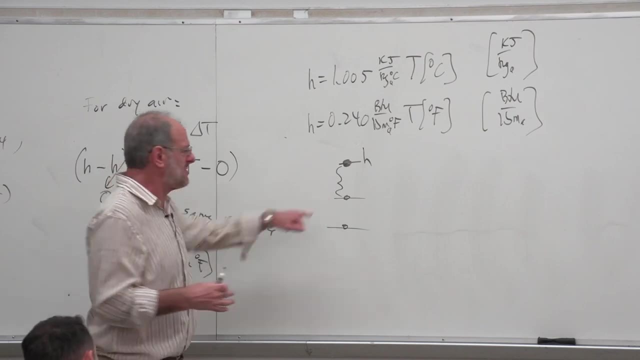 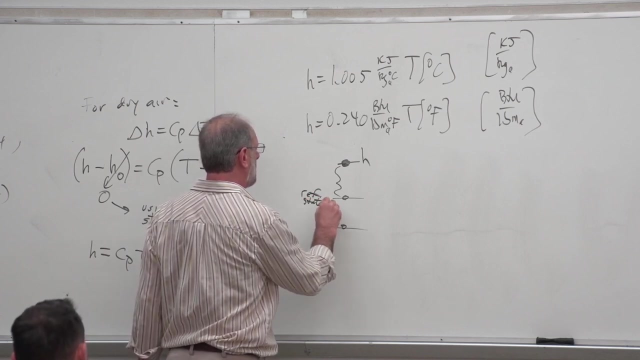 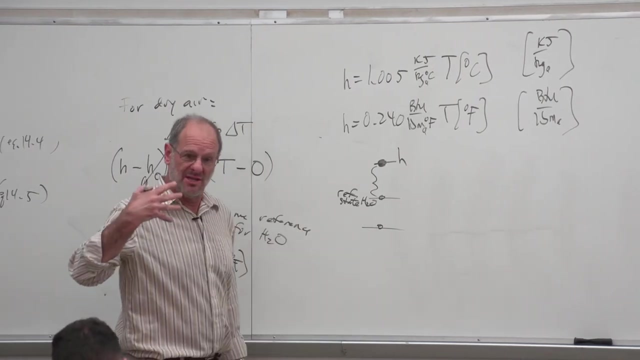 representing H, If we have data for water, water's already with reference to zero degrees Celsius or zero degrees Fahrenheit. So this would be the reference state for the water, But the reference state for the air as presented in the textbook- I'm sorry- the reference state for the dry air as described in the textbook would be. 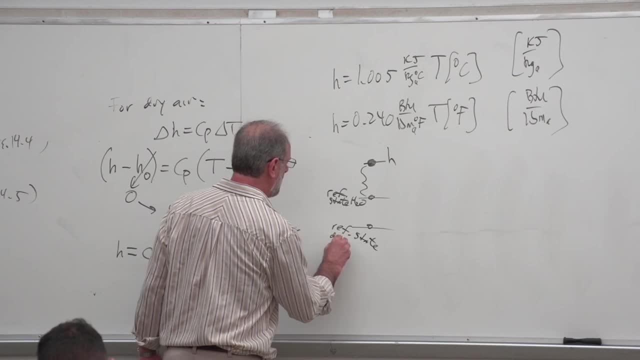 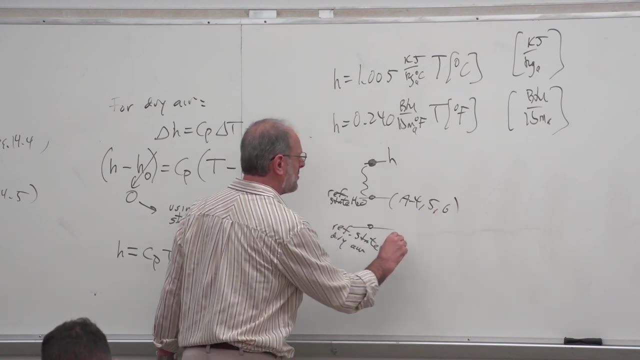 down here. This is a reference state For dry air. Now this reference state for water, you know, is for tables A4, A5, A6.. This reference state for dry air is really the data that's in table A17.. 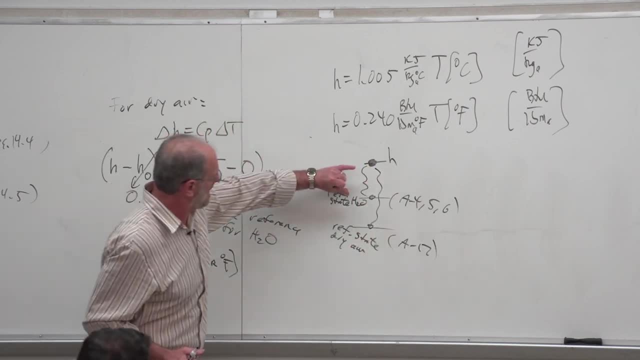 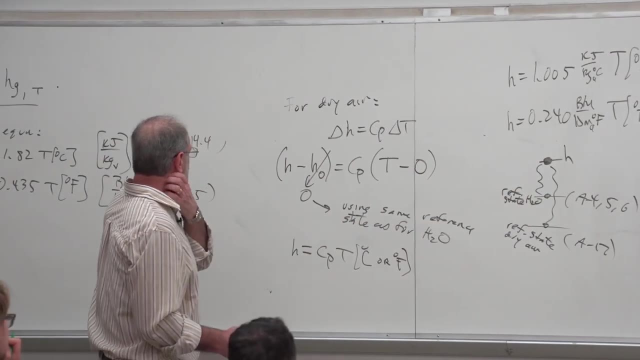 So we have two different reference states. You know we can't use that enthalpy data and that enthalpy data in the same equation. So that's what I've essentially done here. I just redetermined, if you will, the reference state for. 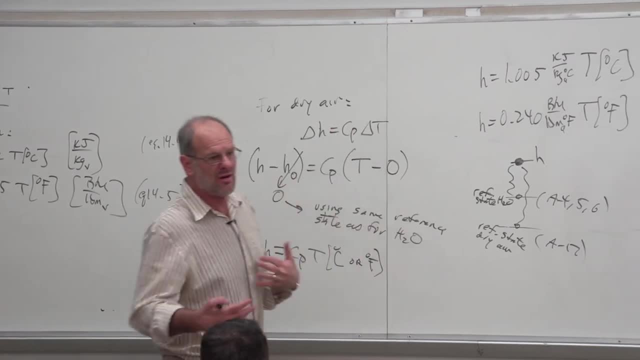 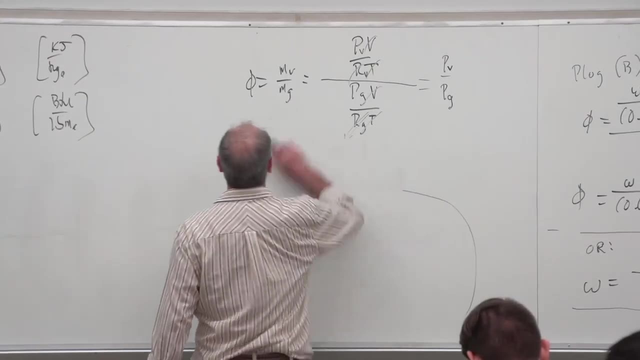 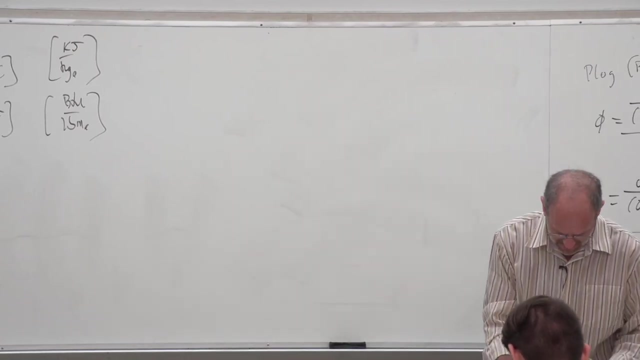 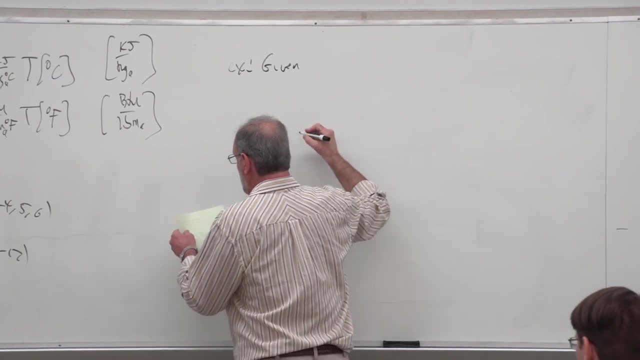 the dry air. I've just moved it up to here so that we can use it in our problem solving. So, with all this in mind, let's look at an example problem and get a feel for what a typical problem of this type is like. So let's say that we're given. 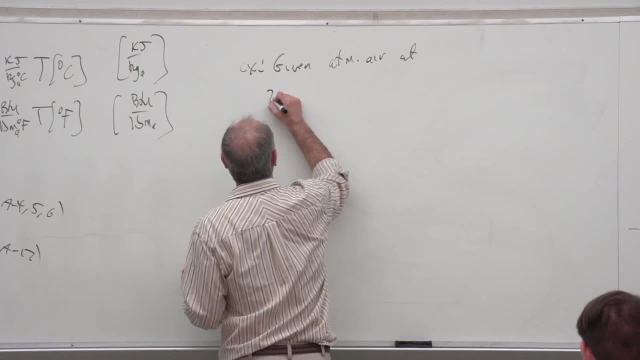 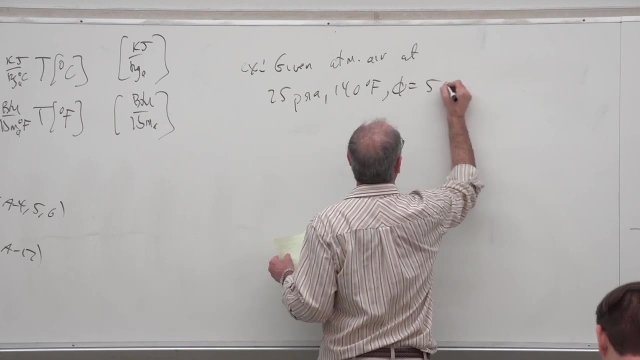 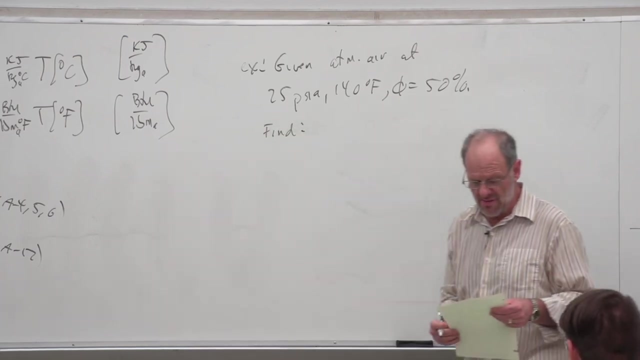 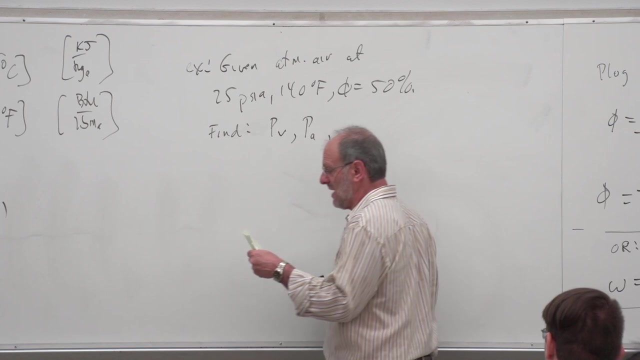 atmospheric air at 25 PSIA, 140 degrees Fahrenheit, with a relative density of 50 percent, And we want to find a variety of things. How about all those different parameters we've been talking about? So let's find the partial pressure of water vapor. Let's find the partial pressure of the dry air. Let's 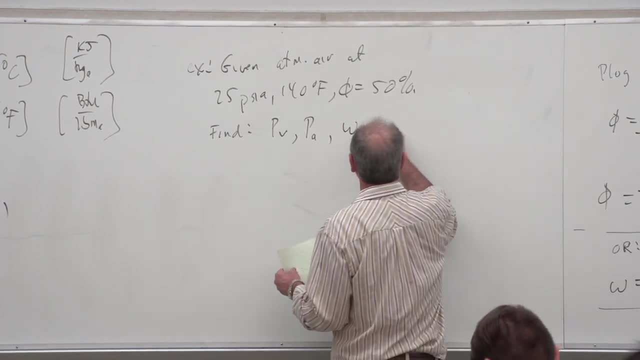 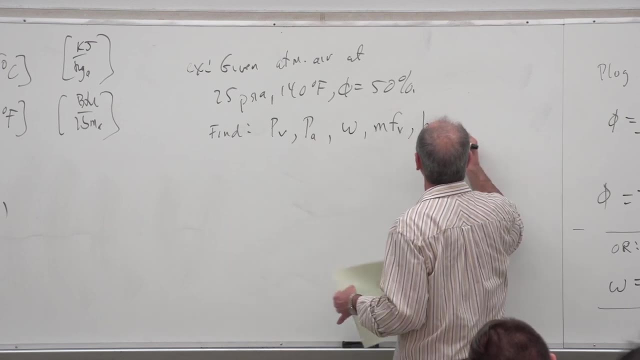 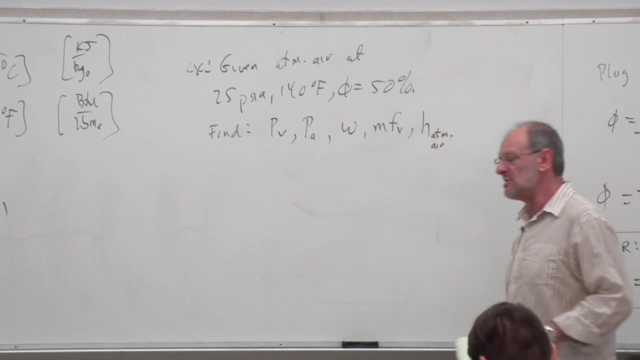 find the specific humidity. Let's also find mass fraction of water vapor in the air And let's also find the enthalpy of the atmospheric air. Let's find the atmospheric air. OK, So all these should be able to be found using the. 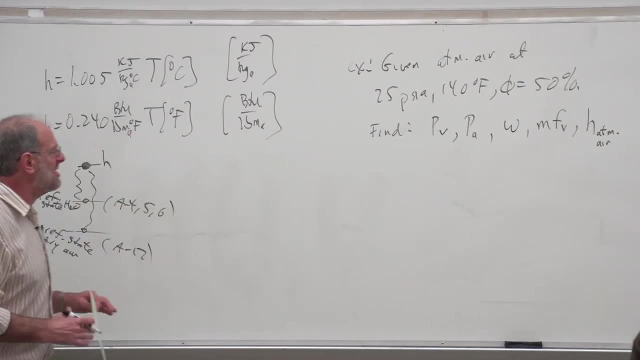 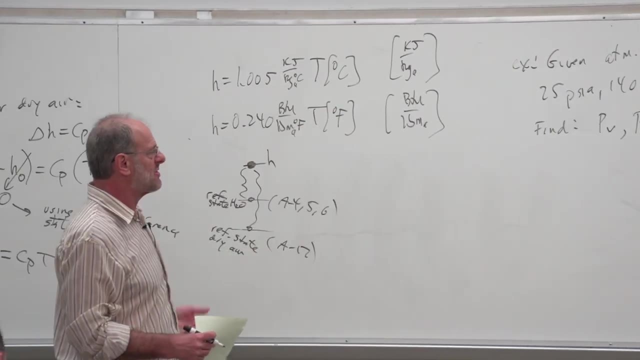 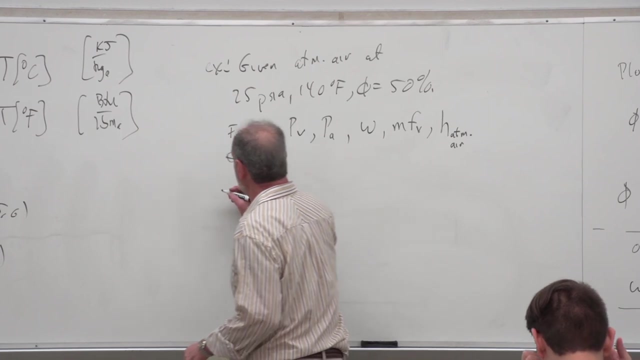 equations that we've already seen. Now let me note again, as we're solving these problems involving mixtures: often there's more than one way to go through the equations and still get the right result. It really just depends on what order you deal with the equations in typically, So let's just begin this one by going. 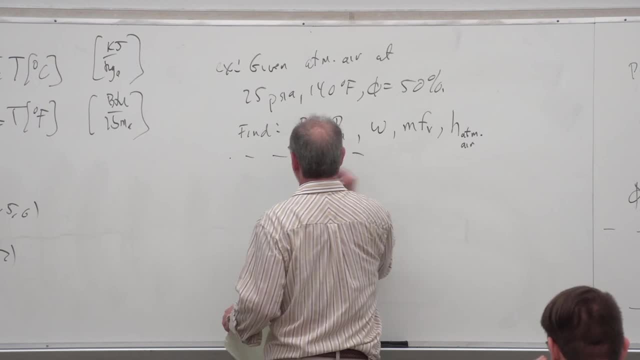 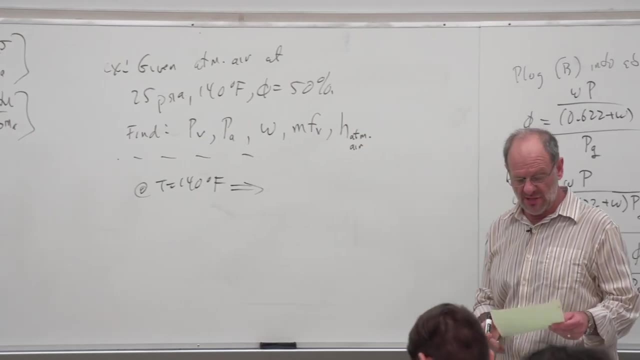 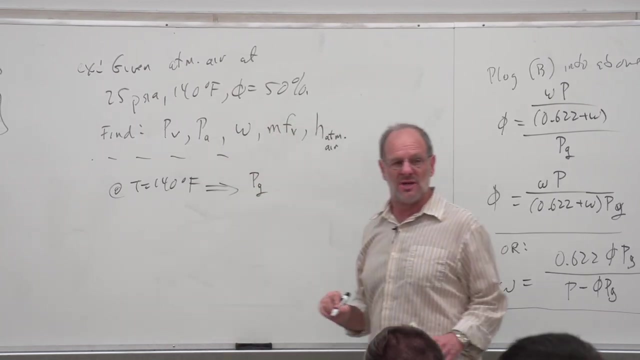 into our property tables at 140 degrees Fahrenheit, I mean. after all, that is the temperature of this particular mixture. And there's two things we're going to need as we peruse through these various equations. One thing we're going to need is the saturation pressure Right. This 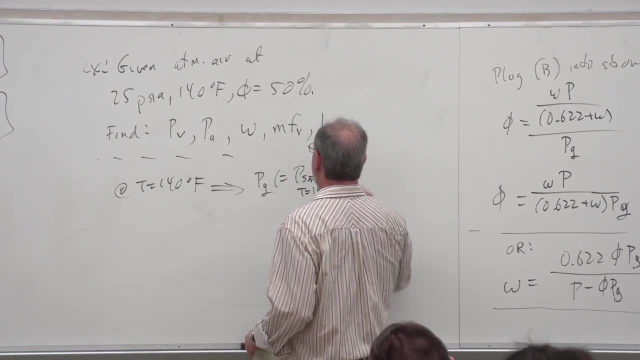 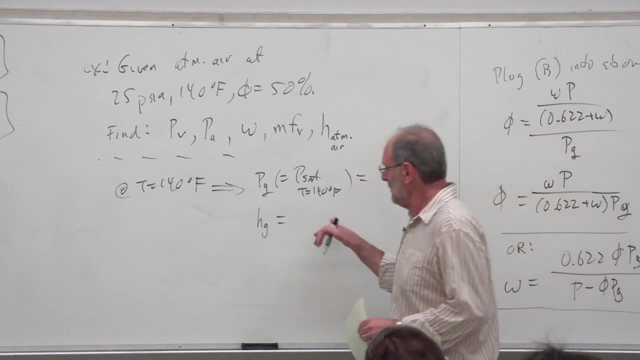 is PSAT at 140 degrees Fahrenheit. So we'll look that up, And we're also going to need the enthalpy of the water vapor. I'd much rather look up data in my tables, because I know it's nice and accurate, But I'm going to look up the water. 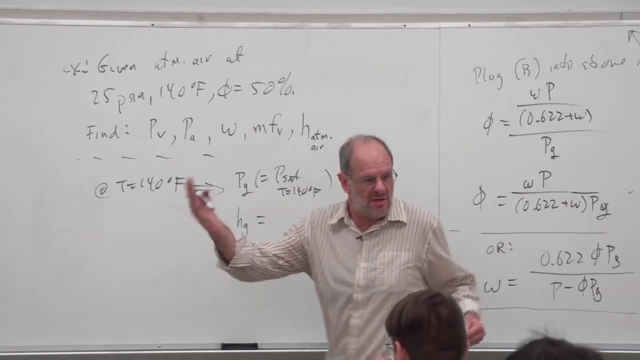 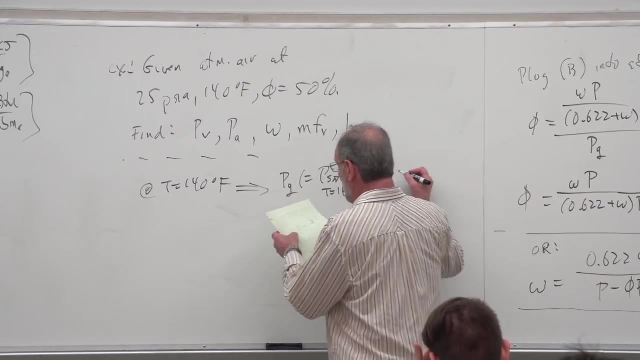 nice and accurate- rather than using an empirical relationship. I mean I could- The numbers aren't going to be off by that much, But for me it's just easier to go into a table and pick out one number than to use a calculation. So with all, 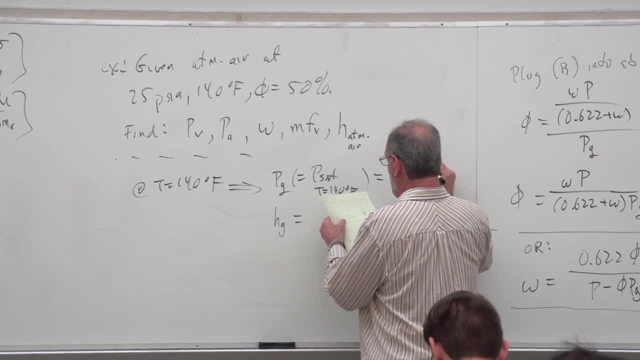 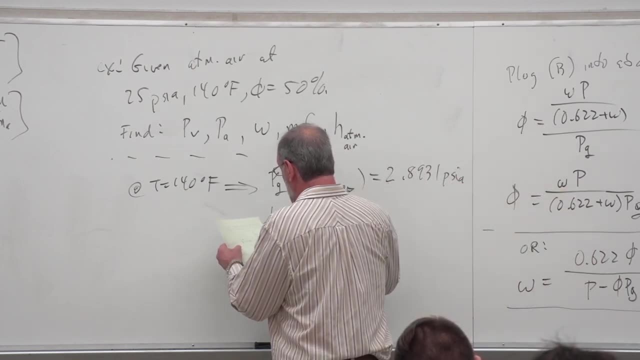 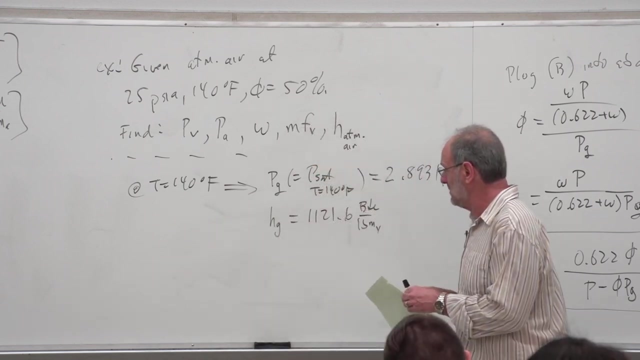 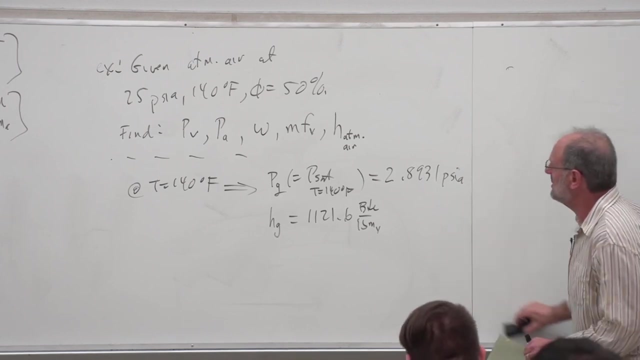 this. the saturation pressure at 140 is 2.8931 psi 8.. And then the enthalpy of saturated vapor is 1,121.6 BTUs per pound mass of water vapor. Again, I like to put a subscript on any mass term that I have, just to make sure I'm using the 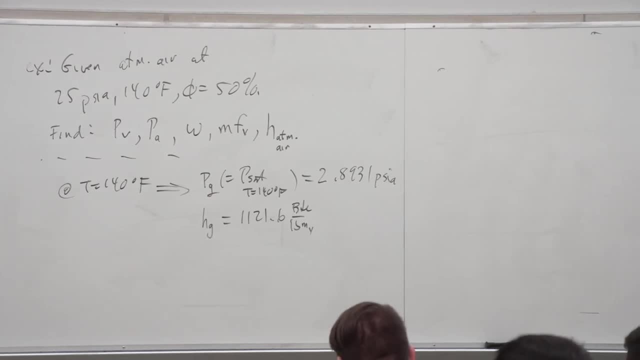 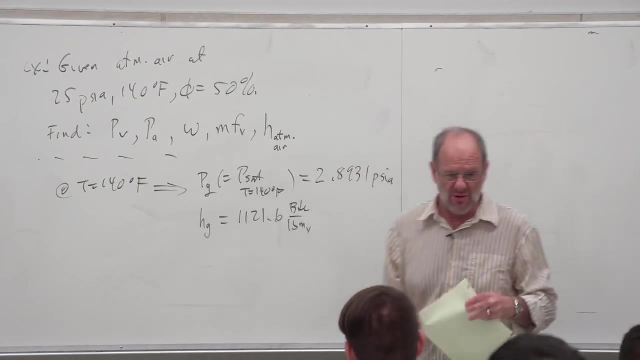 units properly. I mean eventually. when you start combining these terms to get the results we're looking for, you should definitely be carrying the units through, And a pound of air and a pound of water vapor are not the same thing, So carry the units through. 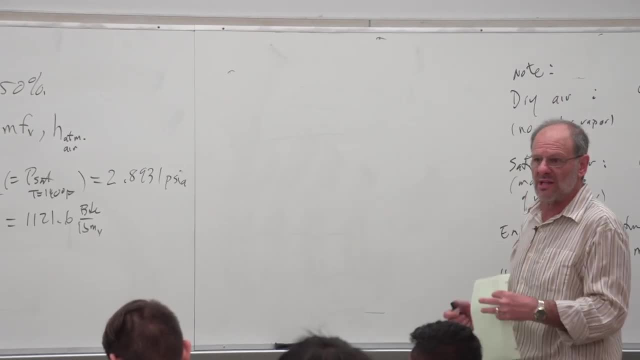 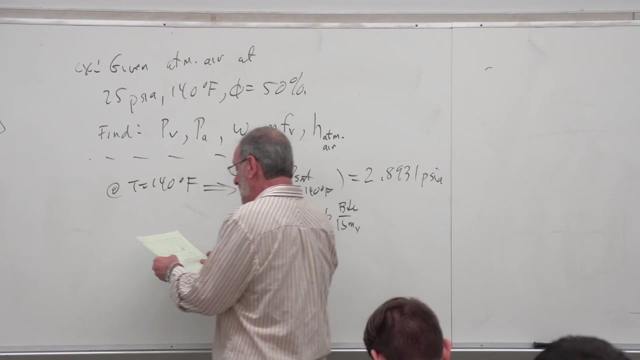 And, as usual, if the units work out properly, there's a good chance you've done the problem correctly. If the units aren't working out right, you missed something. Nonetheless, we have this data that we've looked up in this particular table. Now we can use the relative humidity along with the 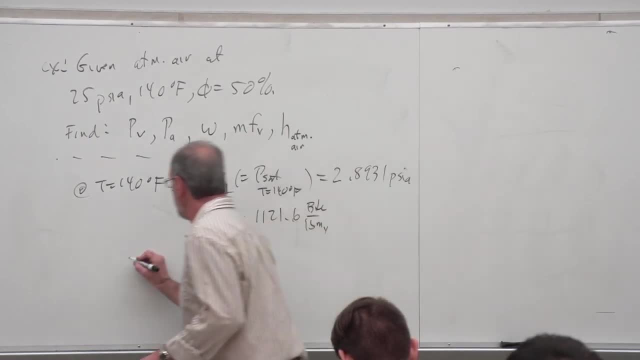 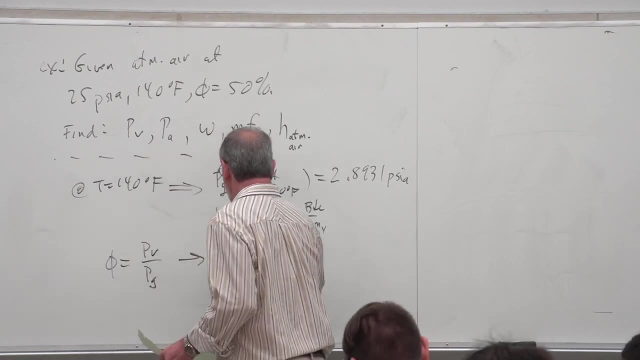 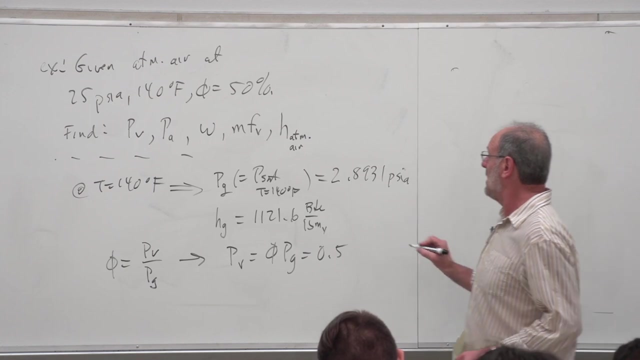 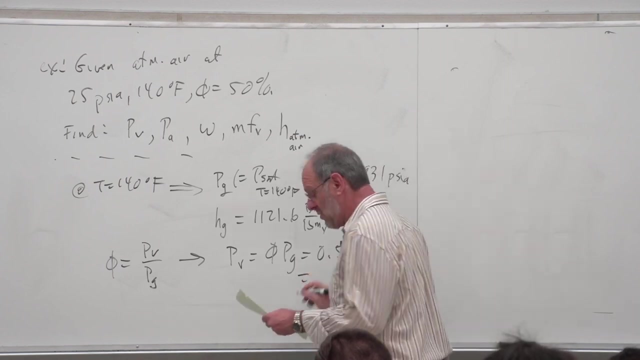 saturation pressure in order to get the partial pressure right. Relative humidity, as we found earlier, is just PV over PG, So therefore PV is phi times PG. 50% is the same as 0.5.. PG is identified above, So we get the partial pressure. 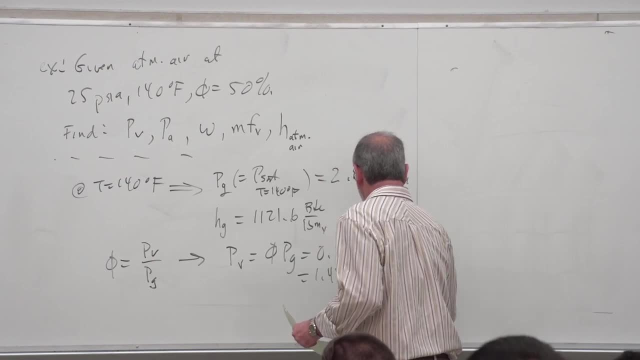 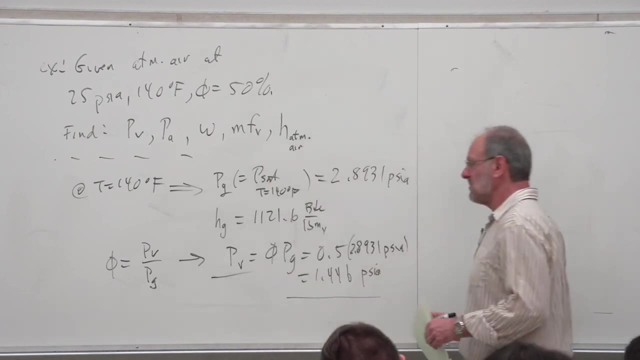 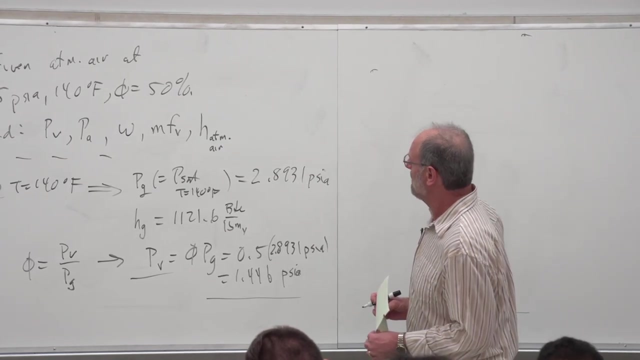 of water vapor: 1.446 PSIA. OK, So there's the first term. Next, we would like to be able to find the partial pressure of the air. That's probably the easiest one. We know that the total pressure is just the sum of the two partial. 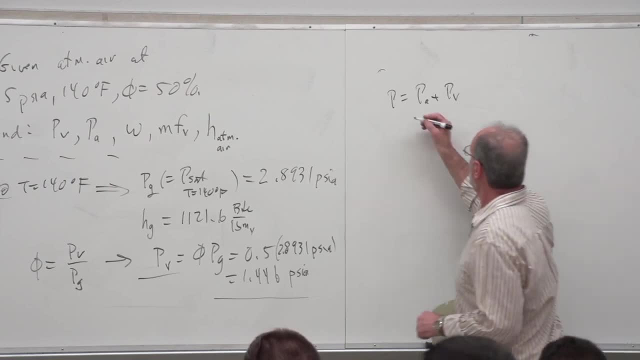 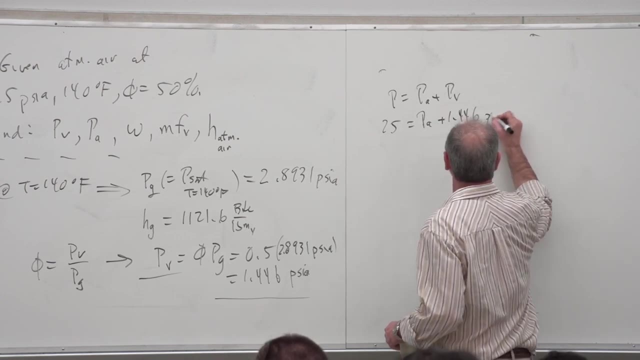 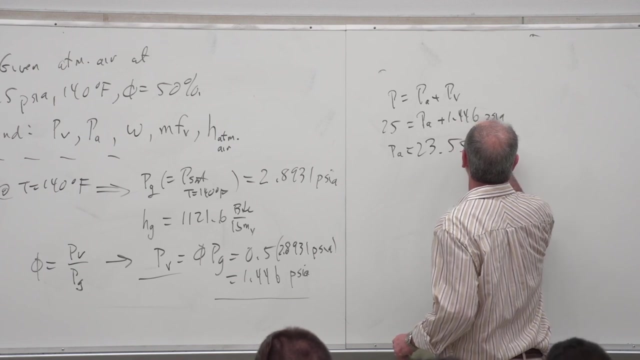 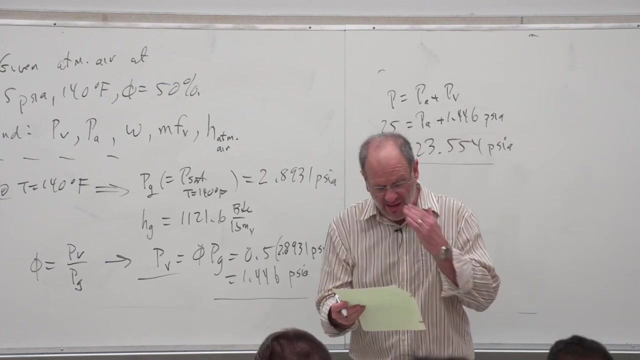 pressures? Really, I should say dry air, not air. Well, so 25 PSIA equals the pressure of the air plus 1.446 PSIA, And therefore the partial pressure of the dry air is 23.554 PSIA. OK, So we have the two partial pressures. Now why don't? 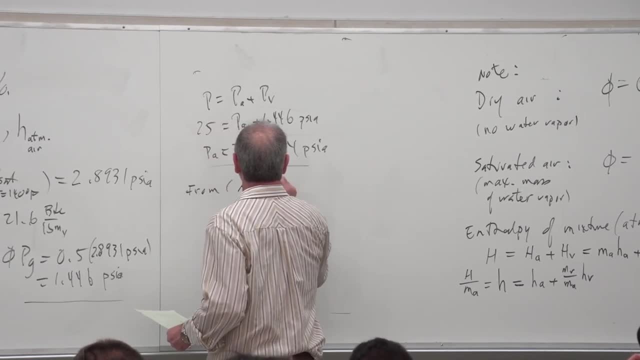 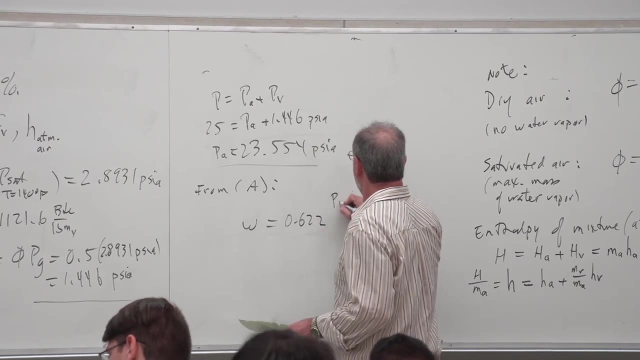 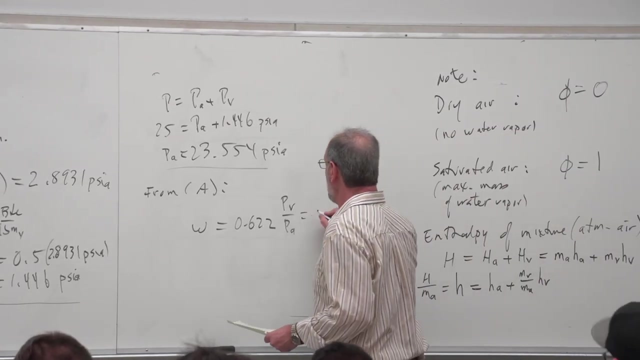 we use equation A in order to find the absolute humidity, And this is just 0.622 times PV over PA. Again, there are other forms of this equation that one could have used, but this one makes the most sense at this point. So 0.622 PV. 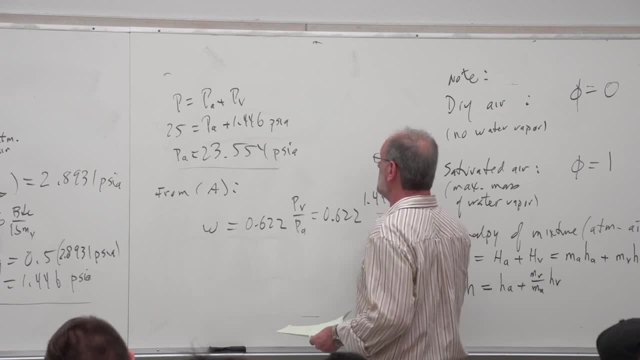 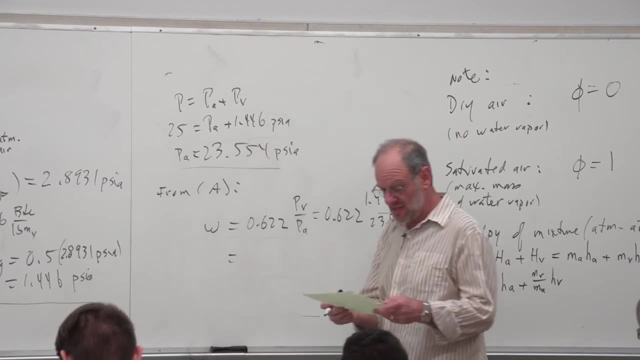 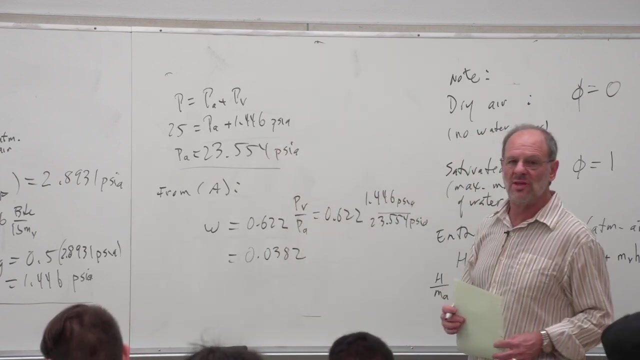 we know, And PA we know, We've made sure that our pressure is equal to the same, We've made sure that our pressure units are exactly the same And we end up with 0.0382.. OK, Now the units. I probably should have continued, or should? 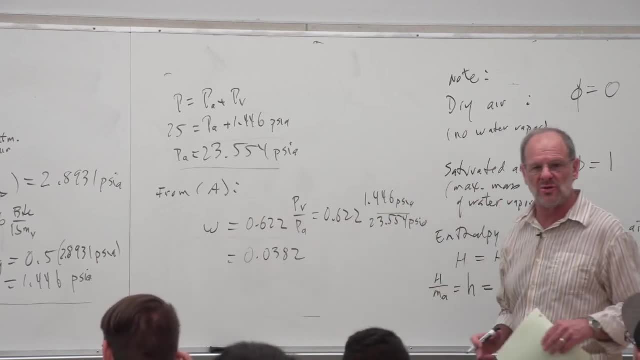 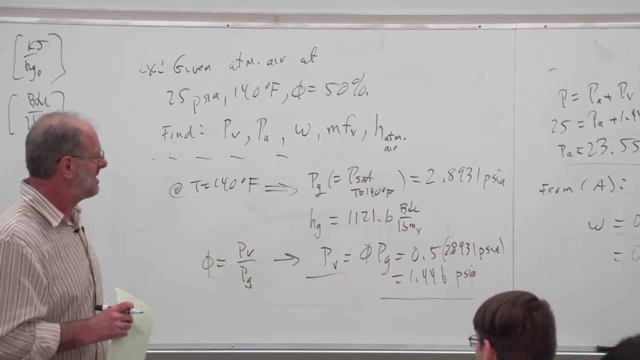 carry through This equation, this 0.622, you may recall that that's just the ratio of the gas constants. Right, And the gas constants have essentially the same units, BTUs per pound per degree, except the gas constant for the water. 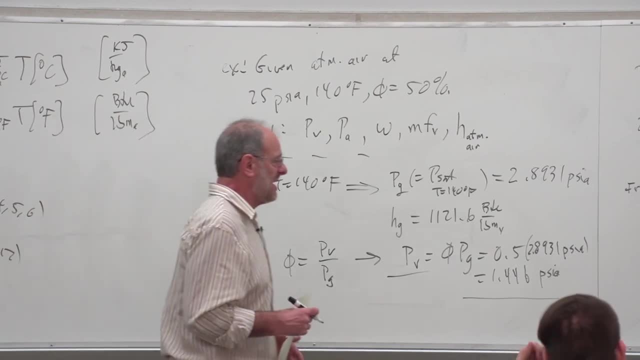 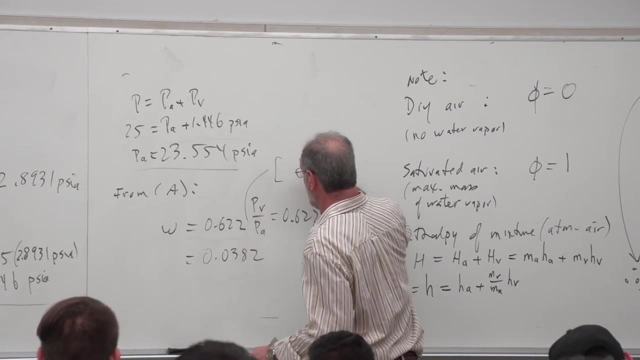 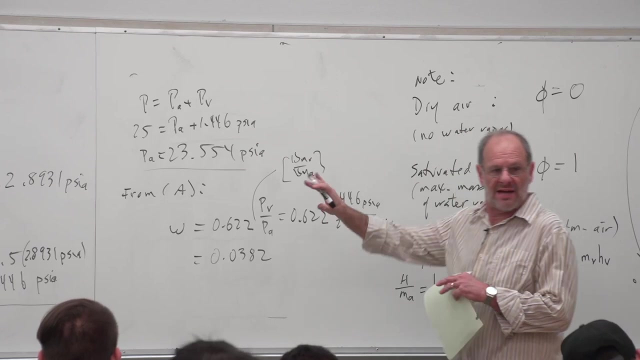 vapor is per pound mass of water vapor And the gas constant for the dry air is per pound mass of dry air. So actually hiding within this 0.622 are some units. The units are pounds mass water vapor per pounds mass of dry air, So you can go. 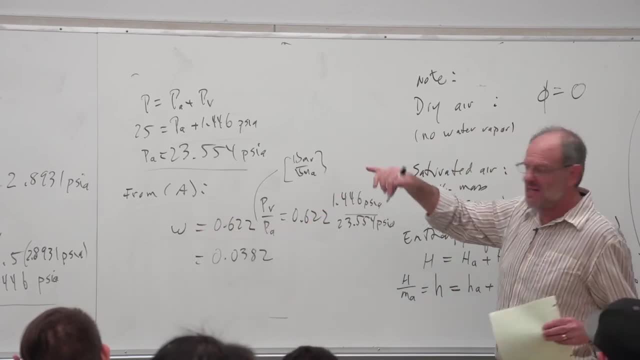 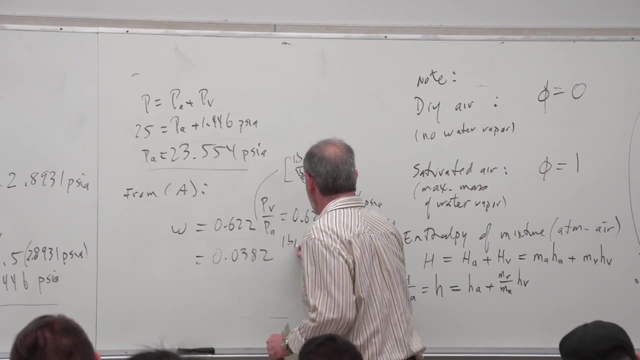 back to the derivation from last time, when I derived equation one right at the end last time, And you'll see this is nothing more than the ratio of those two gas constants. So it turns out the units are indeed pounds mass of water vapor per pound mass of dry air. If you just look at the pressure units, they're going. 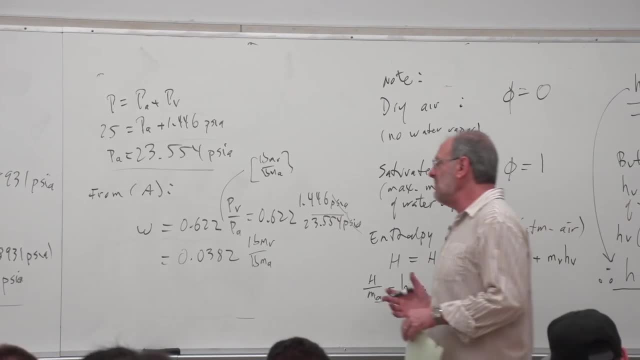 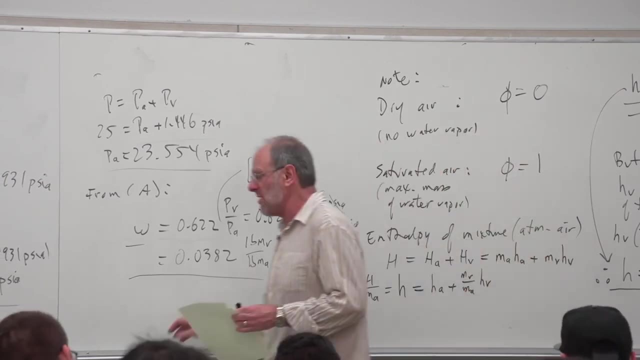 to cancel And it might appear that this is dimensionless. Now some people might argue that it is dimensionless because you have mass units in both numerator and denominator. I would argue otherwise. It's not really dimensionless because you've got the mass of two different components. So yeah, they both have the. 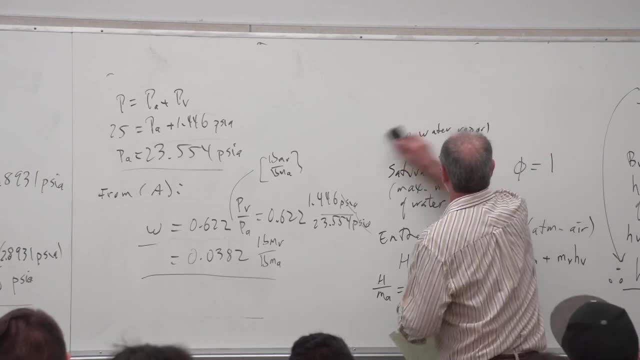 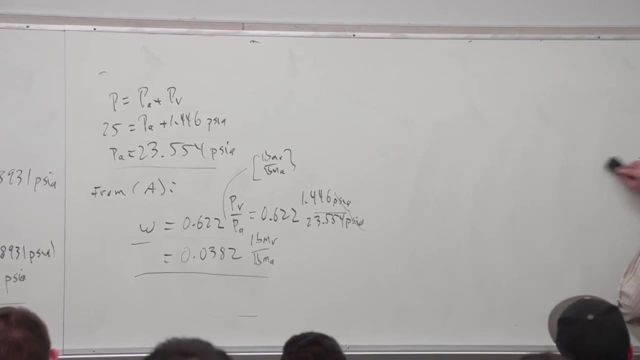 same units pound mass, But certainly it's not dimensionless. It's the mass of two units pound mass. It's the ratio between the water vapor and the air- Well, again, I should say dry air, All right. so now we found omega And let's move on. 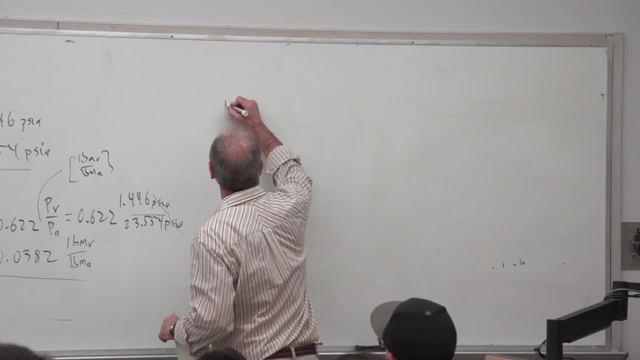 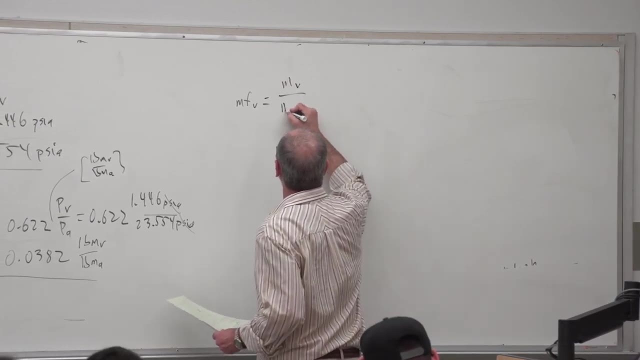 and find our mass fraction. So we're looking for the mass fraction of water vapor And we know that this is just the mass of the water vapor divided by the total mass right, the mass of our mixture, which is our atmospheric air. You 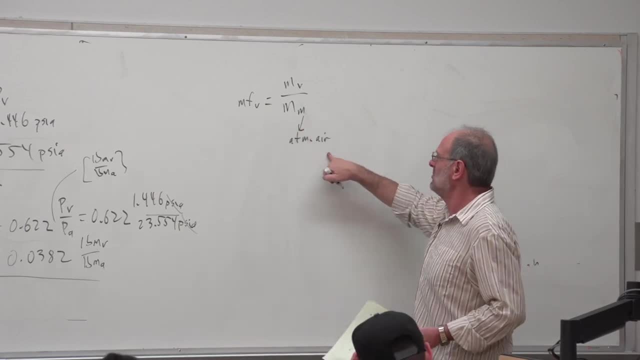 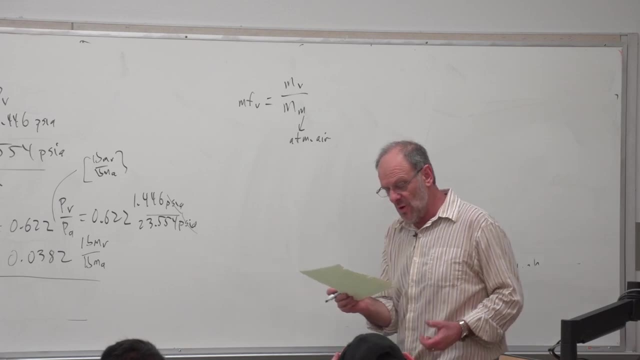 know, sometimes, as we go through problems, I'll use m for mixture, I'll use the word atmospheric air. It's the same thing, But we know that it's the total mass in the denominator versus just the water vapor mass in the numerator. And of. 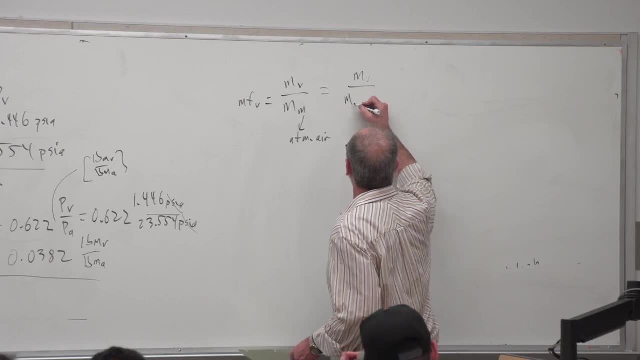 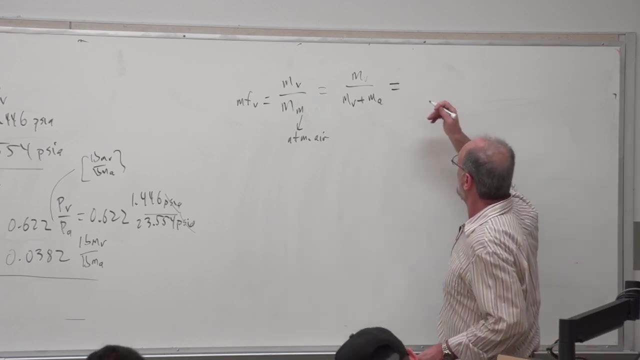 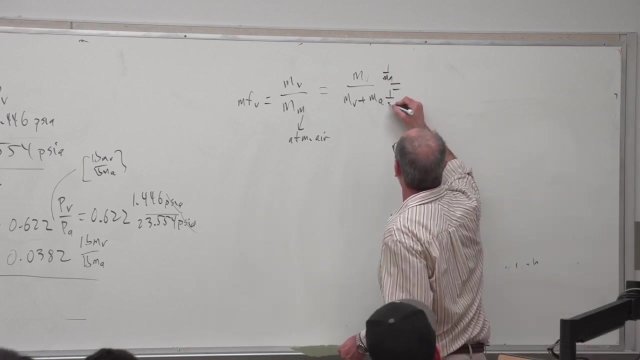 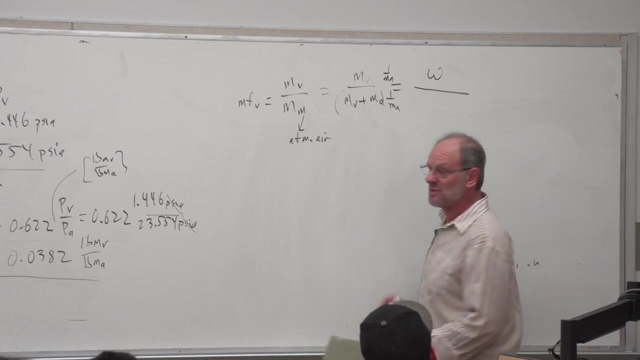 course, the total mass is just the sum of the water vapor plus the dry air component. And now I can just divide both numerator and denominator by ma right Right. And in doing so, well, let's see mv over ma. well, that's what we. 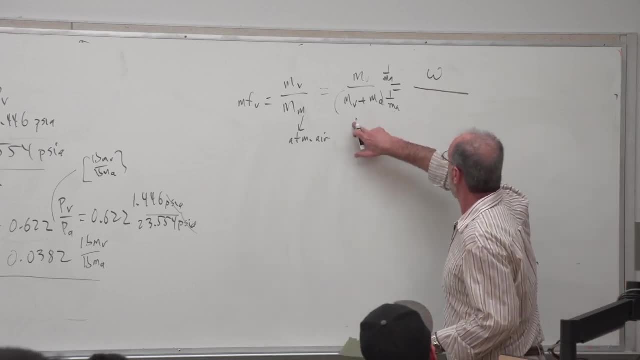 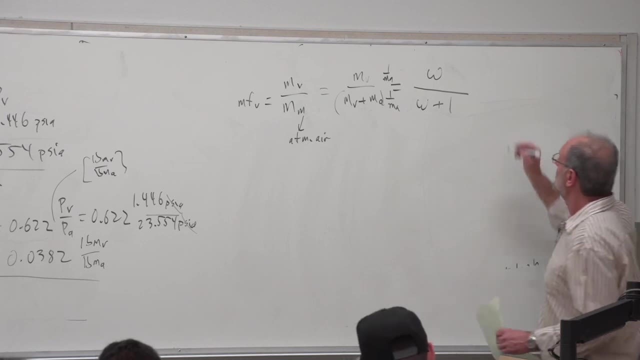 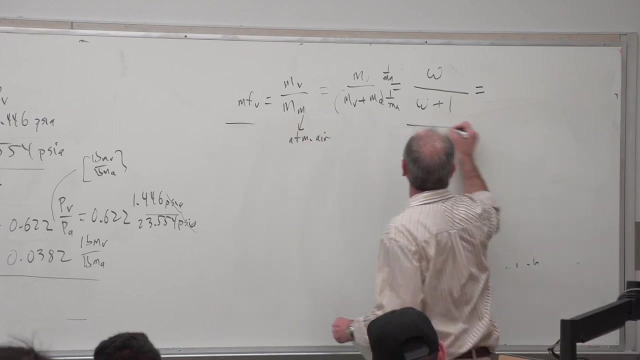 defined as omega. And here's another: mv over ma And then ma over ma. So this is just omega over omega plus 1.. So it's actually pretty straightforward. You'll never have to derive this equation again. Just remember that the mass fraction 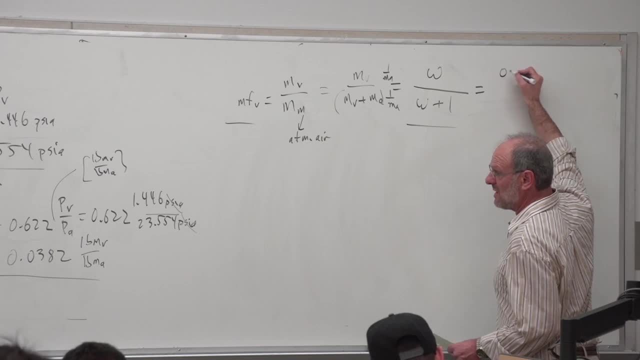 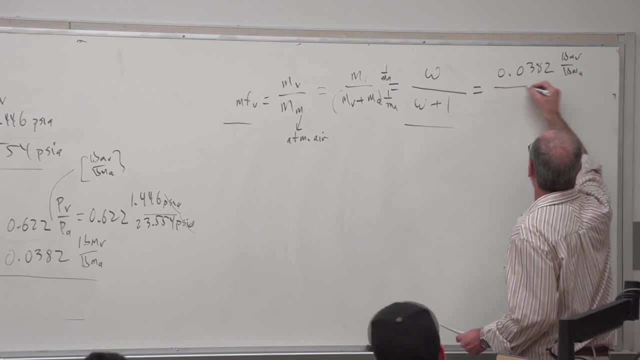 is omega over omega plus 1.. So we just plug in the numbers, We have omega 0.03, 382.. This would be pounds mass water vapor per pound mass of the dry air And then over omega plus 1.. Note that omega plus 1 is going to be pounds water vapor. 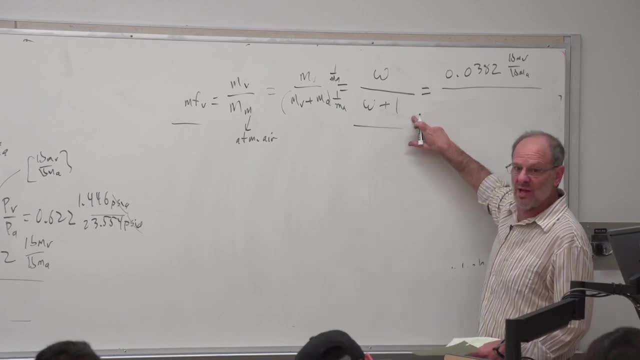 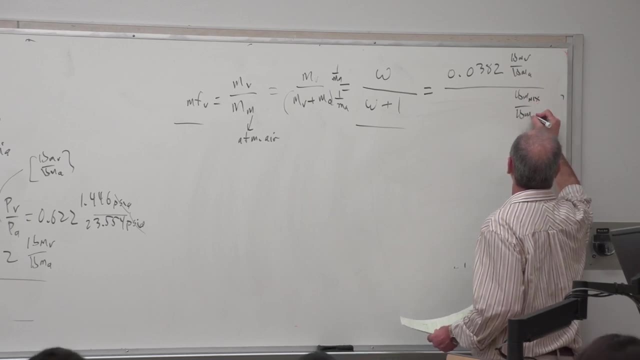 per pound dry air plus pound dry air per pound of dry air. In other words, it's the mass of the mixture per unit mass of dry air, And numerically this is going to be 1.0382.. Okay, So, nonetheless, the air mass is calculated And then the 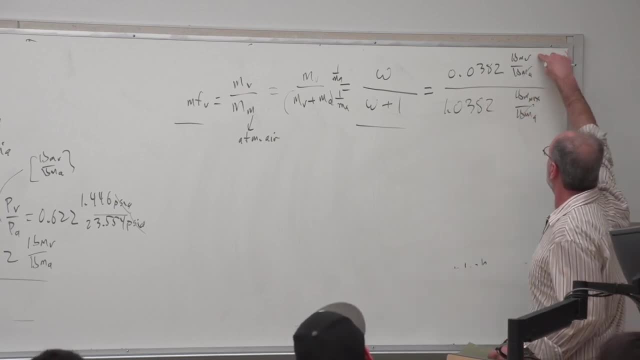 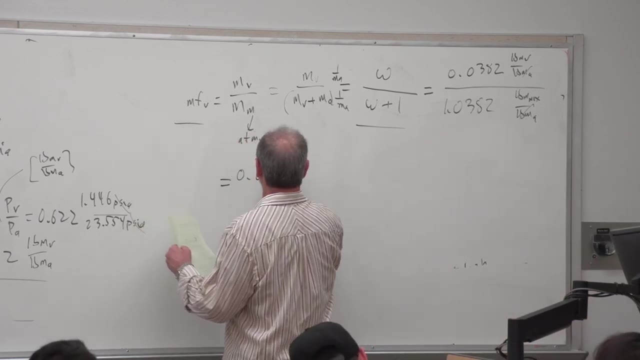 air mass is canceled And we get the mass fraction, which is water vapor, per unit. mass of mixture, which is the right units, And mathematically this just becomes .0368 pounds mass water vapor per pound. mass of the air water vapor. 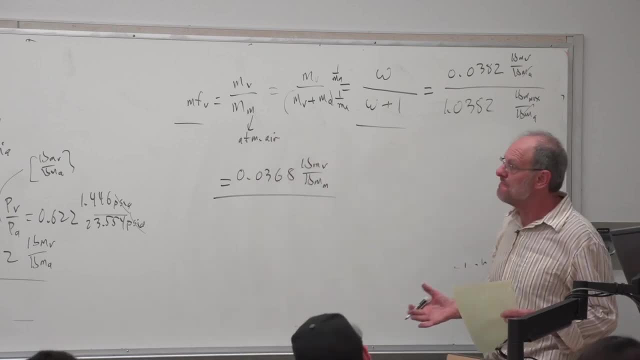 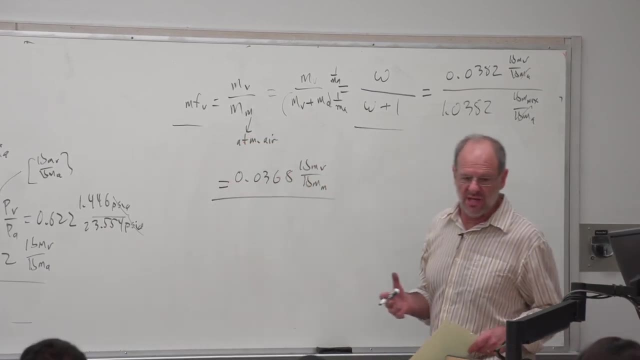 mixture. So there's the mass fraction term, And then the next thing we want to do is find our enthalpy. Now, remember again, we're not just going to take the enthalpy of the air and the water vapor and somehow add them together. We have 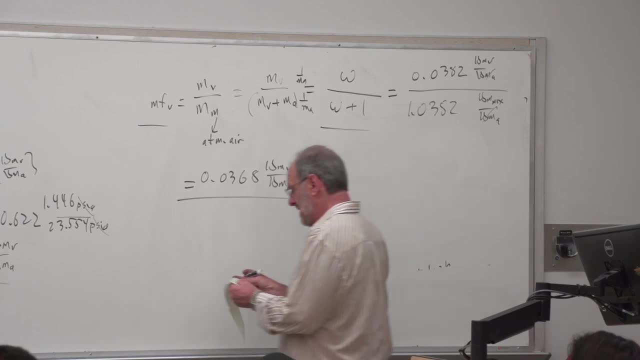 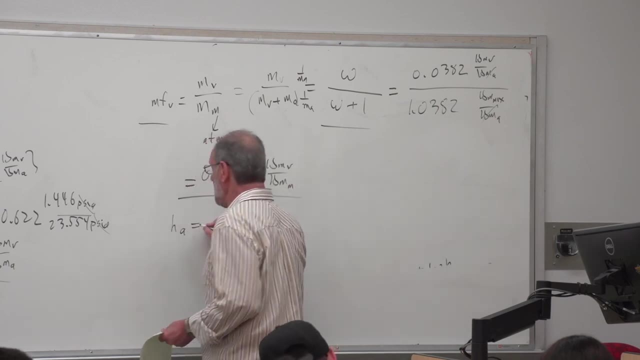 to use the appropriate equation from earlier. So we already have looked up HG, so we don't need that anymore. Let's find HA And again we're going to have to use the appropriate equation, which is just CP times the temperature in. 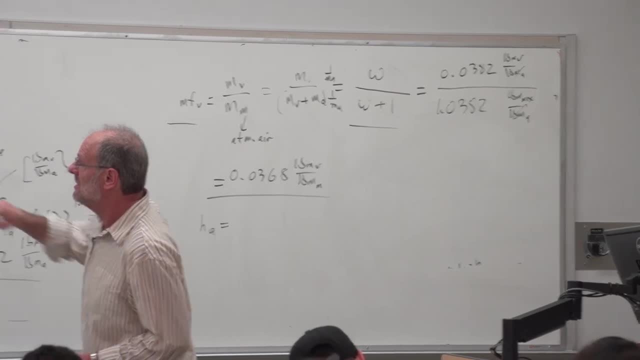 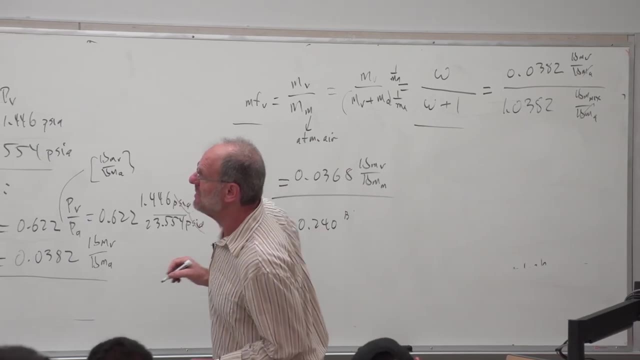 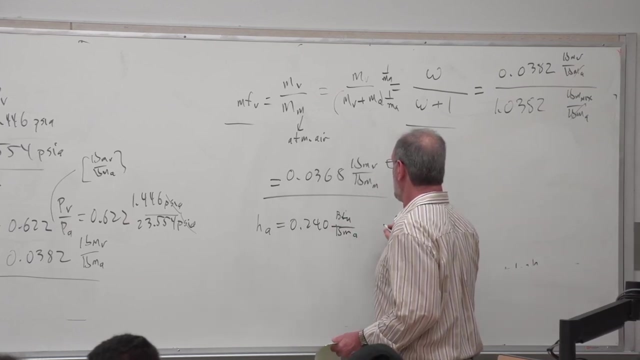 Fahrenheit, since this problem is in the British system of units, So .240.. And this is going to be BTUs per pound. mass of air vapor per unit. mass of the air vapor per pound, mass of the dry air, And then multiplied by the temperature. 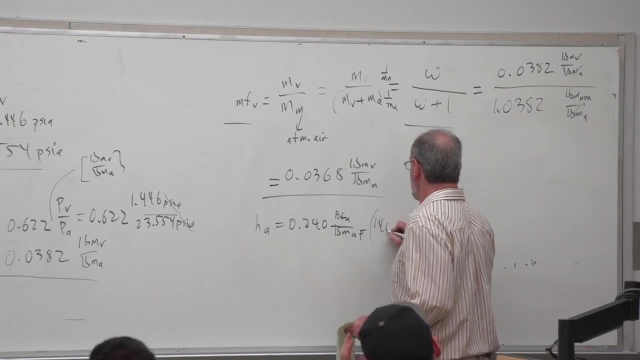 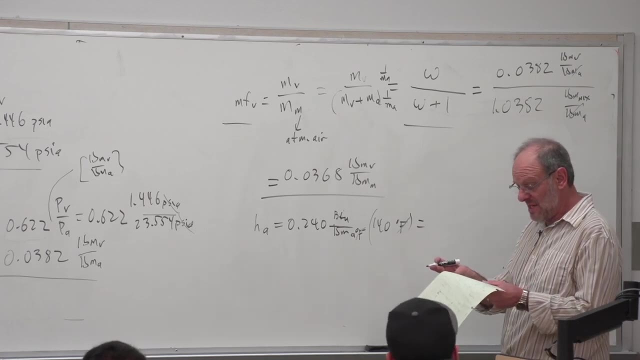 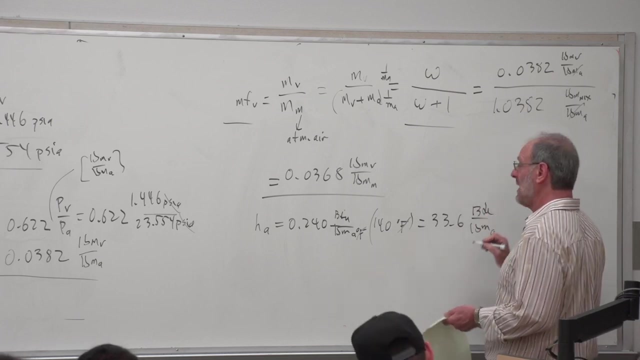 And in this particular case the temperature is given as 140 Fahrenheit. So just 140 Fahrenheit. So temperature units cancel And we go through our math And we get 33.6 BTUs per pound mass of dry air. So there's the data, And then we get. 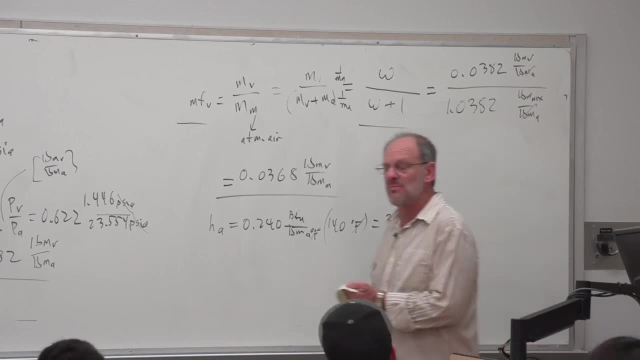 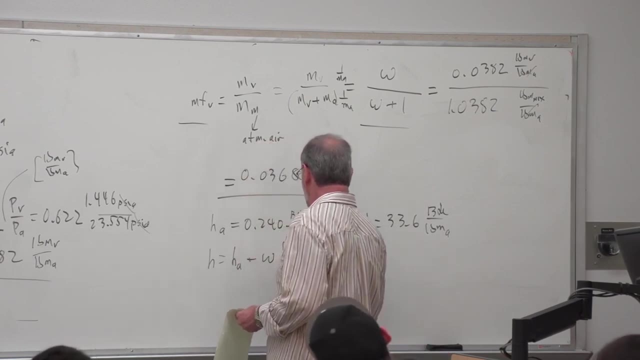 omega for the dry air component. And then the last step is to use the equation that tells us that the enthalpy is just the enthalpy of the dry air, plus omega times the enthalpy of the water vapor And, of course, the water. 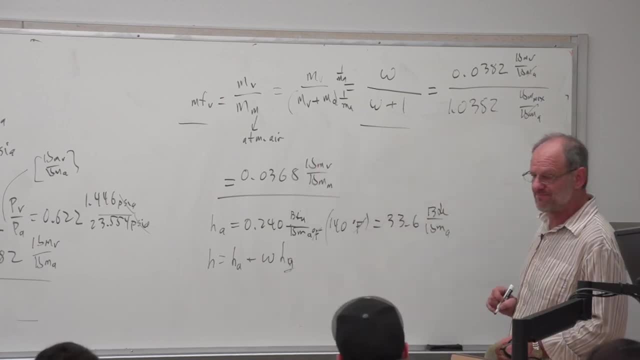 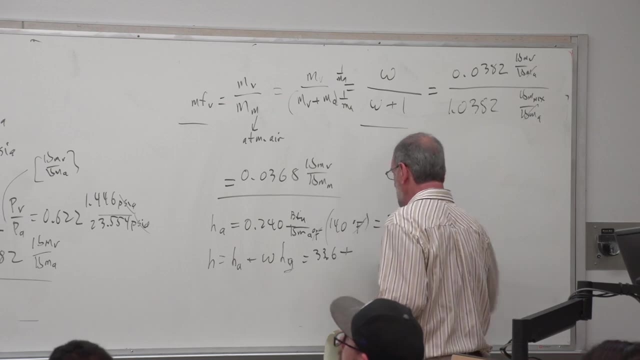 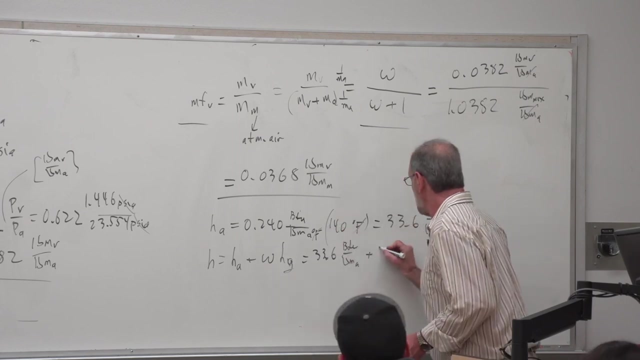 vapor. we've now come to call just HG, So plug in the numbers 33.6.. And let me just continue with the units. So this is BTUs per pound mass of dry air plus and then the omega term: .0382 pounds of water vapor per pound mass of dry air. 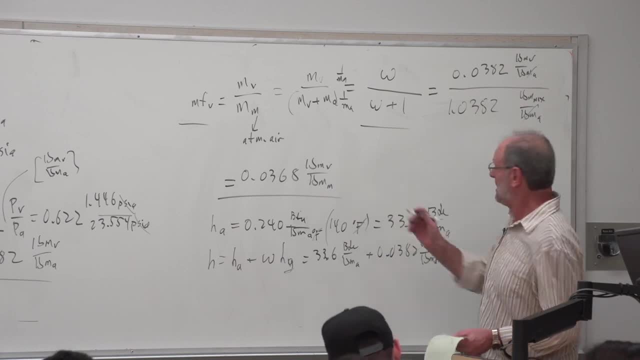 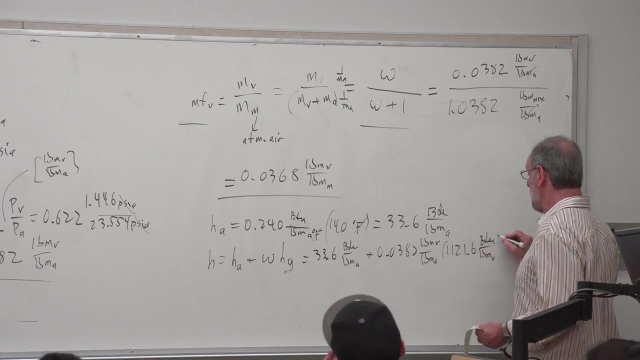 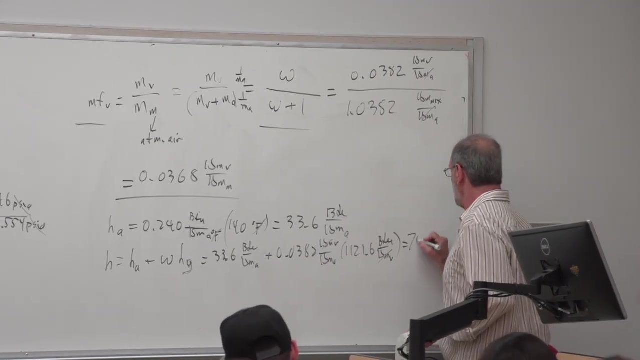 And then times HG for the water, which is 1121.6.. This is BTUs per pound mass of just the water vapor, right? So you can see the water vapor masses cancel And we just get one result here: 76.5 BTUs per pound mass of dry air. So that's the 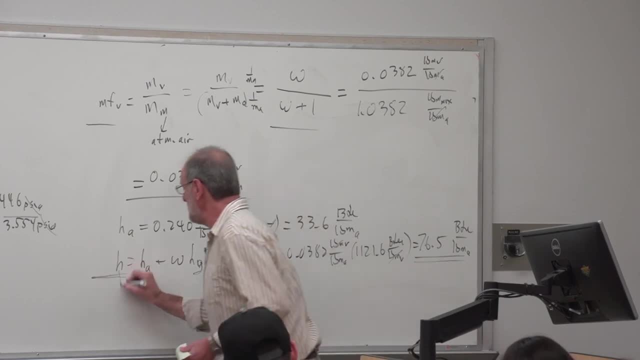 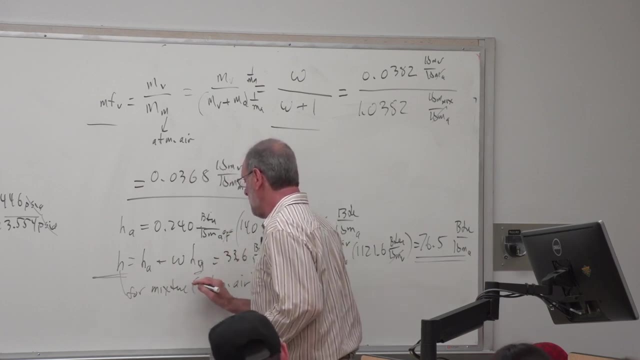 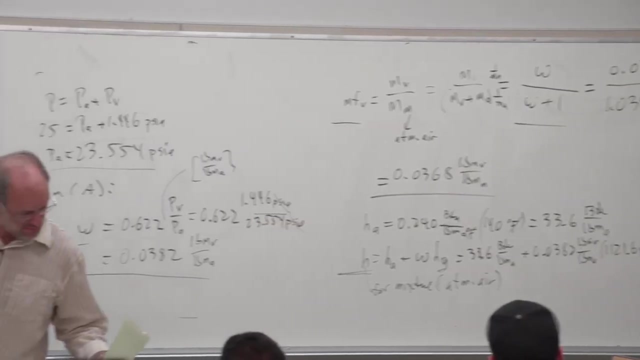 unit mass of dry air. Again, this is for the mixture, which is atmospheric air, But it is on a per unit mass of dry air basis. That might not sound so important right now, but it is important. Keep in mind that this material here in 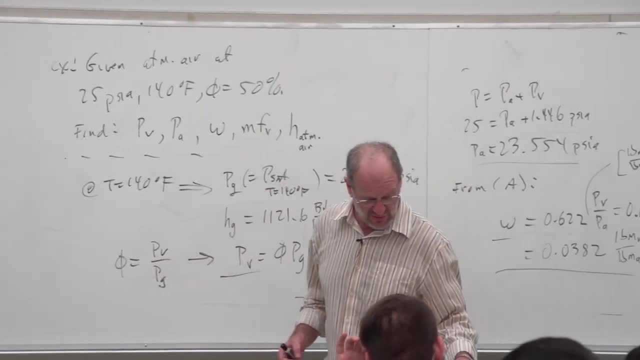 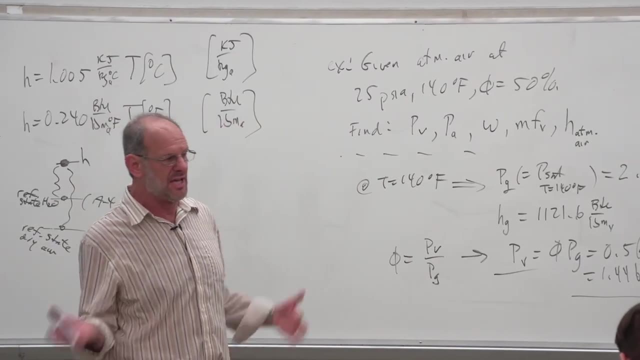 Chapter 14 is really just a prelude to the air conditioning problems that appear later on in Chapter 14.. Okay, When we saw the air conditioning problems, guess what? Back to the first law of thermodynamics. again right, We're going to need enthalpy data because in 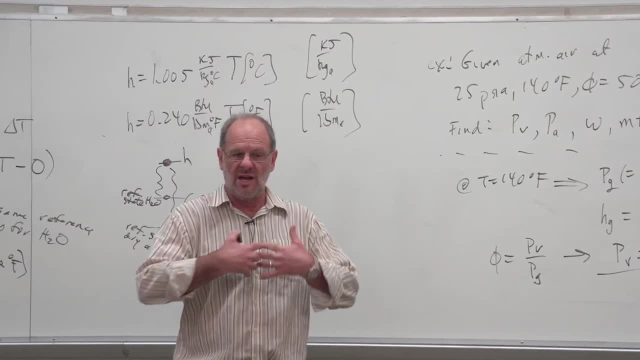 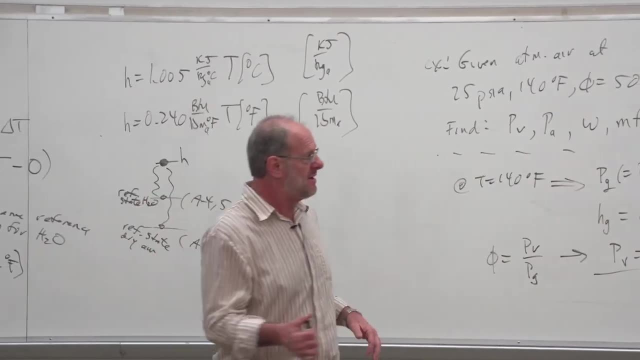 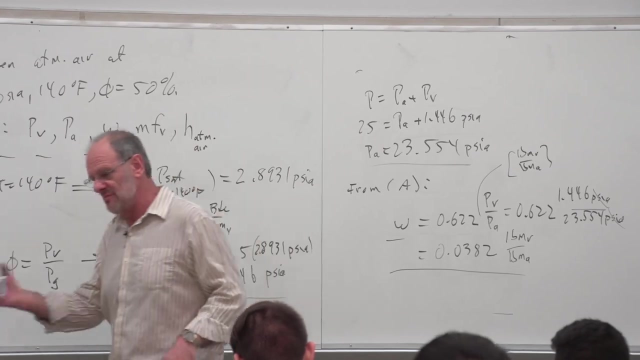 air conditioning systems. these are flow systems. right, We've got air flowing through heat exchangers. We've got air flowing through devices that will add moisture or remove moisture from the air. We need to keep that in mind, that we're not just doing this again because it's fun, of course, which it is, But we're 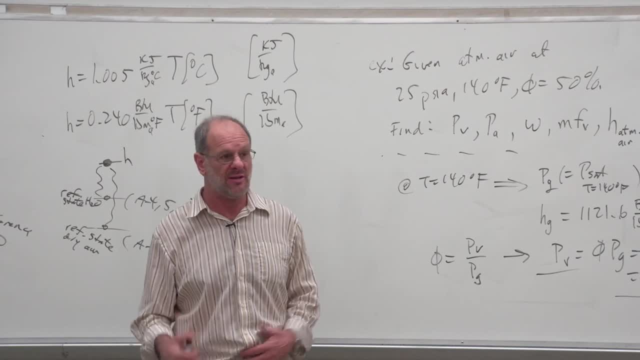 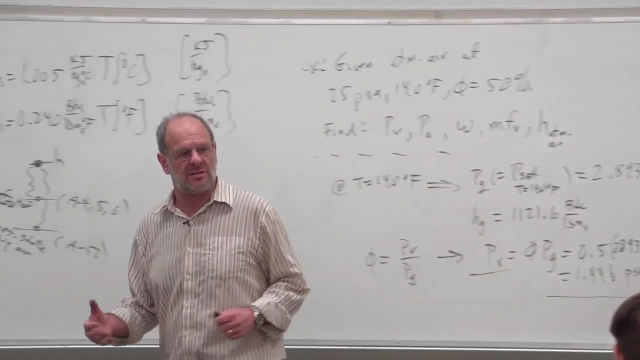 doing it so that we can solve future problems, Future problems in air conditioning, First law problems involving steady flow systems, All right, So any questions just in general about this. Remember again, this is just the data that we're going to end up using in some future problems. 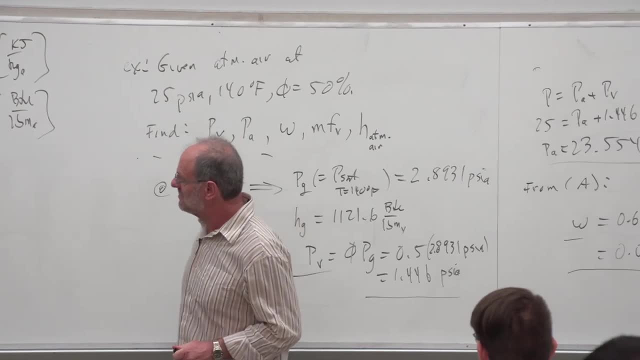 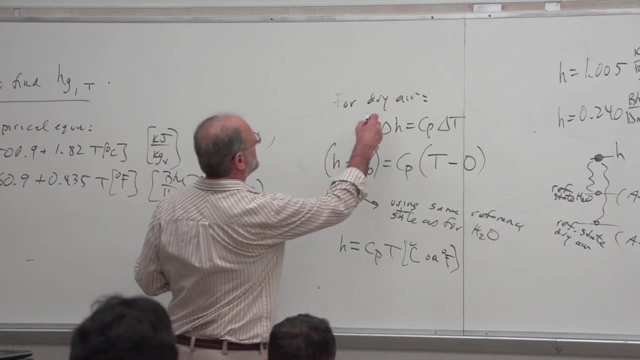 Yes, So the variation when you take the energy? Yes, yes, This is just for the dry air. Oh, in fact, you know- I think that's a good point- that I probably should have put HA here and HA here, just so that I. 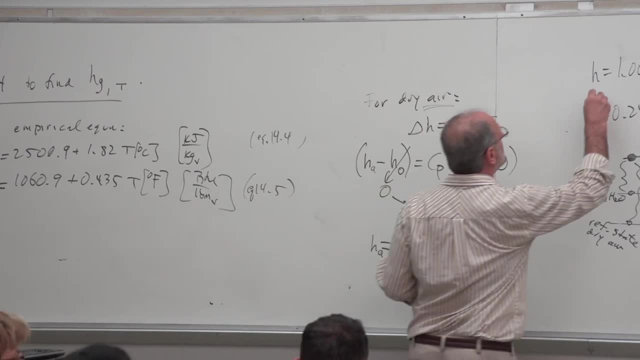 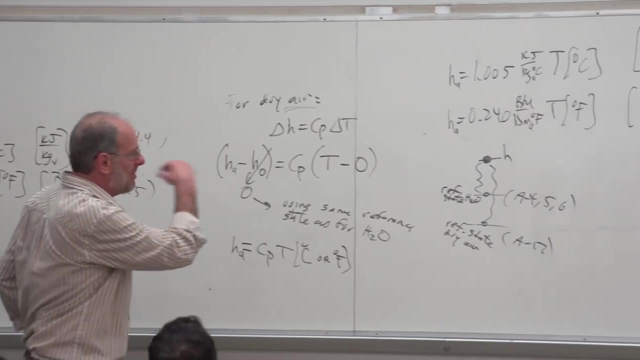 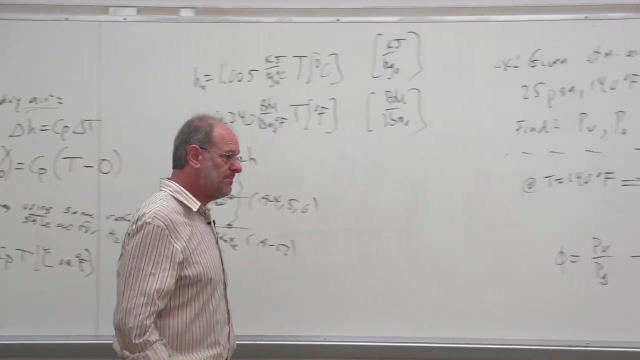 it's really specific to us that this deals with just the dry air component. So, yeah, if you would all again go back to your notes by a page or so and just make the note there that that represents the dry air And also, I think, the reference of when you're using the reference. 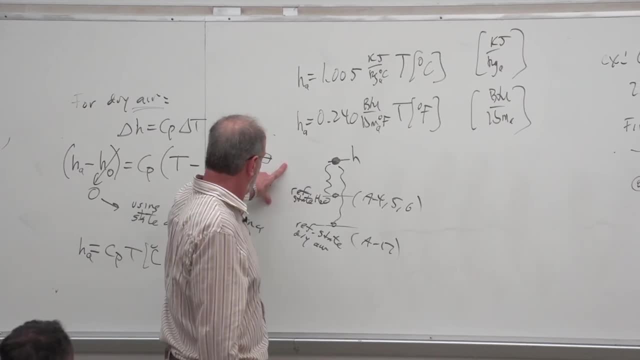 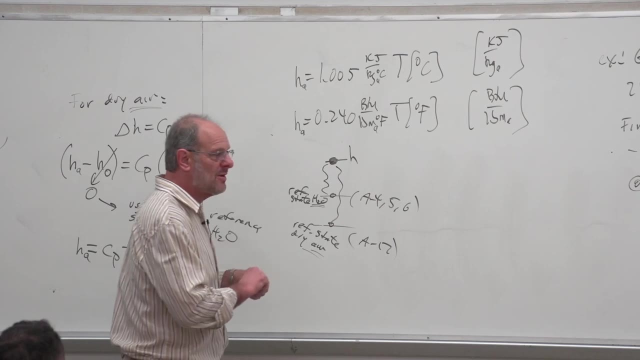 state. So for people like, it would give us HA, but as people A4,, 5,, it would give us HV. Right, right, This is for water and this is for the dry air. So yeah, And again, this is just to illustrate how they have different reference frames. so 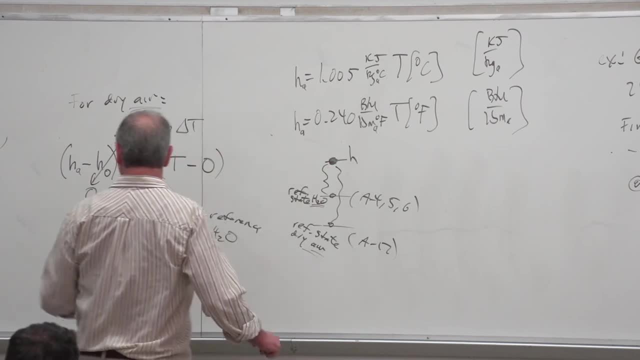 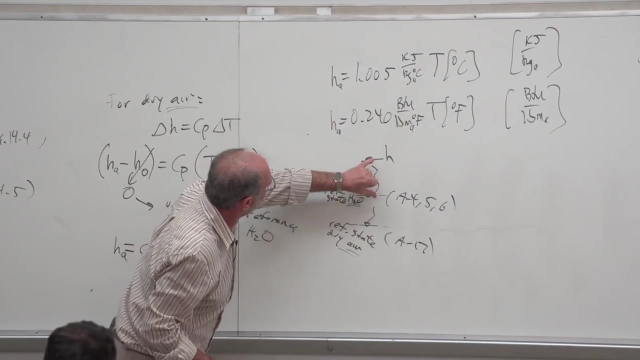 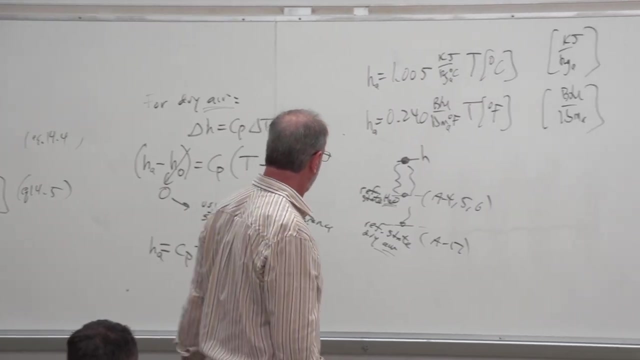 that you know we can't use this data. Essentially, by using this equation, we've subtracted off this amount so that we're really just left with this amount, so that our reference frames are the same. Yeah, but it means the subscript will be different depending on the table. 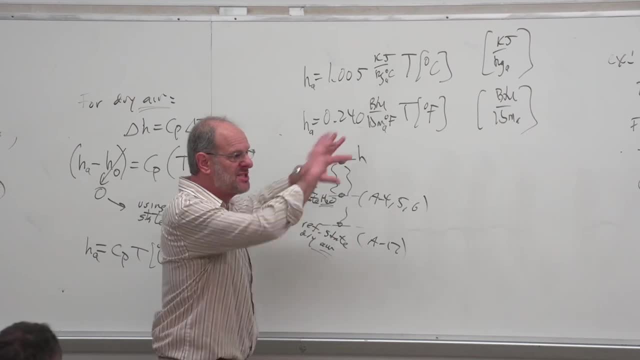 Correct. But let's just note we're never going to use table A17.. So again, I mean, in these types of problems I bring this up just to specifically note that we can't use table A17 because of the different reference states. So 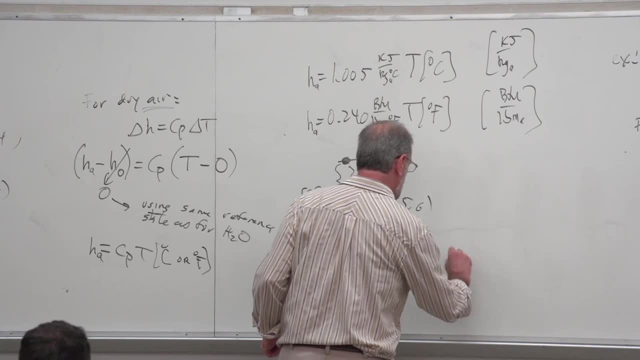 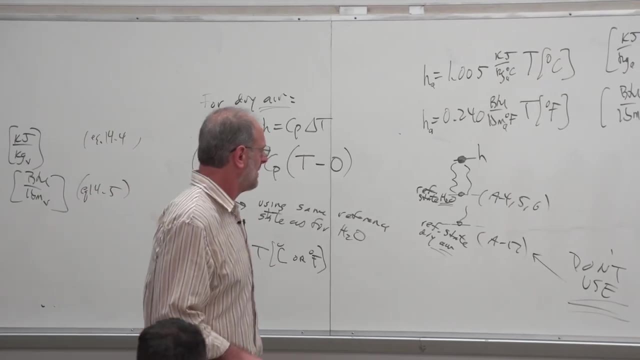 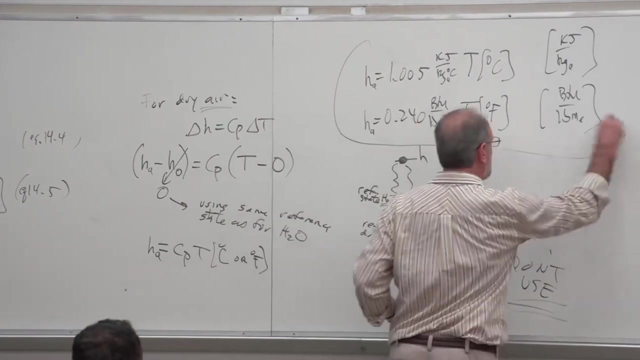 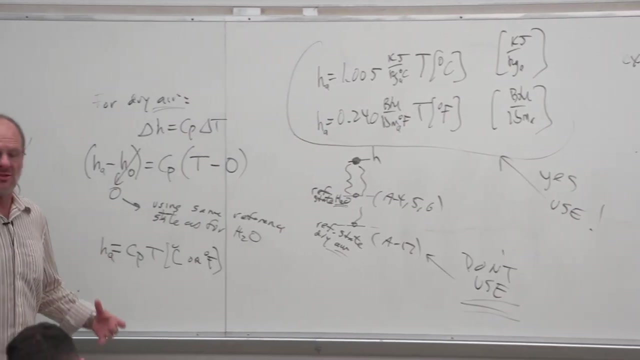 never use table A17, right, Never used. It just doesn't have the right datum, datum meaning reference state. So this is what we use, these equations, right? Any other questions on this? All right, So now let's move on to the next. 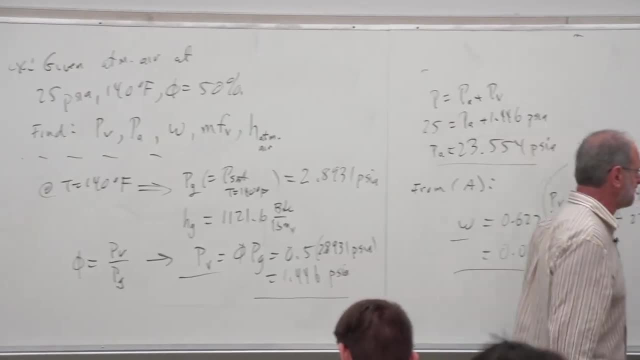 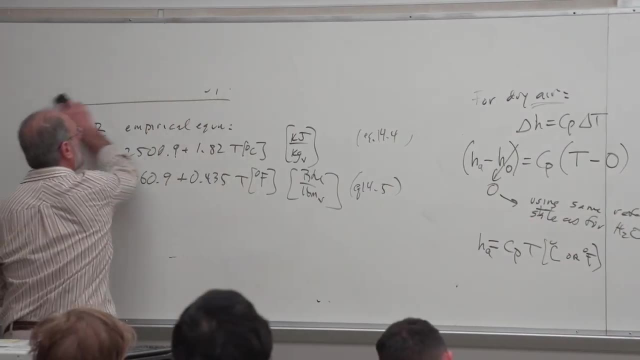 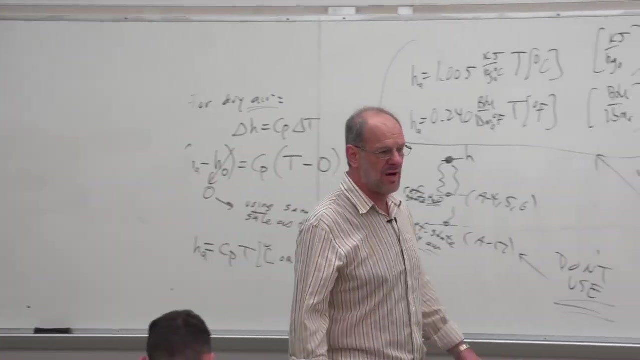 topic, which is the dew point. I mentioned dew earlier. We know what dew is. We've all experienced it before and we've experienced it perhaps in more ways than one. Certainly we know that when we walk outside, tomorrow morning will be. 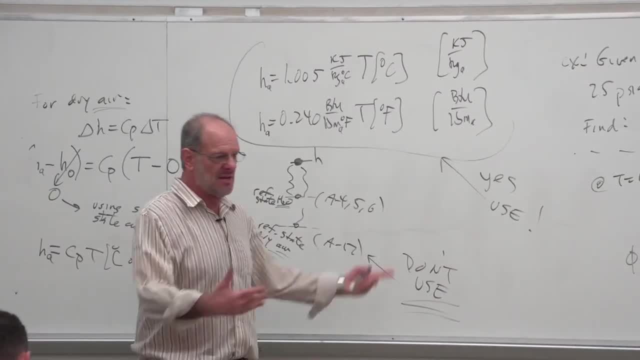 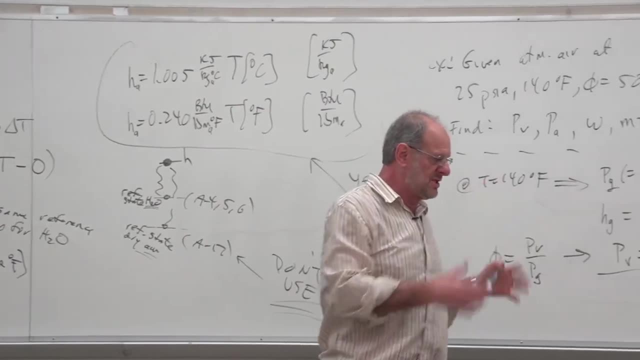 a good example. right, We have this nice deep marine layer. We have this nice deep marine layer and it comes on shore in the evening and it's cooler over the shore than it is over the ocean, So the air, which is saturated at a higher. temperature as it moves in off the coast is now going to hit a lower temperature. At lower temperatures the atmospheric air can't hold as much water. right At lower temperatures the partial pressure is lower. So we know that as this nice moist air blows in off the coast and hits us here in LA or 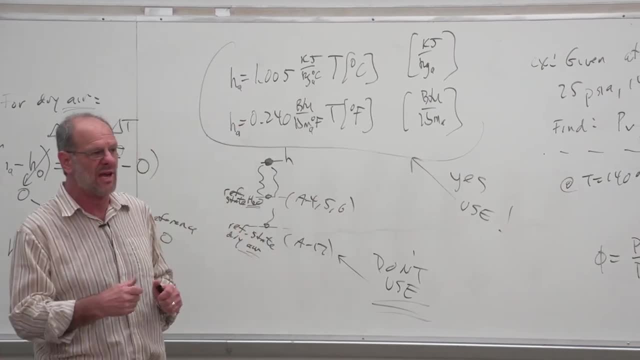 even inland, probably tomorrow. we're far enough inland, we'll still get some of that dew right? You wake up in the morning and everything's going to be covered with a layer of moisture. Well, where did that moisture come from? 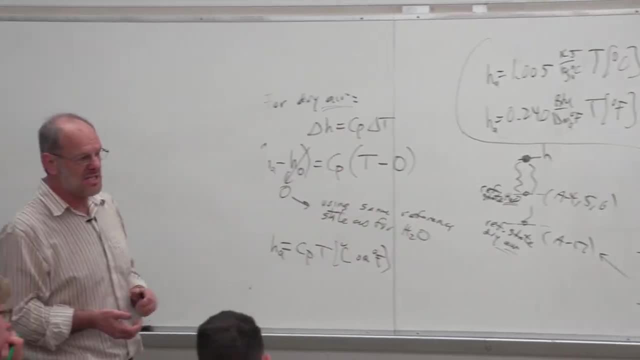 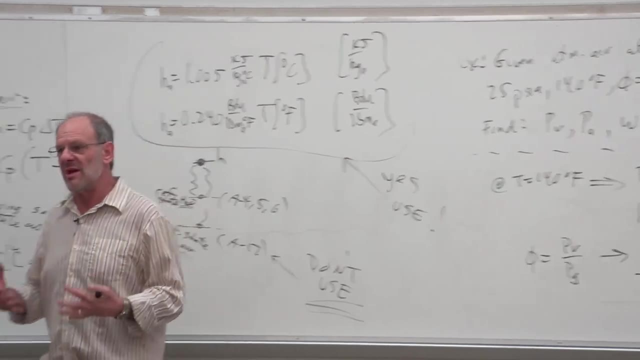 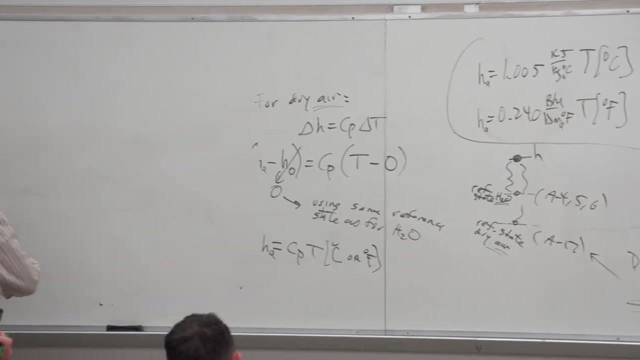 Clearly it comes from the atmosphere, right, And the only reason it exists as liquid water- that is, is dew on the ground- is because the temperature got too cold to hold that maximum amount of water vapor at the higher temperature that that air existed in as it was blowing on shore. So this is what we have to. consider when we consider the dew point. Okay, The dew point is the amount of water vapor that's going to condense out of the air. The dew point represents the temperature below which water vapor is going to condense out of the air. Okay, And in fact this is essentially opposite of what we were just talking. 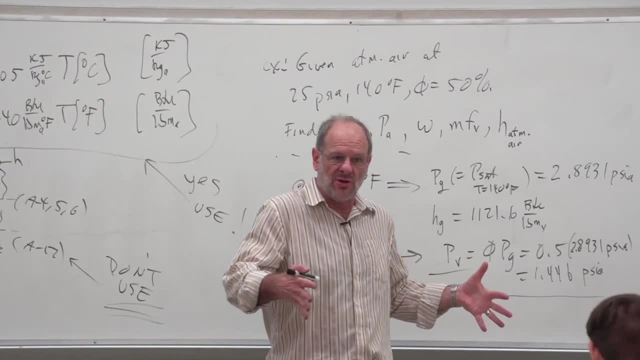 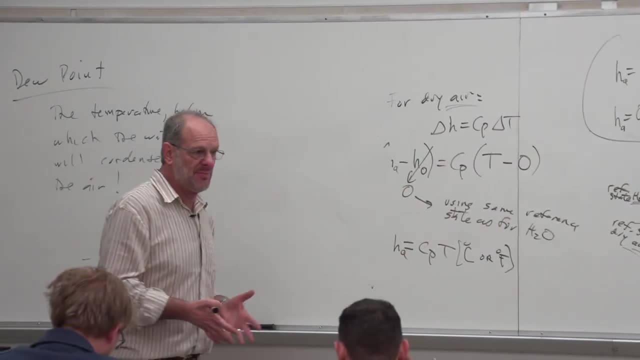 about earlier today. Earlier, I had said that as you raise the temperature, you can get more water vapor into the air because there's partial pressure that's going on. As you drop the temperature, you're able to hold less water vapor in the air because the partial pressure is going down. It's really just that simple. 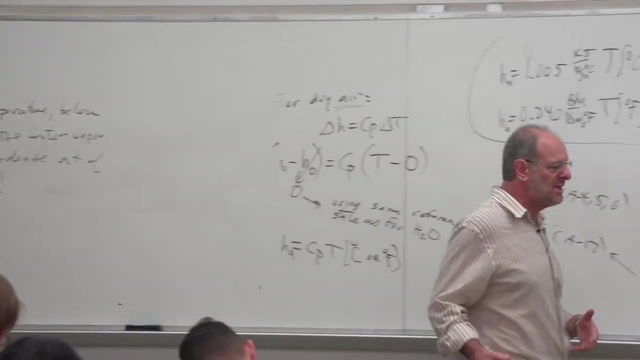 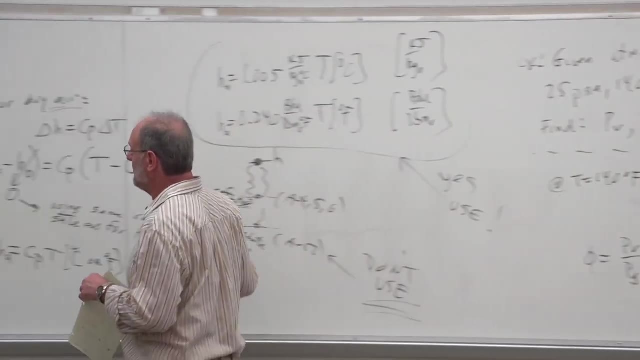 So there's always going to be some temperature, called the dew point, below which water vapor is going to begin to condense out. And again, this is what happens in our environment This time of year, in the springtime in Southern California, And of course it 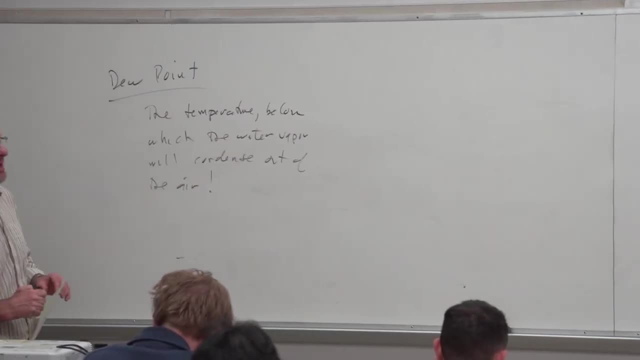 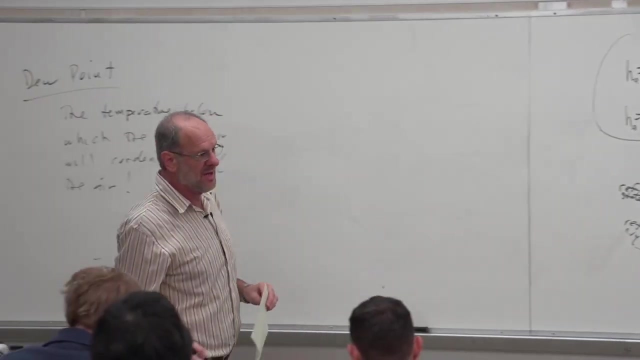 happens everywhere in the world. Fog, by the way, is liquid water, Right, It's liquid water that's just as suspended in the air. Fog is not water vapor. Fog is a form of dew. It was not always fog, Right, It was just water vapor. It's a. 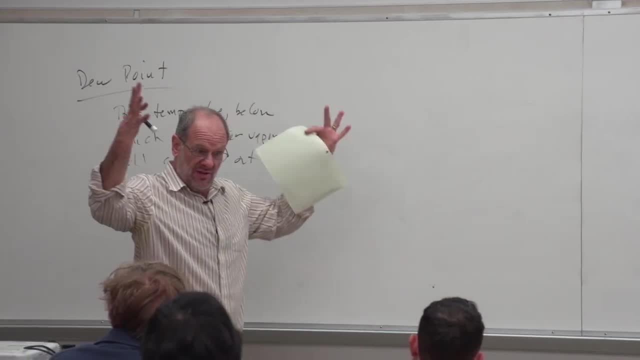 vapor. You can't even see it, You don't even know it's there. But if the temperature drops low enough, the water vapor condenses into a liquid And you see it, right, You see it as fog or as it collects on the ground. it's dew. So 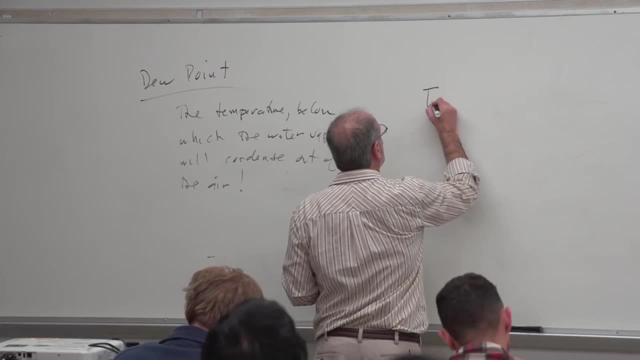 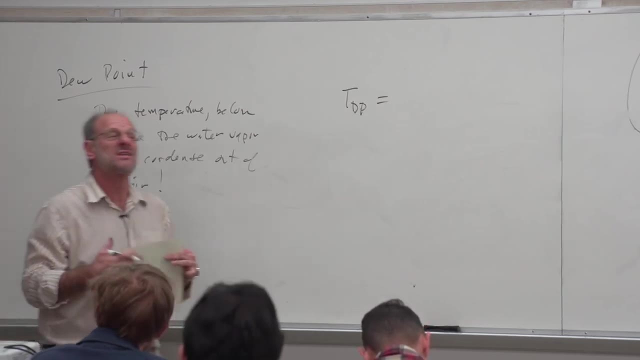 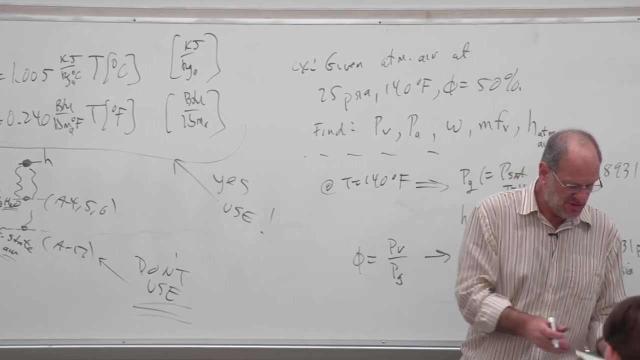 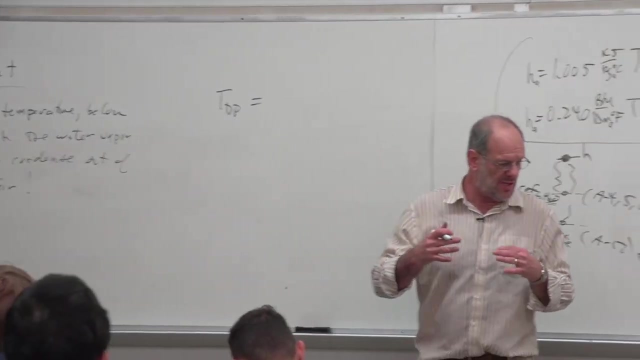 what is the dew point, then? Well, at what temperature represents, I'm sorry, what temperature represents the maximum amount of water vapor that can be held in the air. You know, this temperature is the saturation temperature at the partial pressure. If the temperature drops below the saturation temperature at, 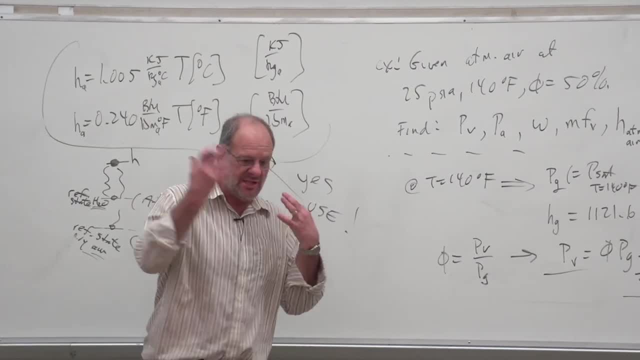 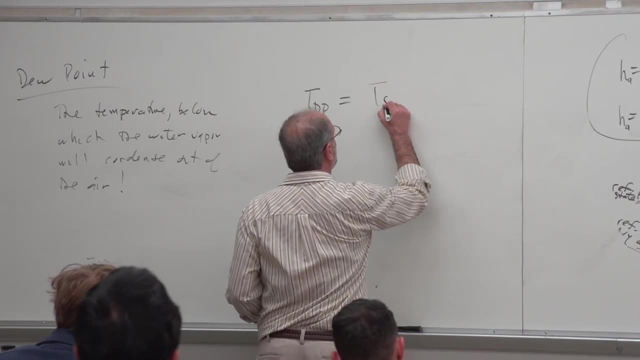 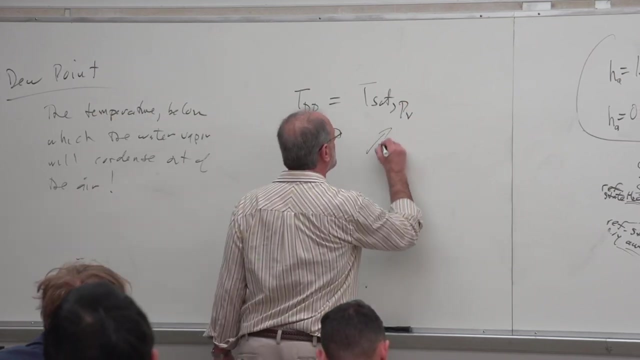 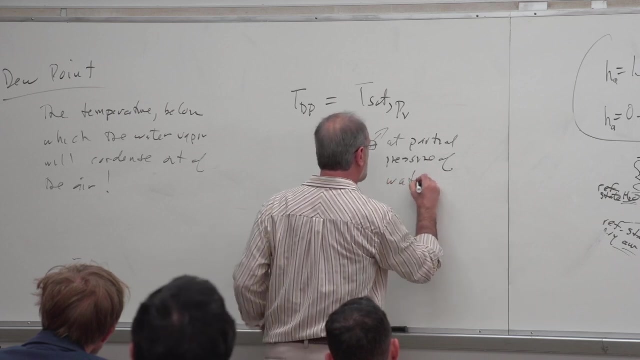 the partial pressure. condensation will occur. If the temperature rises above the saturation temperature corresponding partial pressure. then you can hold more water. So the dew point is really nothing more than the saturation temperature at the partial pressure of the water vapor. Okay, So this is how we define the 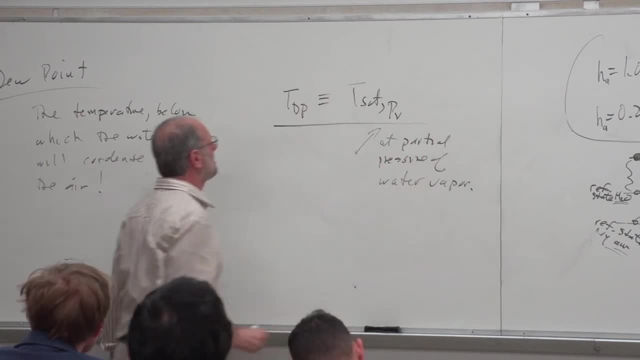 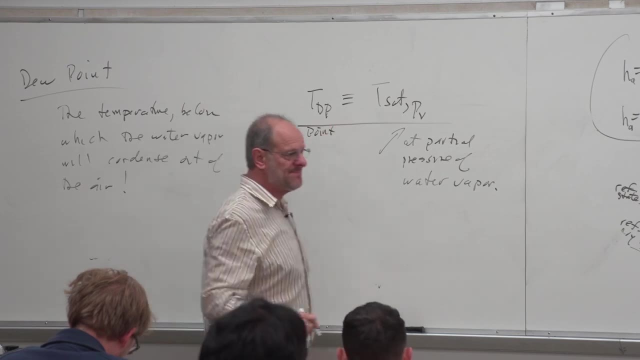 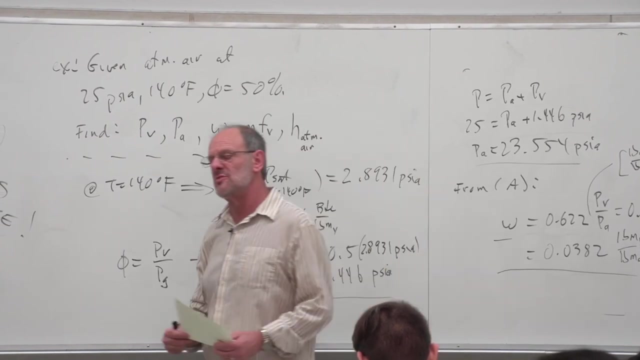 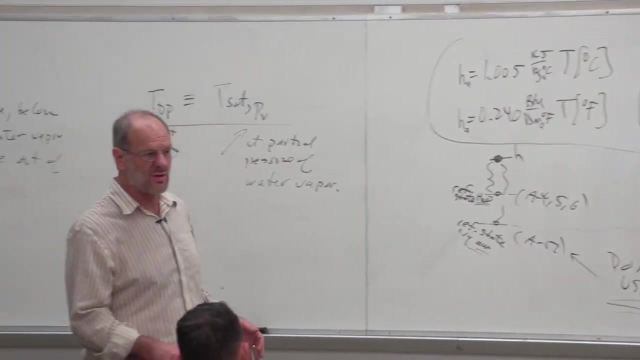 dew point. I'll put three lines in my equal sign. And this is an important equation. So this is the dew point. Okay, So if we have atmospheric air, when the falling temperature reaches the water saturation temperature, condensation begins to occur. We simply call that the dew point. So let me go through a real 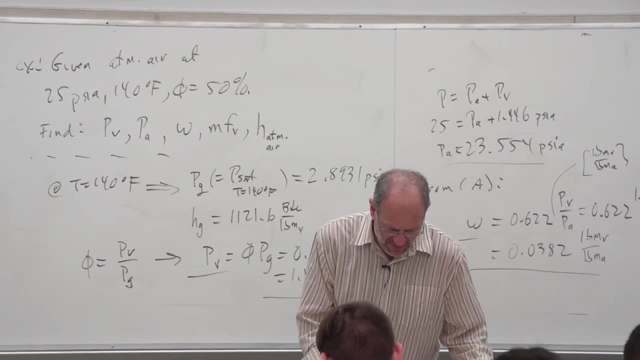 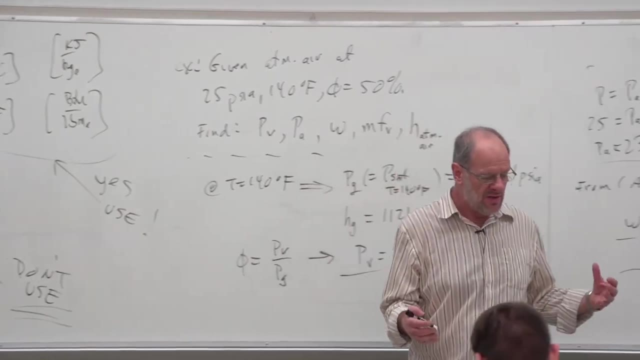 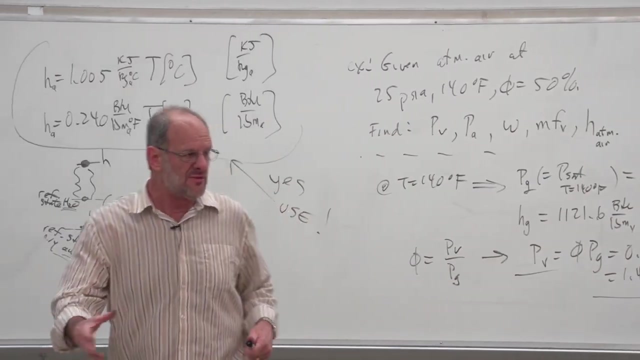 simple little example problem of this And, by the way, this kind of example problem is pretty typical. Yes, we could have dew forming in the atmosphere, but I mentioned earlier that you probably have other experiences of hitting this dew point. What if you take a cold can of soda pop out of the refrigerator and you 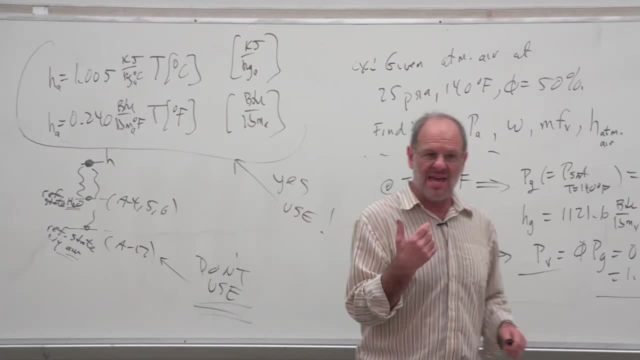 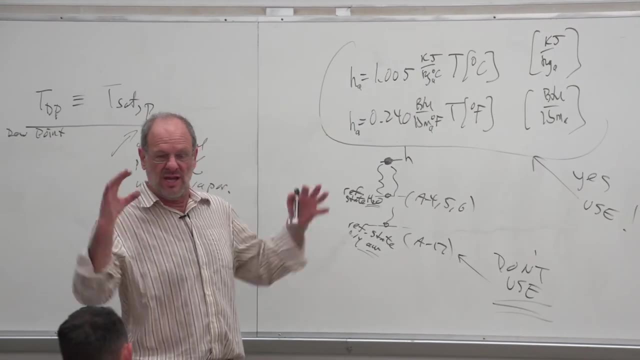 bring it outside. on a nice, warm, humid day, The outside of the can gets wet, doesn't it? Did water leak through the can out of your soda pop? No, of course not. It's dew, right, It's colder than the dew point. So any water vapor in the air. 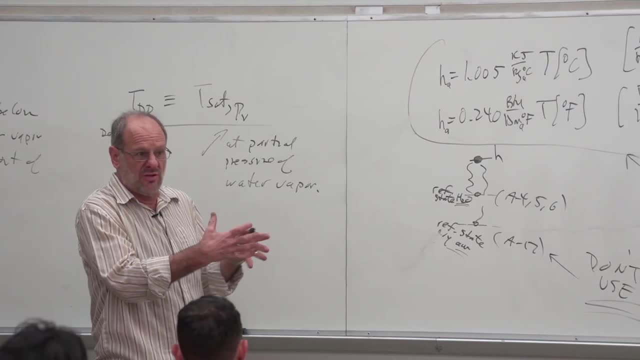 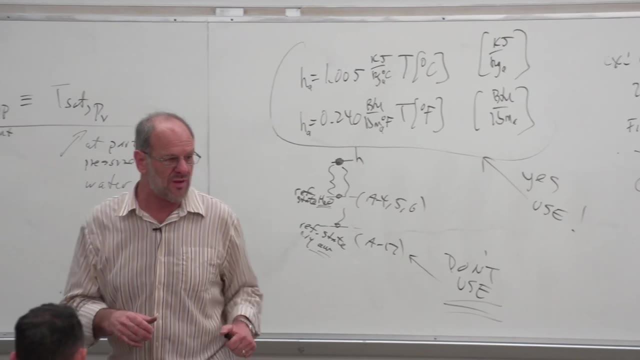 that immediately touches that can well. it drops below the dew point. You're going to get condensation occurring. What about windows? Anybody who's been, let's say, in Hawaii or any other humid place? you got your air conditioner on it's 90. 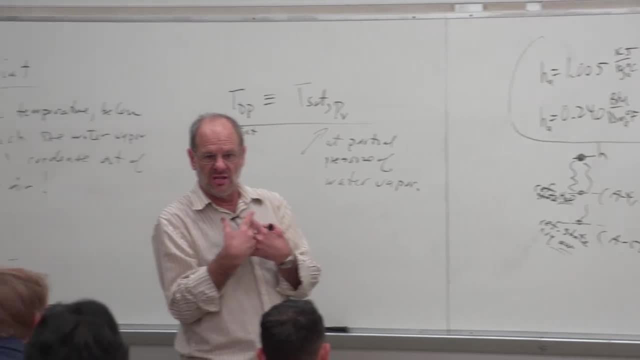 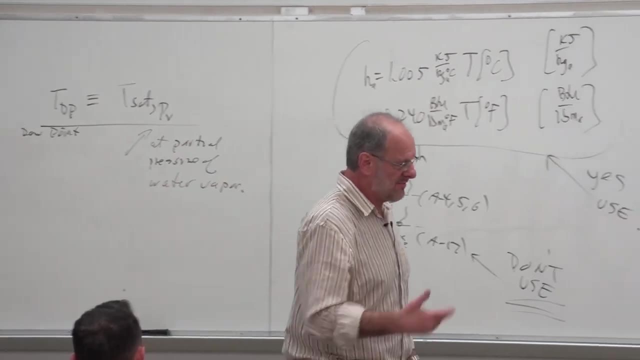 degrees outside with high humidity, You turn your air conditioner on on the inside of the car, those windows get cold and then you have dew forming on the outside of the windows. A lot of people from this part of the world never consider that that fogging up on their windshield is actually on the outside, not on the 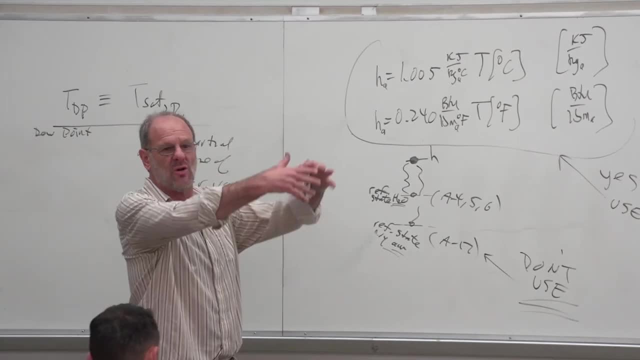 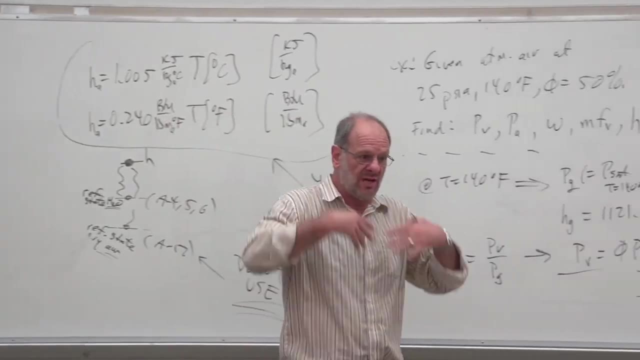 inside right Here in Southern California, it would likely be on the inside. We'd have a cold evening. We'd have people inside our car. Because of the people in the car, the car is warm. There's more moisture right because we're all. 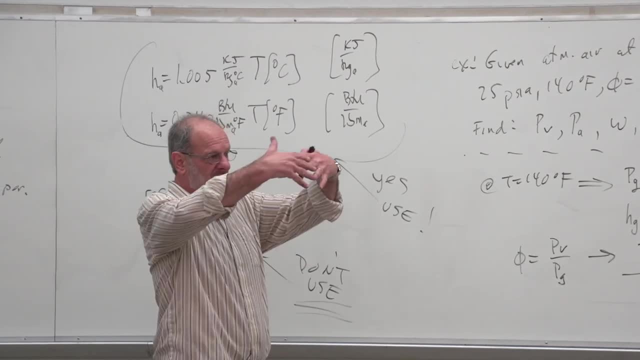 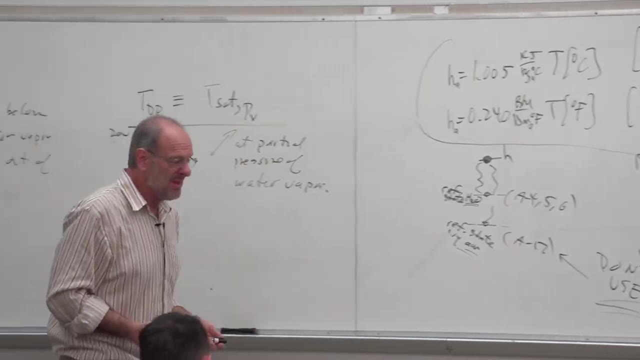 breathing out and moisture water vapor is getting into the air. And now this warm, moist air hits the cold window and then your water vapor is going to condense on the inside of that window, right? So if you're in a humid area and you can't see through the windshield, just 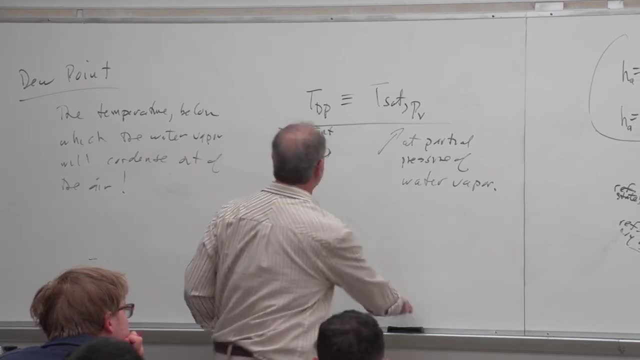 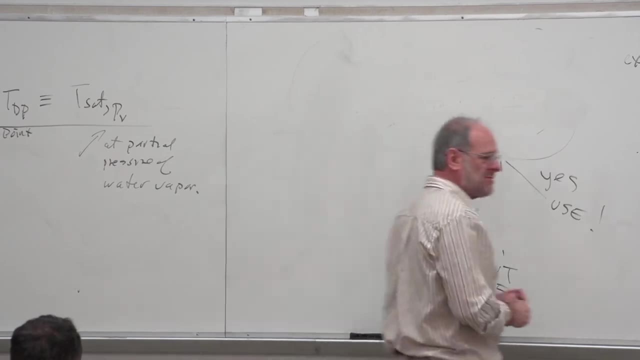 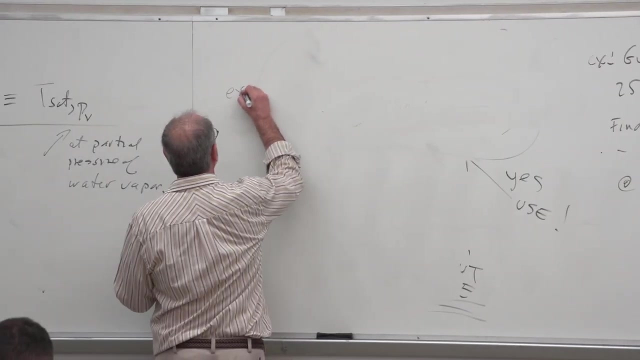 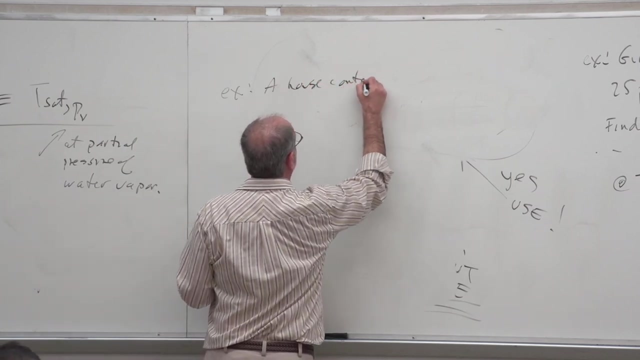 turn your windshield wipers on. Otherwise, turn your defroster on right. So that's the nature of the dew point. So here's your example. Let's say that we have a house and the house contains air, water vapor and water vapor. So 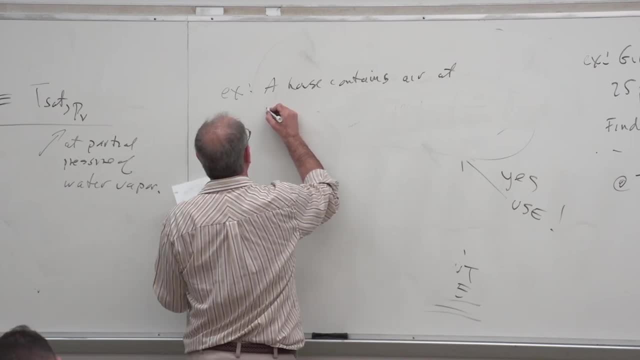 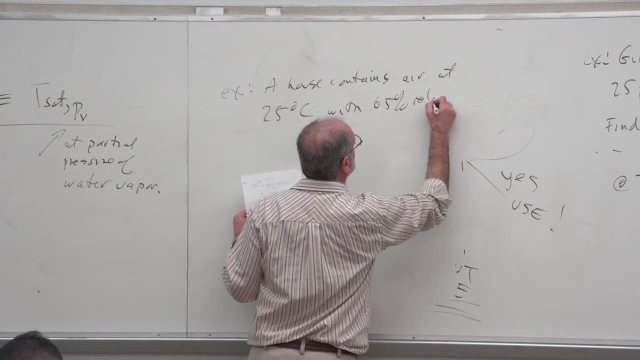 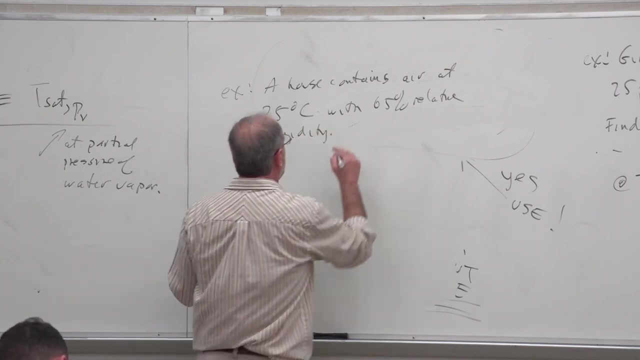 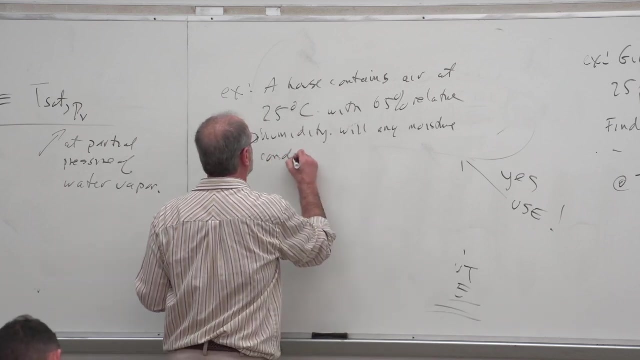 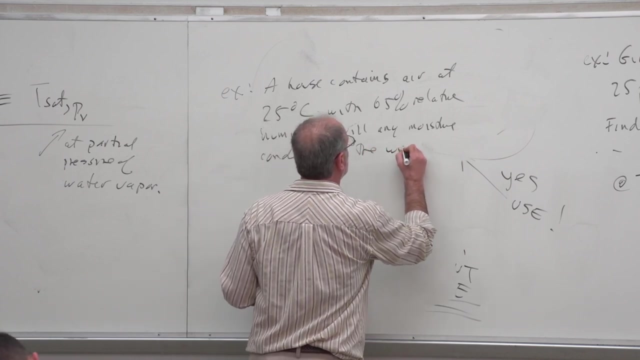 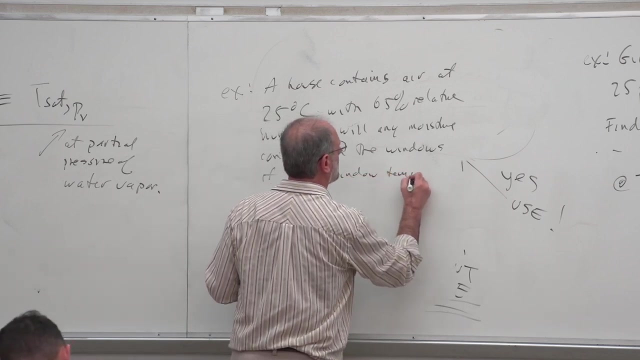 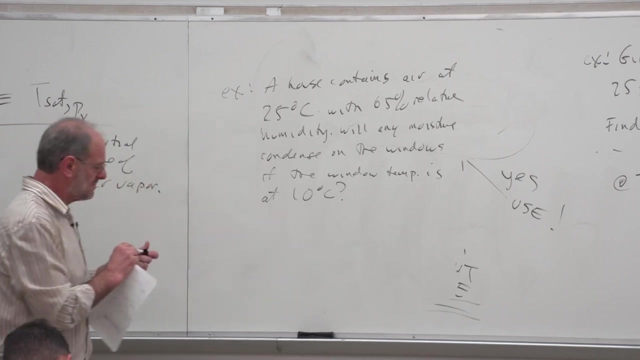 we're at a particular temperature. So let's say it's at 25 degrees Celsius with a 65% relative humidity. OK, And here we'll ask: will any moisture condense On the windows if the window temperature is at 10 degrees Celsius? OK, So in. 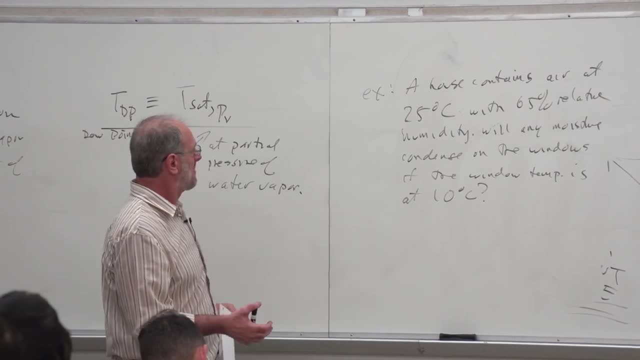 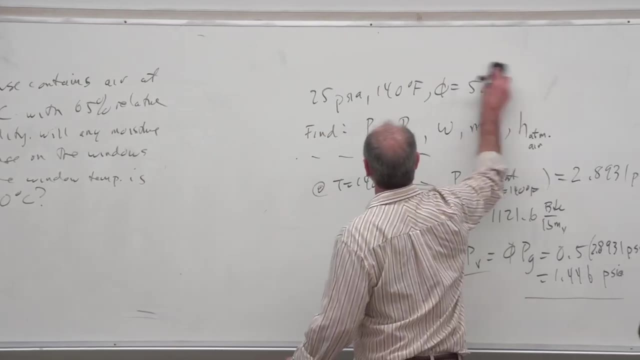 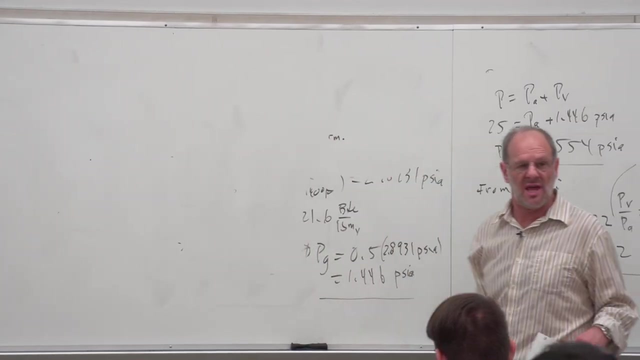 other words, we have a cold day outside. On the inside, we're keeping it nice and warm: 25 degrees C. There's a decent amount of humidity in the air- Relative humidity is 35%- But now we're on a cold day. right, The windows are cold You. 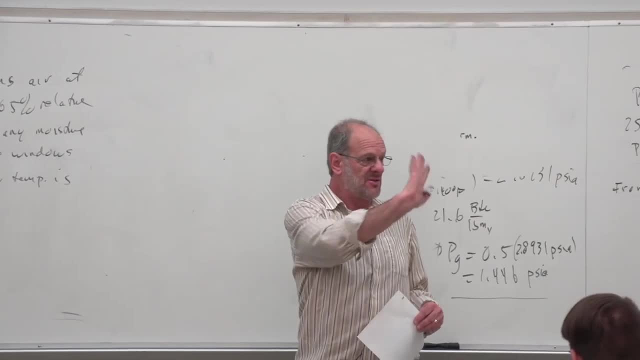 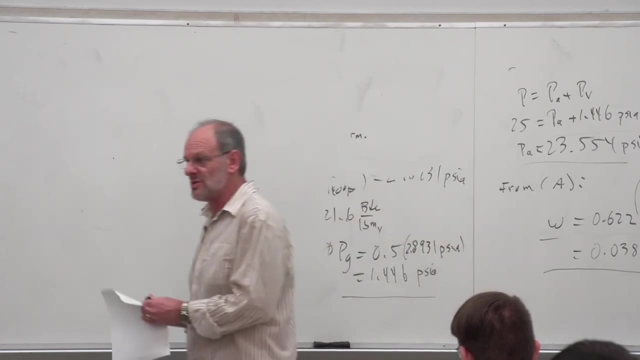 touch the windows on a cold day and they're cold. In fact, sometimes there's moisture that's condensed on the inside of your windows. on a nice cold day, when you've got the heater going on in your house, right Well, the windows have. 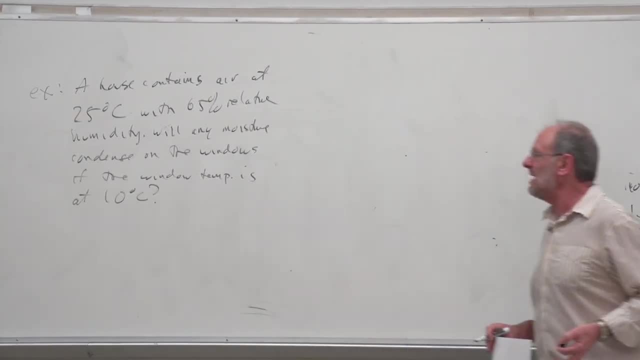 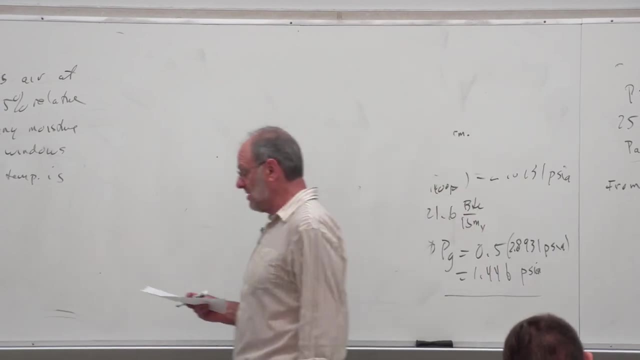 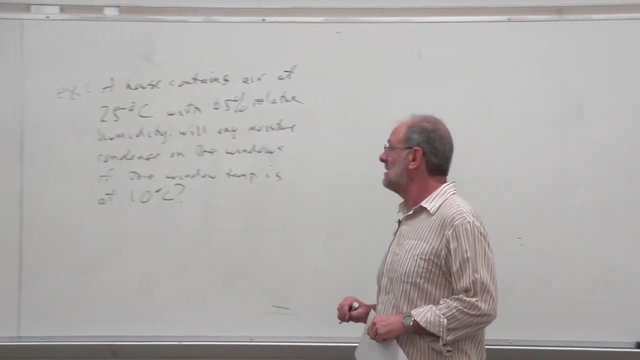 allowed the air to hit the dew point. So the question is: will any water vapor condense on, really, the inside of these windows? And how do we figure that out? Well, all we have to do is find the saturation pressure at the partial. 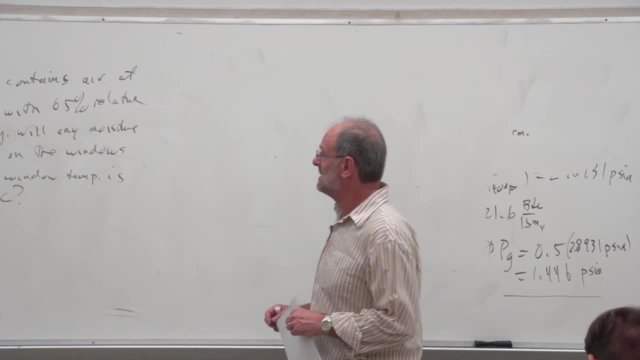 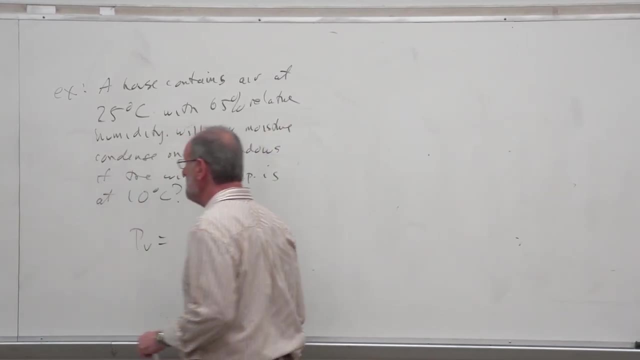 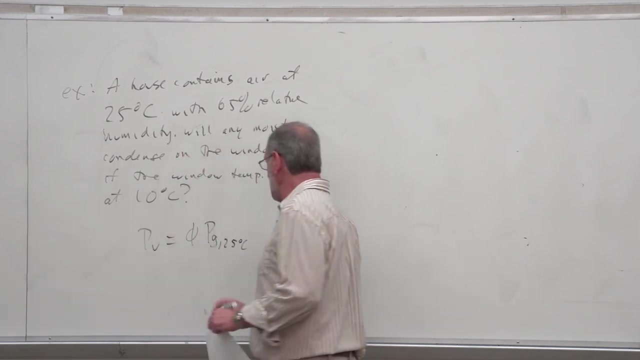 pressure of the water vapor, And that is going to be a function of the temperature. So, first, what is PV? Well, from one of the equations presented earlier, this is just a relative humidity times PG at the given temperature, which is 25 degrees Celsius. So what is PV? Well, this is just a relative humidity. 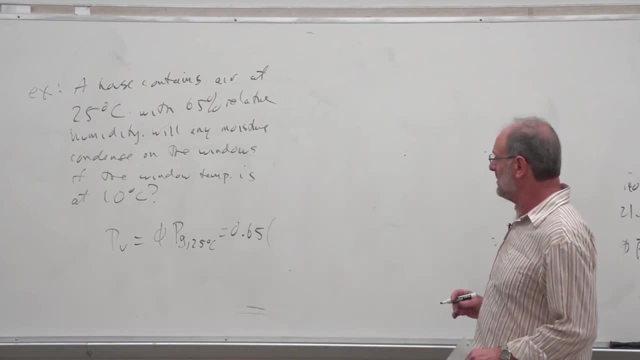 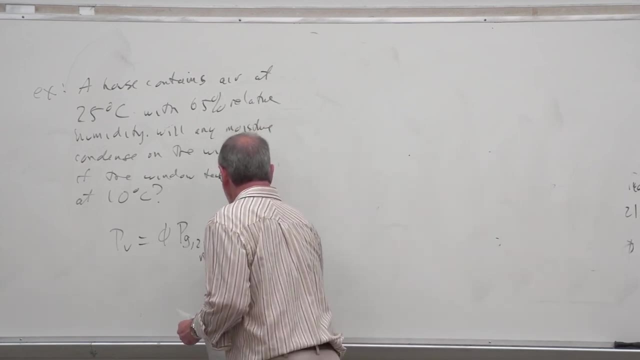 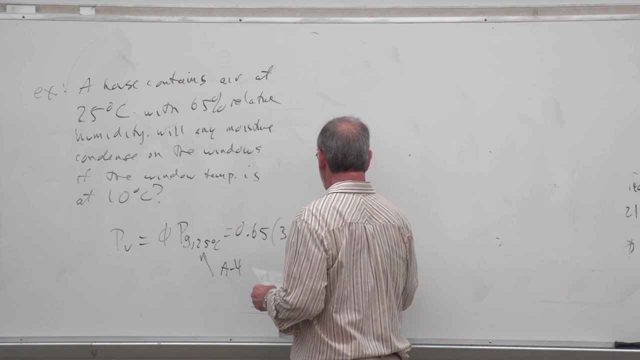 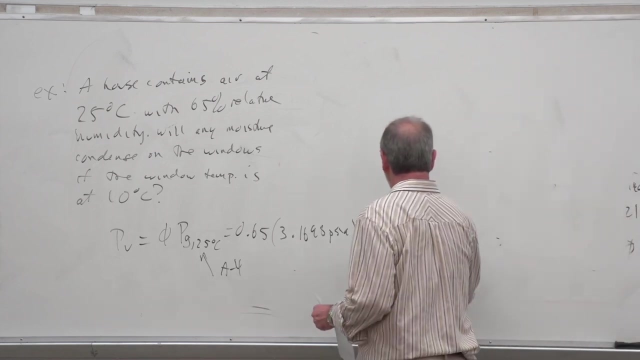 is 0.65.. The saturation pressure at the given 25 degrees Celsius- and this is just going to come from table A4, is going to be 3.1698 PSIA. So therefore the partial pressure of the water vapor is 2.06.. So now we find the saturation. 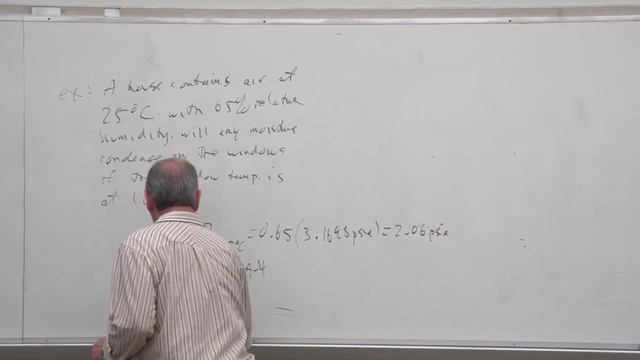 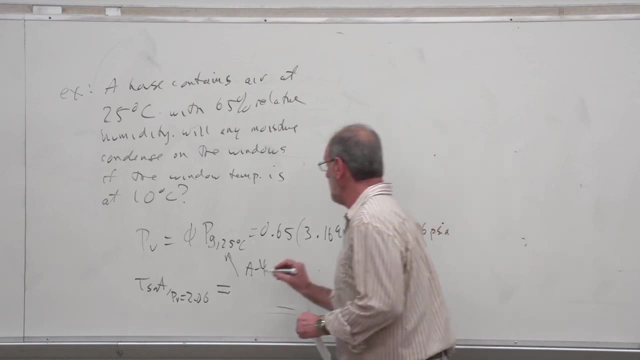 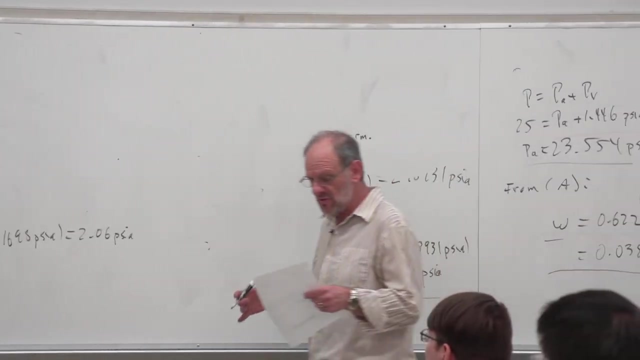 temperature At PV equals 2.06.. So here we now have to use the other table right, Table A5. We go into our pressure table And of course we are going to have to do some interpolation, But what we do find is that this is equal to 18.0 degrees. 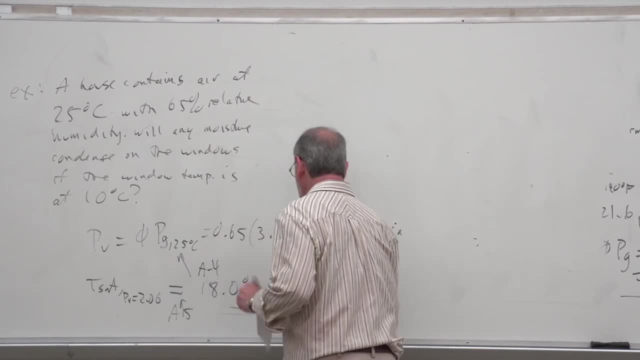 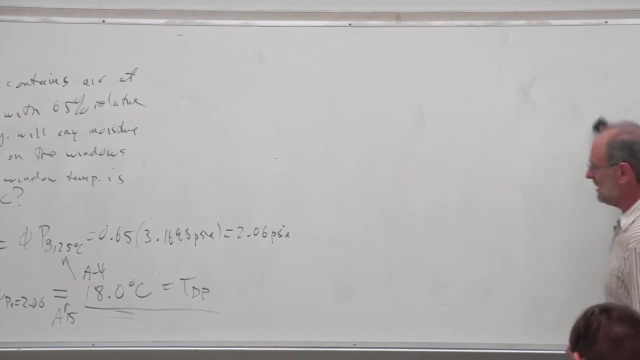 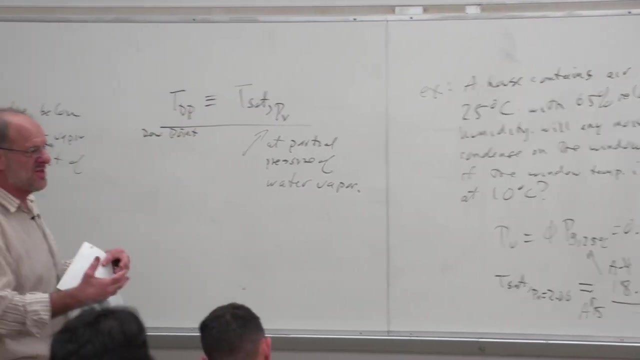 Celsius. So that's the dew point, And now it's just a matter of interpreting our results. I have had plenty of students that have calculated the dew point temperature and then not even know what to do with it- whether that tells you that the water is. 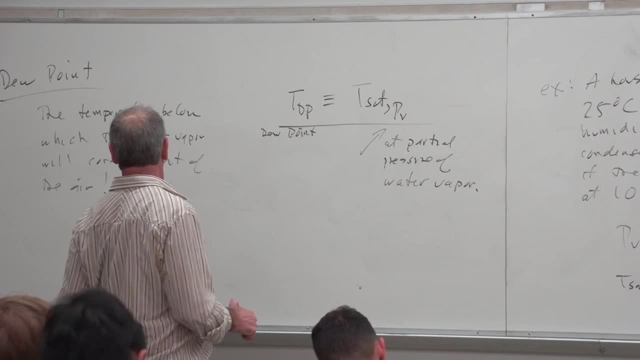 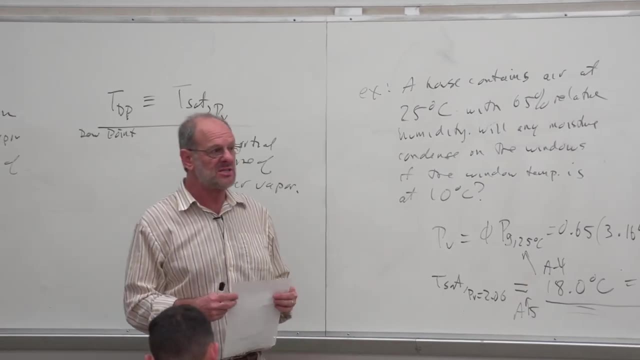 going to condense out of the air or not, But the rule is pretty clear: The temperature below which the water vapor will condense. Any temperature below 18 degrees Celsius will cause the water vapor to condense. So is 10 degrees. 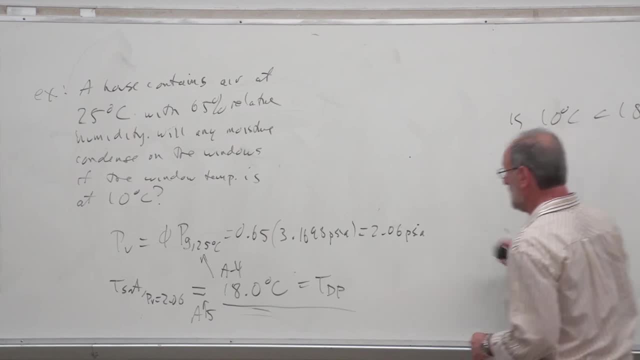 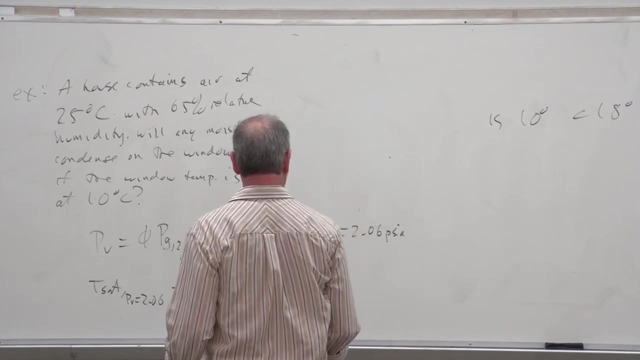 Celsius less than- I'm sorry, 10 degrees. this should say Fahrenheit. Again, my apologies. And this should oh uh-oh. OK. Now I'm confused and I got to look at my notes again. Yeah, I just have. it is supposed to be Celsius, This is. 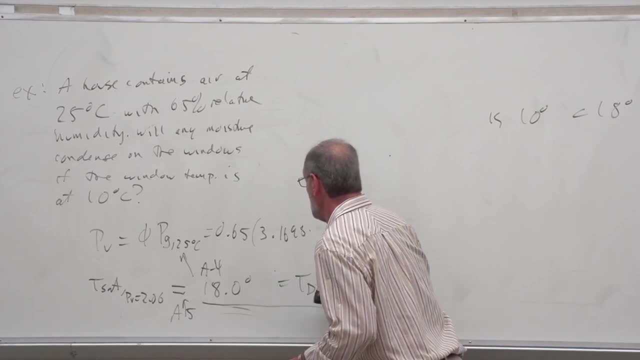 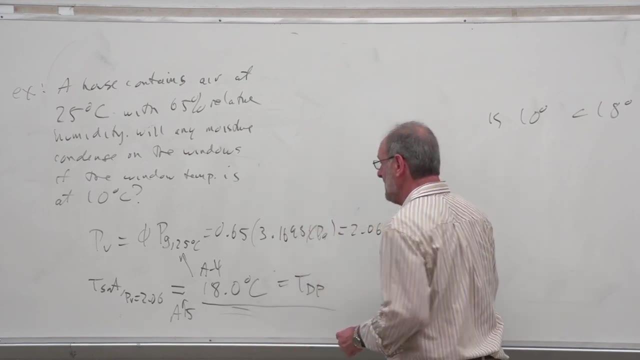 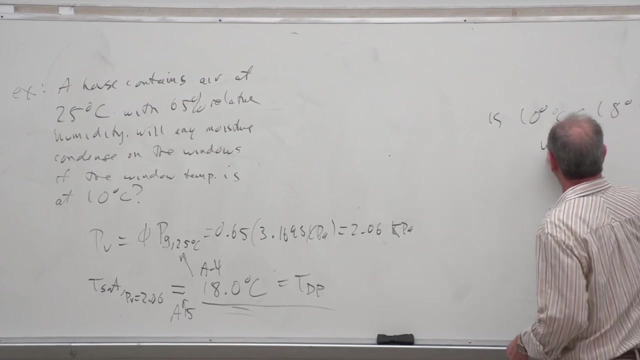 kilopascals, not psia. So yeah, that was right. 18 degrees Celsius. This is in kilopascals. Sorry about that. Nonetheless, is 10 degrees Celsius less than 18 degrees Celsius? The answer is yes. 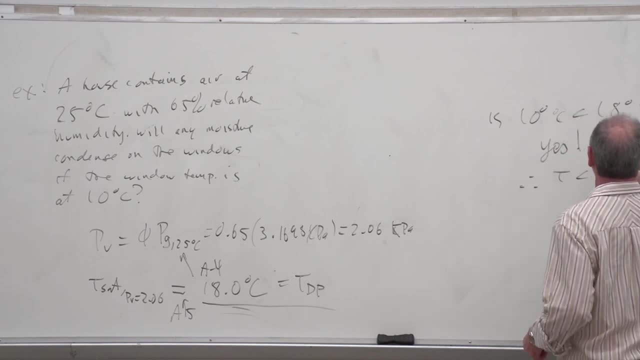 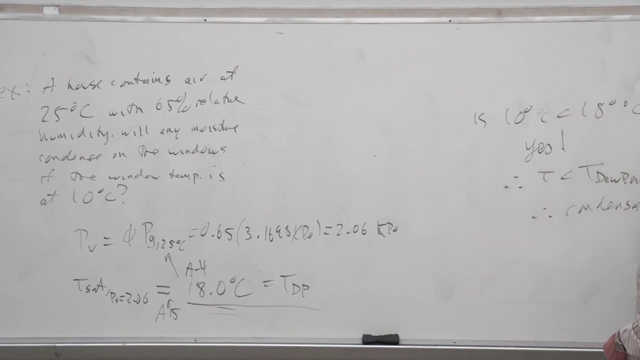 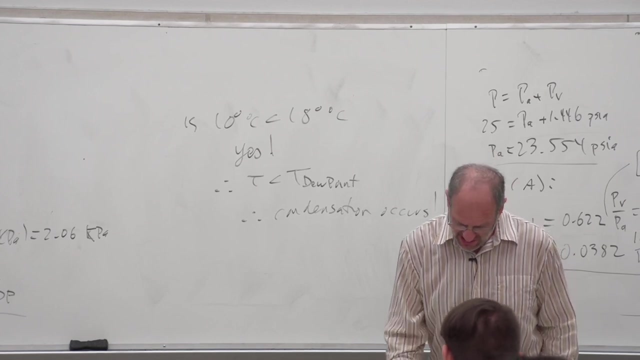 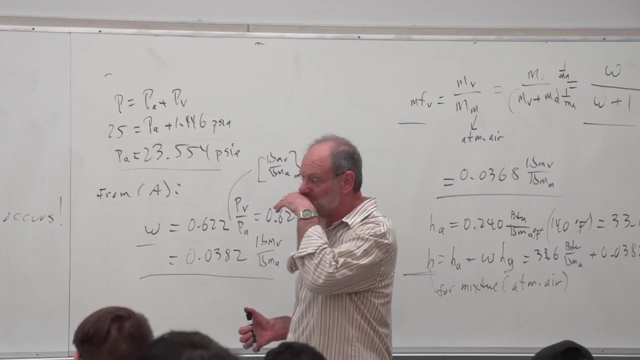 The answer is yes, And therefore the temperature is below the dew point And therefore condensation. So this is one way that we're going to utilize this information. So are there any questions on this particular problem? So now, 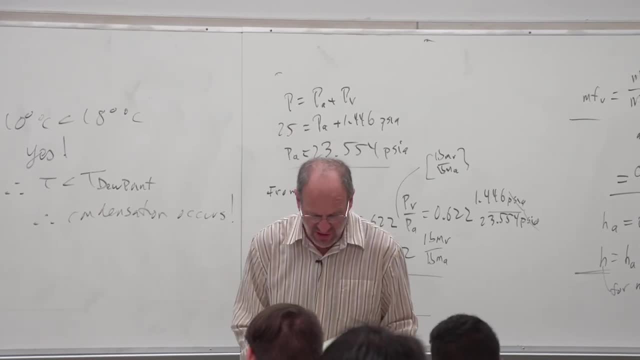 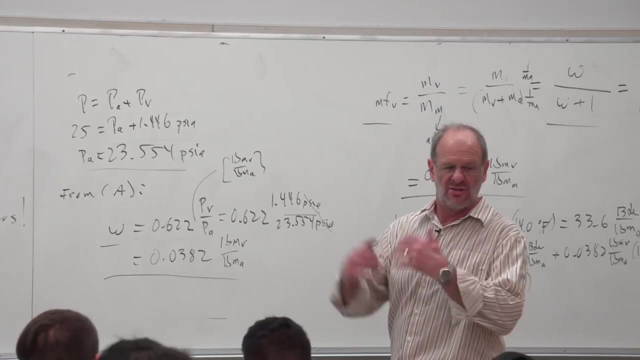 we're beginning to look at some realistic problems associated with dew point. By the way, this is just an academic exercise and it's not just an exercise in trying to figure out if your glasses are going to fog up when you go into a hot. 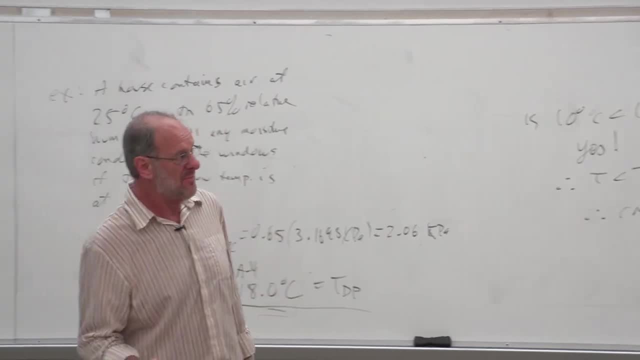 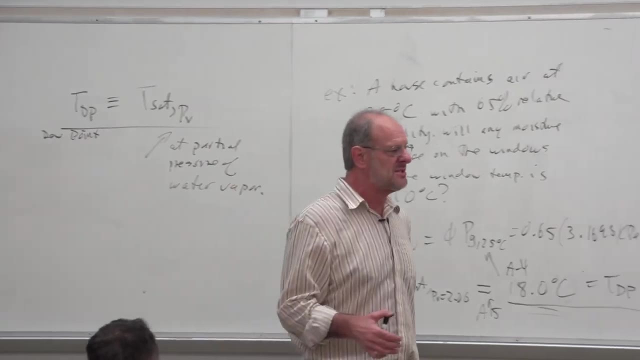 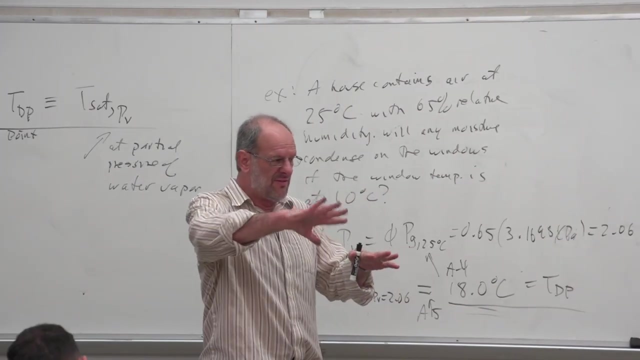 humid environment after coming out of your air conditioning or whatever. There could be real safety issues associated with this. There have been instances, particularly in the south of the United States, where you have hilly areas where it gets really cold at night but it's very humid during the day. You find that. 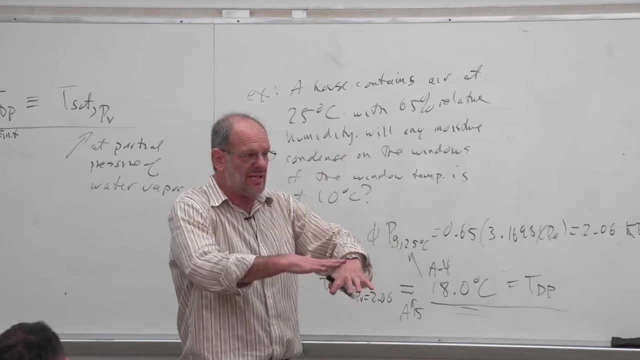 fog, which is really just dew, is really not a problem. It's just a little bit of a little bit of a problem, But it's a little bit of a problem, And that's what the weather forecast does. The weather forecast does. The weather forecast does. 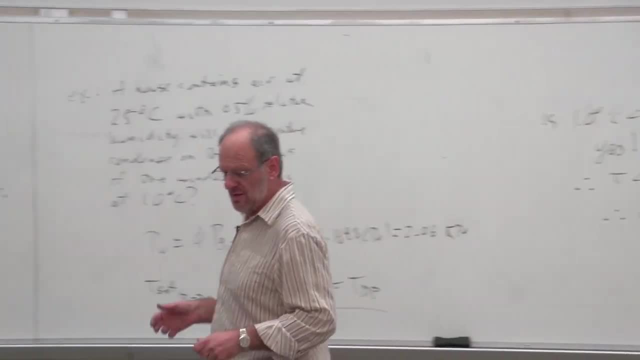 do tends to collect in the bottom of these different hollows, if you will, these different valleys. That's cool, you know, if you're living in that area, it's kind of nice to have the cooling effect of all that moisture. On the other hand, 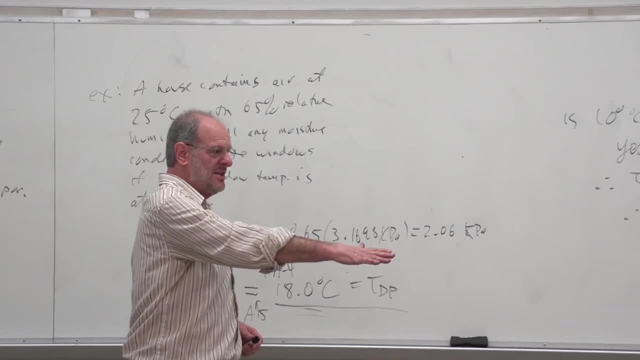 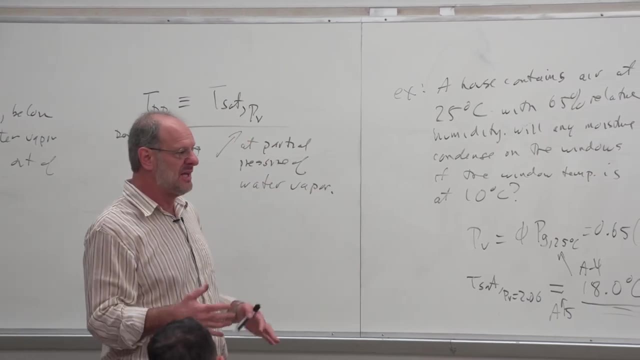 if you're a truck driver and you're just driving long haul and all of a sudden you come down into a valley and visibility goes from perfect to zero, just like that. that's a safety issue. There's some areas where they actually do what they. 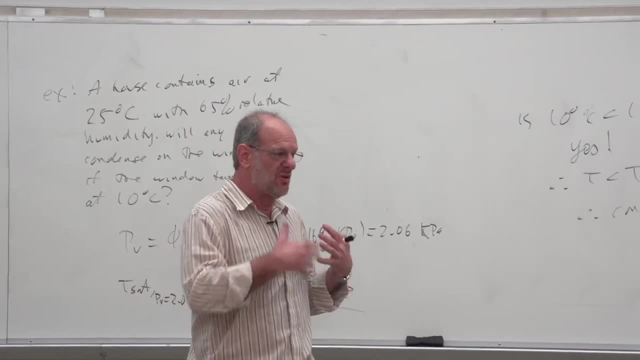 can, to try to heat up the local area, the local air, so that you don't get a lot of dew, You don't have this dew forming, so you don't have massive pileups and truck accidents and all that. So, yes, this could be important. This is also. 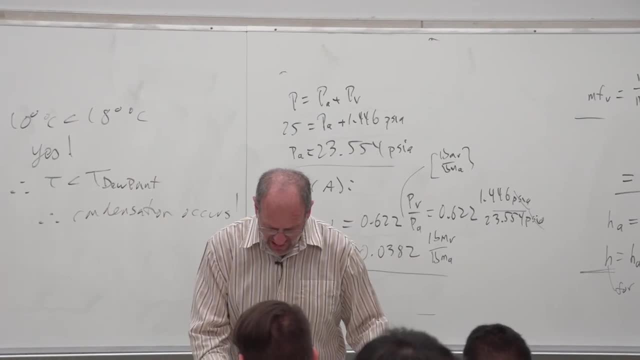 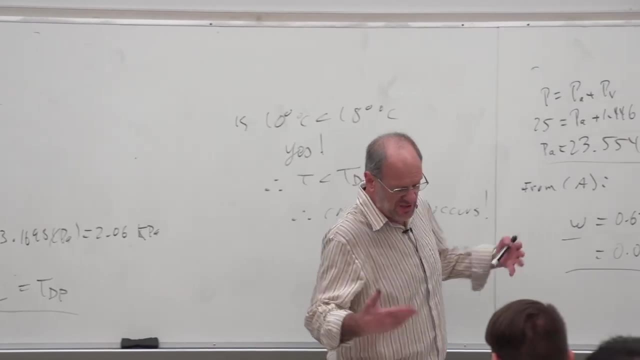 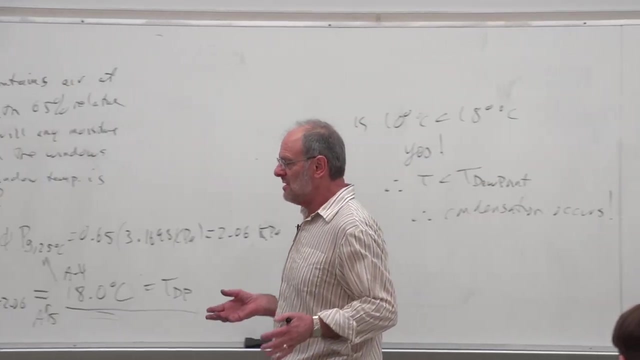 important from another point of view. Often we would like to know what the moisture content is of atmospheric air. And you know, not because we're interested in the dew point, just because we're interested in the comfort level of that particular air. How can we determine the moisture content in some sort 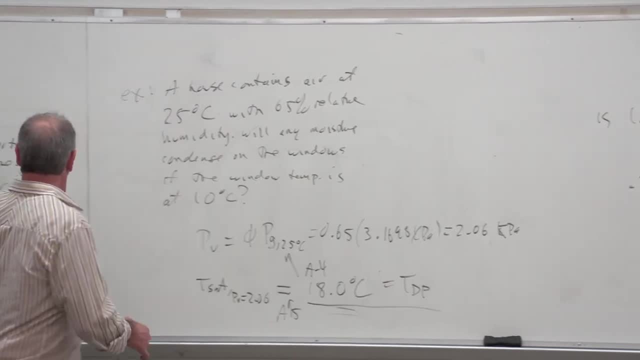 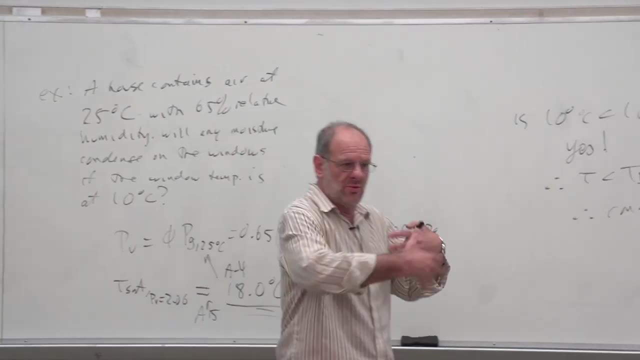 of atmospheric air. Well, you know, if you're a truck driver and you have a lot of dew, well you can utilize the dew point. What if you were to just take a sample of that atmospheric air and then run it through some sort of a cooling? 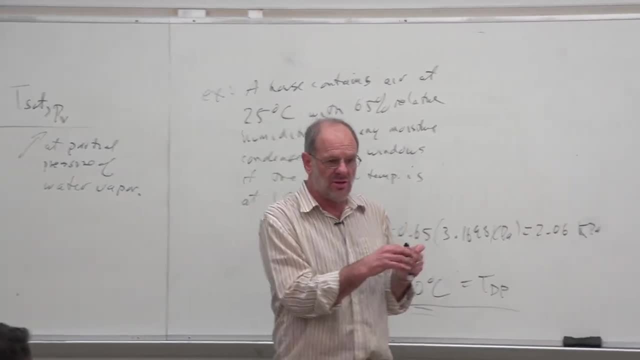 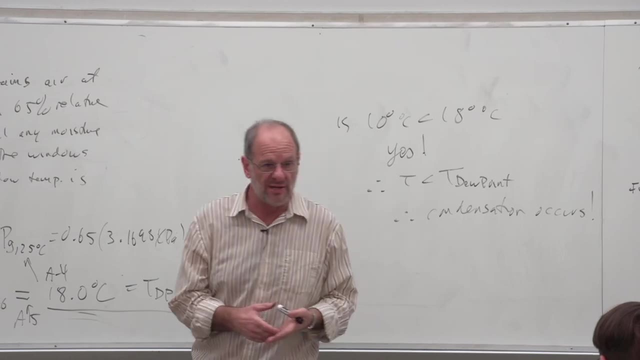 device, some sort of a heat exchanger, and then just continually monitor the temperature. When you notice that the water vapor is beginning to condense, read off the temperature. That's your dew point And you can actually work backwards from the dew point, similar to what we've done in this example problem. You can. 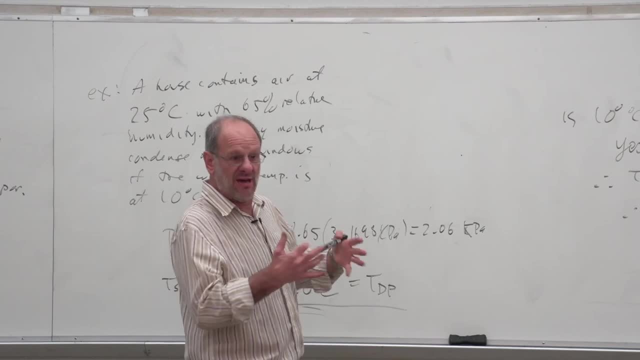 work backwards through the dew point and actually find the dew point. And you can actually work backwards from the dew point, similar to what we've done in this example problem, And you can actually find the amount of water vapor in that air. So that might be of some interest to you for some particular process or for. 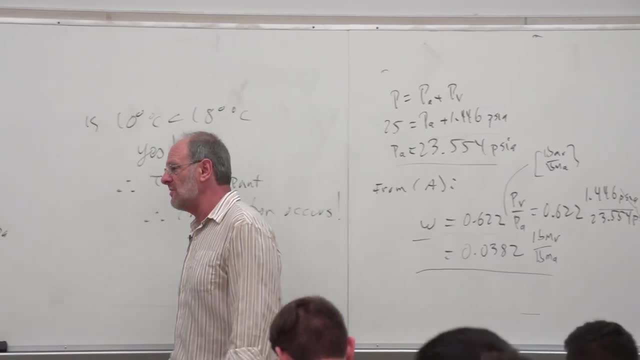 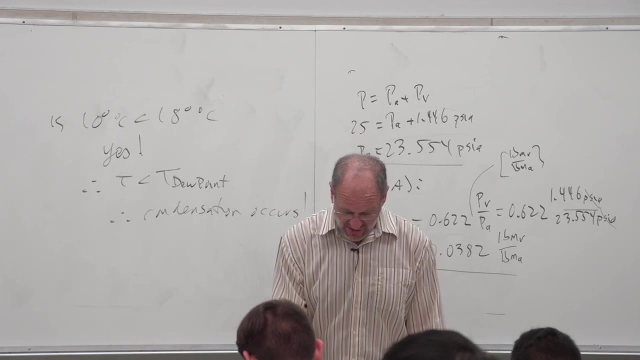 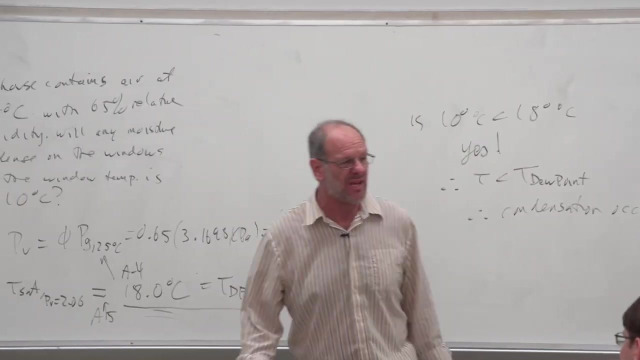 whatever reason you want. So certainly we could use the dew point for more than just, you know, an interesting academic exercise. There's safety issues, There's issues associated with comfort. You know that's part of being an engineer. What are your applications for what you're learning, Anyway? so I'm not going to get 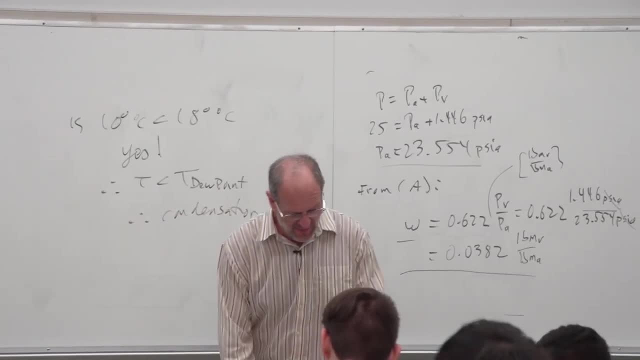 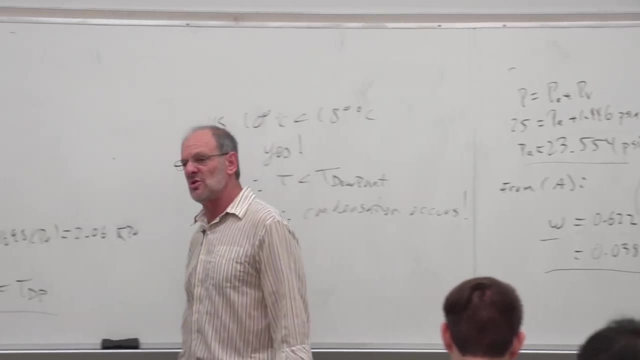 into any more today. I'm going to go back to the previous slide. I'm going to go today, So that's all. Next time we're going to continue with this discussion of air water vapor mixtures. I've got some other sample problems to do for you. We've 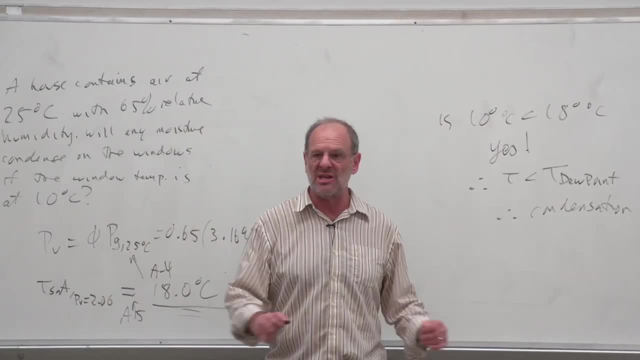 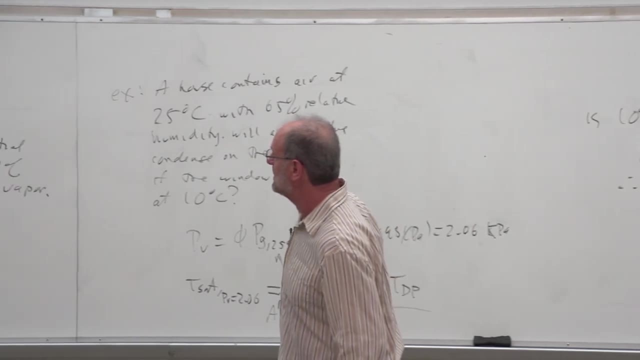 got some other processes to be considering, But that'll be next week, So have a nice weekend, everybody. Is there a question? Yes, Under the definition for dew point, Yes, What does it say? Condense out? Condense out of the air? Yeah, the temperature below which water vapor will. 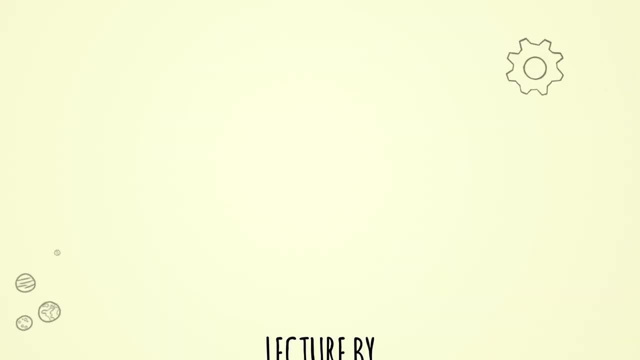 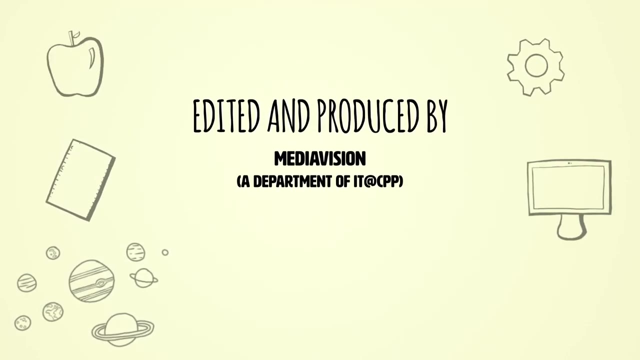 condense out of the air. All right, Thank you.